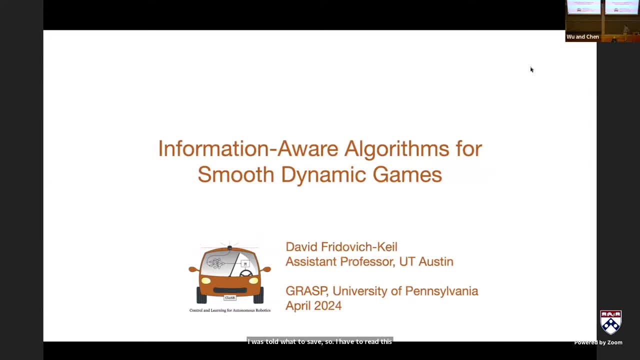 Previously recorded talks can be found in our YouTube channel and website. If you are listening, If you are joining us via Zoom, please submit your question using Q&A button at the bottom of your screen. These will be answered during the Q&A panel at the end of the talk. 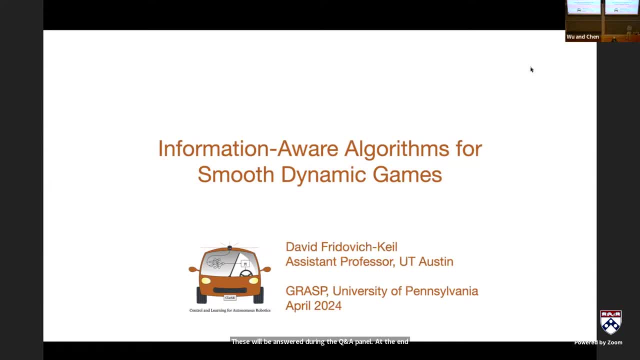 If you are here in person, you will have an opportunity at the end of talk to provide your questions to the panelists. to the panelists, And we have two students panelists. One is Bruce Lee and Igor Spaisov- Spaisov, I think I'm probably the only one who can pronounce it properly- being of Slavic origin. 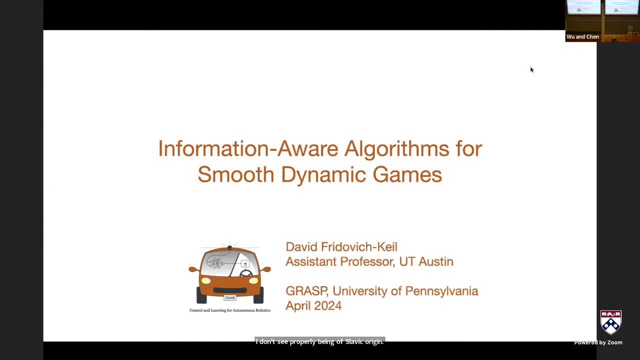 All right. so let me just tell you, David has been working with Claire Tomlin. Claire Tomlin was his thesis advisor and they were looking at how to model interaction And we have two robots using game theory, which there were several other people who have done similar work, right. 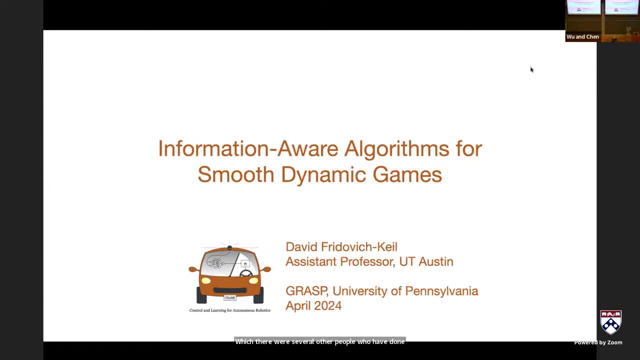 And yes, yeah, you probably will mention them, Lily, and with Shankar Shastri, and so, So, as for the future, please tune next Friday, April 19th and 1030, to our next Grass Lab on Robotics featuring Christy Morgan. 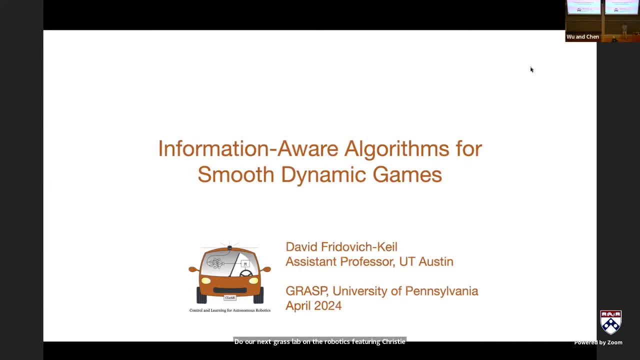 It's from the University of Washington. It's interesting because Lily is also from the University of Washington. She also did work on this game theory. For more information on upcoming events, be sure to follow us on social media or check out our website. 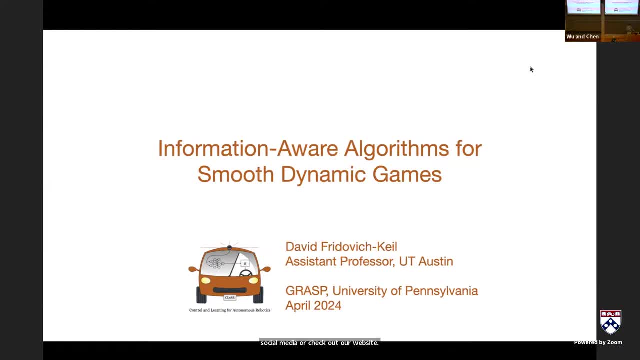 Don't spend too much time on social media. It's not good for you, It's really not good for you. Yeah, Thank you again and have a wonderful day. This is the instructions from the above. Anyway, David is a delightful guy who really has a deep ingrained curiosity, which I really appreciate. 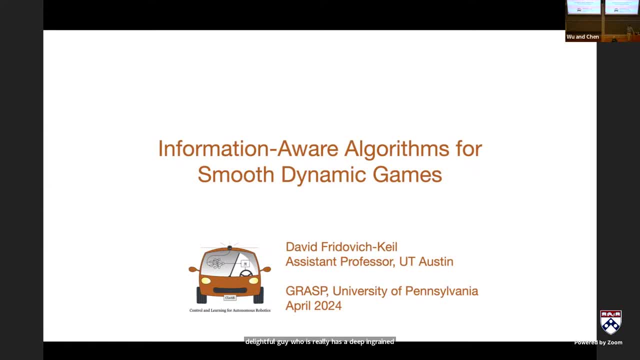 And sometimes you may have heard me complaining that some of the students don't have enough curiosity, And David and I shared a lot of interesting things about culture, about different people and history, in addition to all of the sciences. So enjoy his talk. 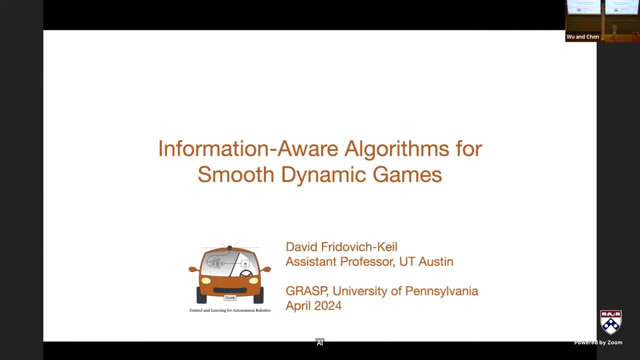 All right. Thanks so much, Ruzhna, for a really kind introduction And thanks to all of you. Thank you And thank all of you for having me. So I want to tell you – yeah, Yes, we did. 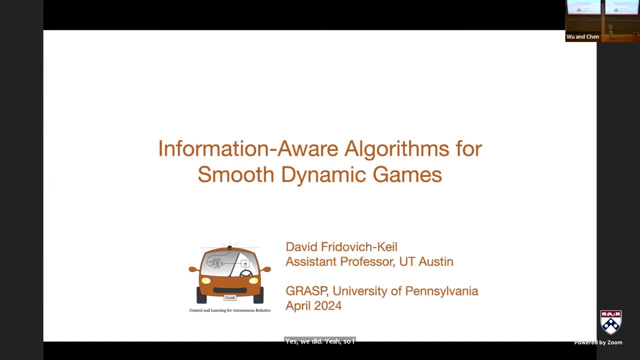 Um, yeah, I, I. so I was using this um TA, the lab TA, for the intro robotics course, And so I remember, you know, creating all these lab assignments and inserting bugs just to make the students you know. 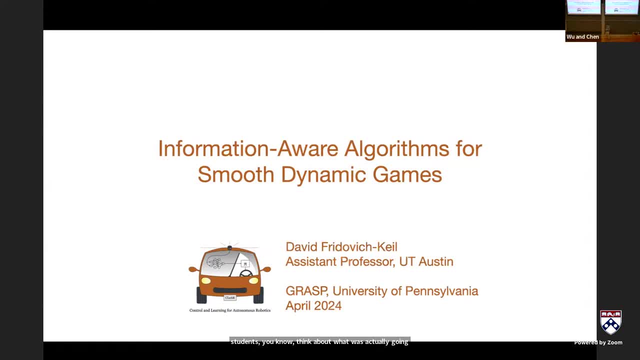 think about what was actually going on and figure out how to how to fix them. So, um, yeah, that was, that was. that was the first time I think we actually really interacted, and it's been, it's been great Okay. 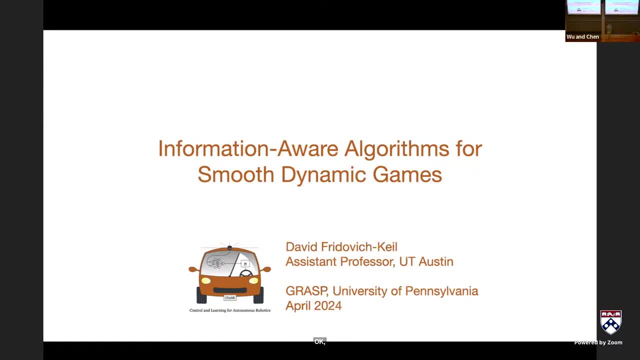 Okay, So, um, what I want to tell you about today is a topic that I think has really captured my imagination since I first entered, uh, I guess, um first encountered it back in maybe 2018 or so, Um, and at that time, what was happening was I, um. 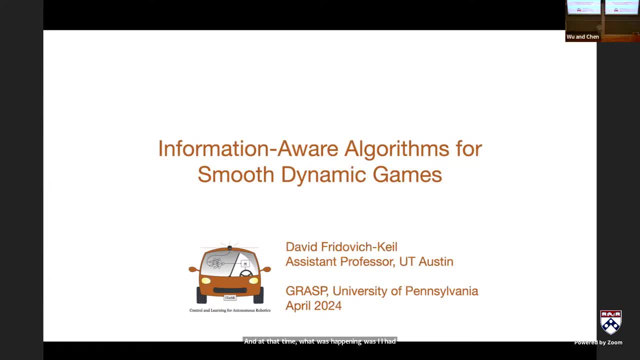 I had previous experience, exposure through my PhD with um Claire Tomlin in uh solving zero sum games that modeled robust control problems. So, uh, we were interested in say, making sure a quadcopter could reliably track a trajectory and exactly. 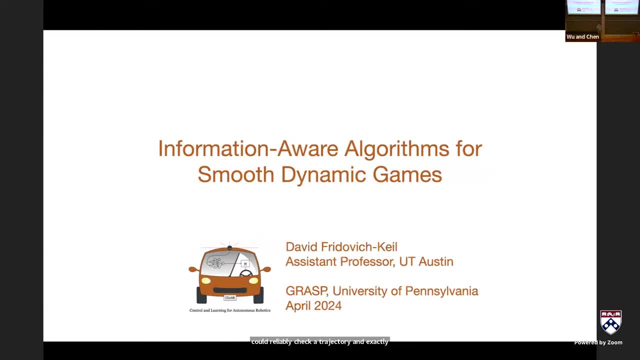 characterize the- you know- margin of error it might have when tracking that trajectory, so that we could make a hard guarantee: Hey, this thing is not going to hit the wall or whatever. Um, and so we- I was familiar at the time with 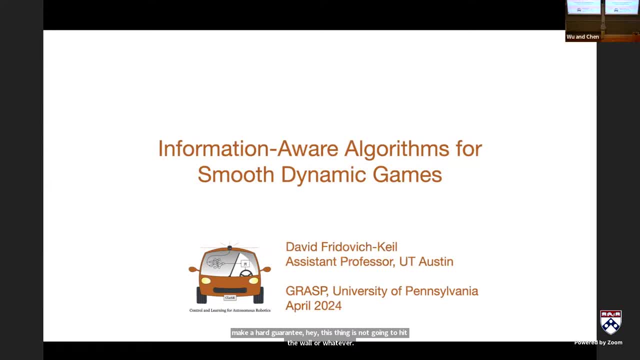 with casting that kind of problem as a zero sum game played over time between- uh, you know the protagonist, uh, you know myself controlling the quadcopter and uh, the antagonist. you know nature, um, you know injecting some kind of disturbance over time And uh. 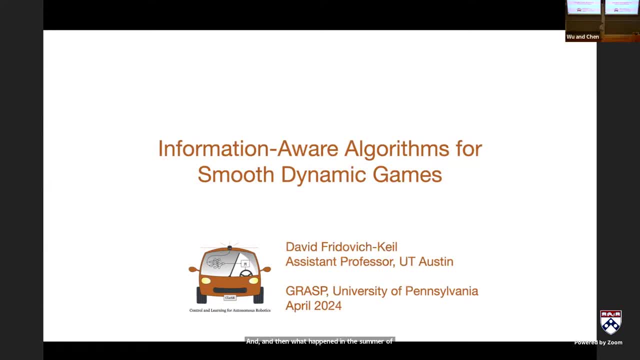 and then what happened in the summer of 2018 was I went to uh, turned out a self-driving car company and I was working on motion planning. and I got there and they basically told me: um, you know, Hey, uh. 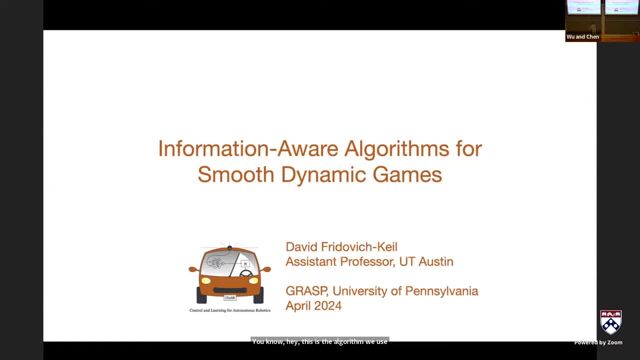 this is the algorithm we use to do planning. Um, you know, we solve some kind of MPC problem and that's how we do it. Um, and then we have this gigantic software stack that you know, does some fancy perception and predicts uh. 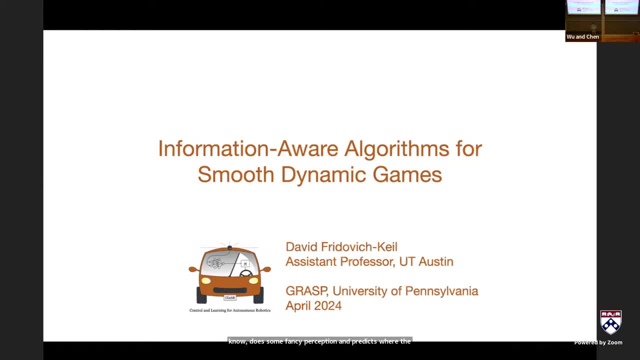 where the rest of the world is going to end up in the next few seconds, And then, and then we try to react to it via model predictive control And um, and so we had all these these problems that I was dealing with and, uh, what? essentially all of them. 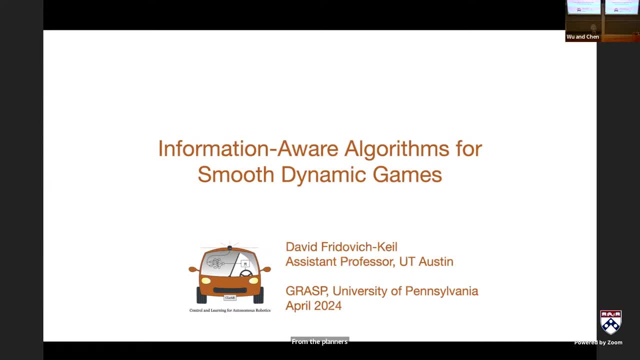 From the planners perspective, boiled down to was a mismatch between you know what we predicted would happen and, uh, how we reacted, And so we were basically spending all day long trying to fix those kinds of mismatches, And then the predictor would um make some change. 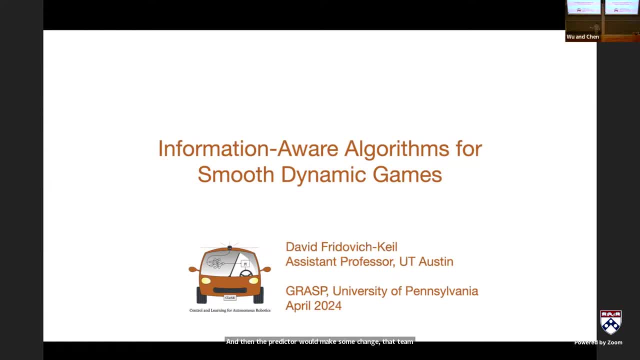 That team would push a push, a new feature. It would break everything we did, And we'd have to react. Um so we had this joke that was: um Hey, prediction, you guys should just like predict what we're going to do at the same time. 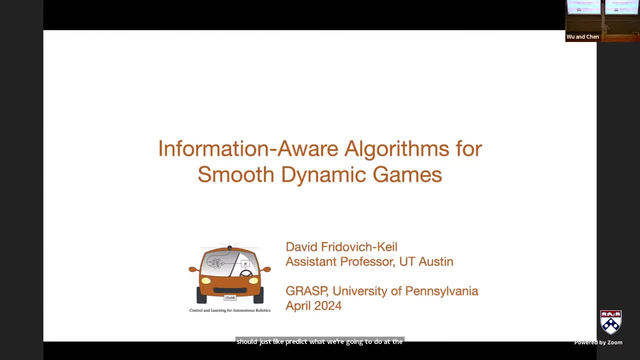 And then the planner. you know, we can just go home, You can fire all of us, So, uh, so I kind of was thinking about this through that summer and realized they were actually right. So really what was going on? was that the planner and the predictor? 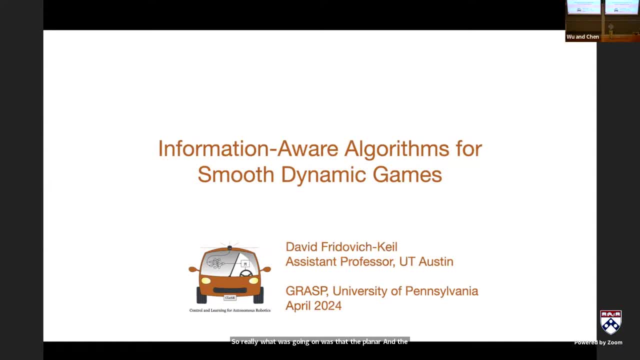 like these were being. you know, these were solving problems that were being treated sequentially. Let's predict what's going to happen, based on what we saw over time, And then let's react. Let's react to it. That was a sequential process, but really, um, you know. 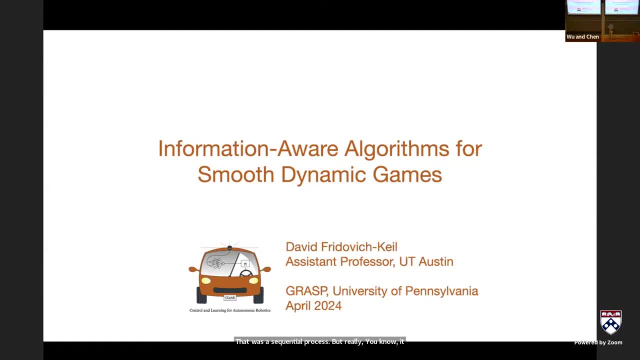 it was neglecting the fact that what we plan to do will influence what others see in the future and how they'll react, And so the actions we choose to make in the future are going to impact what we see in the future, And so we can influence other people. 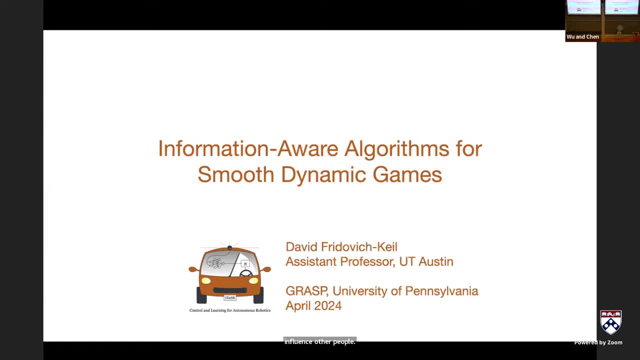 And you had to treat that problem in a coupled way, And so that got me thinking about, um, in player interactions, framing them as games that are, you know, non-cooperative perhaps, and, uh, how to solve this problem. 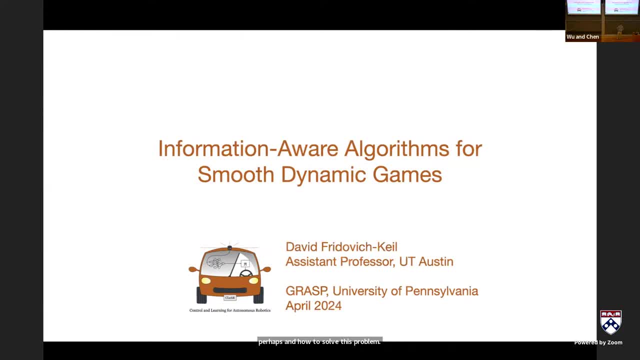 So I kind of went to my boss at the time at this internship and said, Hey, I think this is the right way to think about this problem. And he was like, yeah, sounds good, but uh, I don't know how to solve any of those problems. 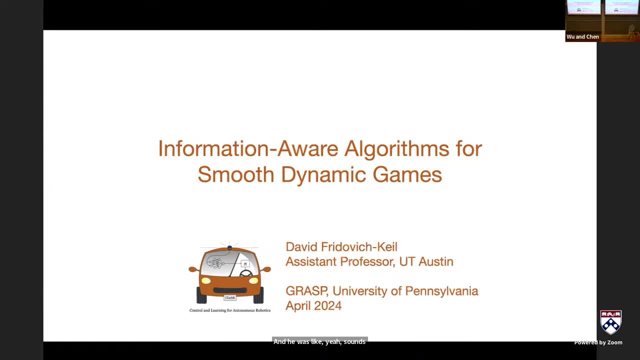 And so that that's kind of why I've been working on it for the last five or six or how many years, since 2018.. So, um, okay, So that's a long winded way to say- I'm going to try to tell you about some algorithms to solve games efficiently. 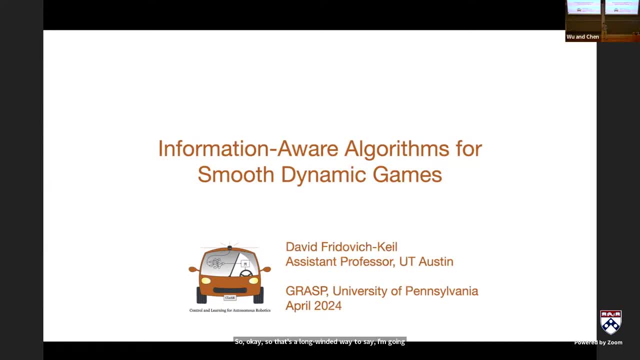 or at least these specific types of games. And, uh, what the real theme of the talk is is to kind of show you that the algorithms that you use to solve these particular problems encode something about the information structure of the problem itself. 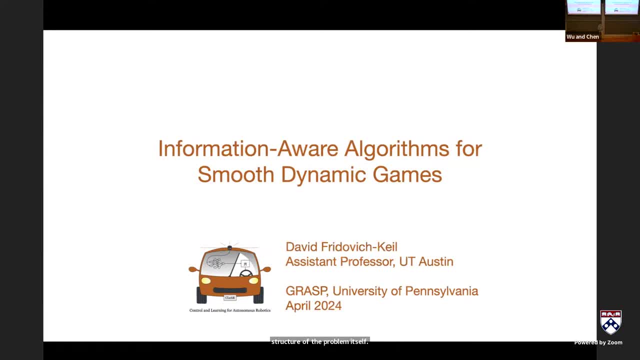 And by information structure I mean what information does every player have access to when they need to make a decision? So this will all hopefully become clear throughout the talk. It's a bit of a tutorial and then you'll kind of smoothly see a research topics. 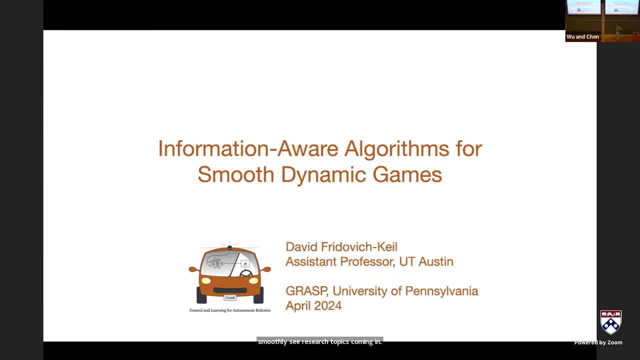 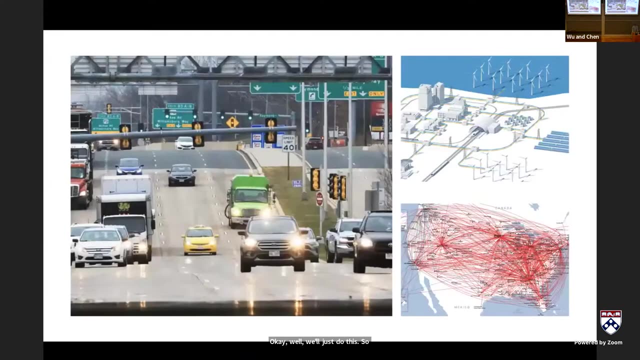 coming in. So that's the plan. if I can get this thing to work, Okay, Well, we'll just do this. So great, Perfect, Okay. So, um, I've told you about how I, how I encountered these. 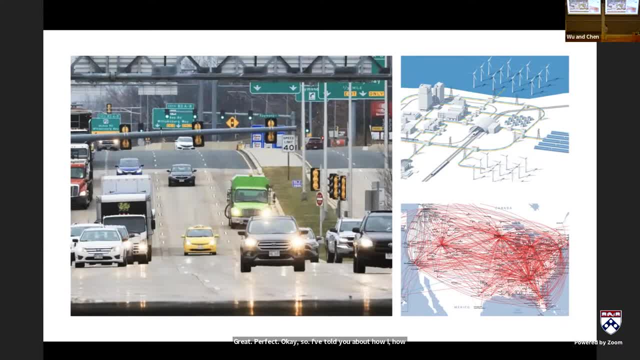 uh, game problems in terms of autonomous driving. That's obviously on the left, Um, but uh, if you're not so interested in driving, the same kinds of problems arise all over the place. So in particular, I've become recently interested in like aircraft routing. 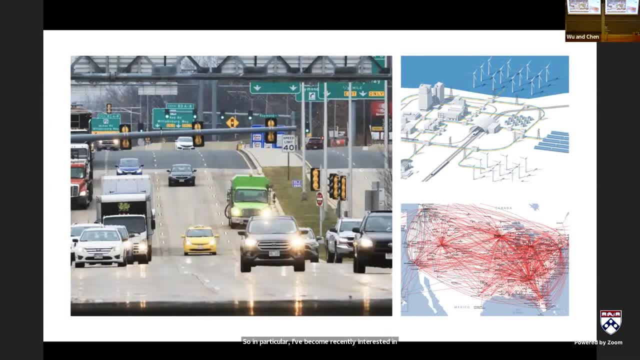 Um, as another instance of these problems, I'd love to learn more about, uh, you know, power flow. I think the same kind of models will appear there too. But anyway, for the purposes of this talk, uh, I just want to keep. 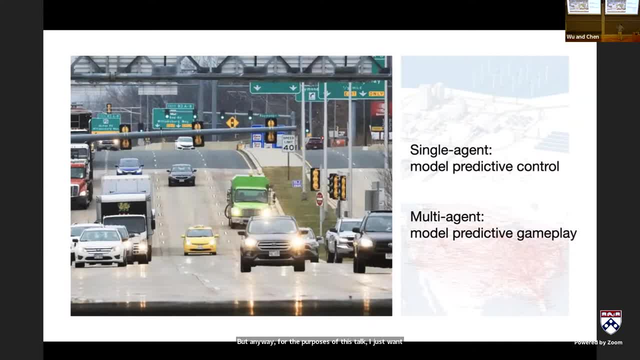 uh, traffic as the running example. So we'll be thinking about traffic problems as kind of the natural instantiation of these games And if you're thinking about traffic, if you're working at one of these companies, like I was in 2018,. 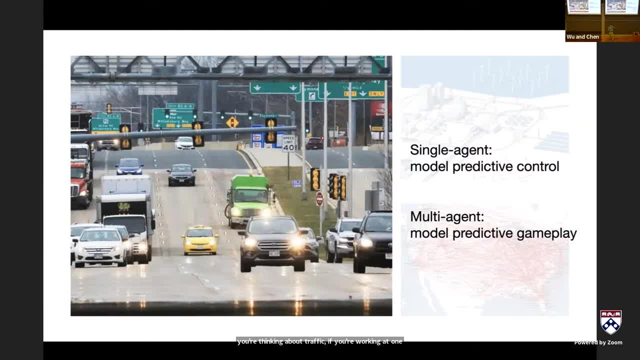 um, you know you'll be thinking immediately about model predictive control as the kind of paradigm for planning, for decision-making, Um, but in this talk, uh, we're going to be talking about games, And so you can think about. 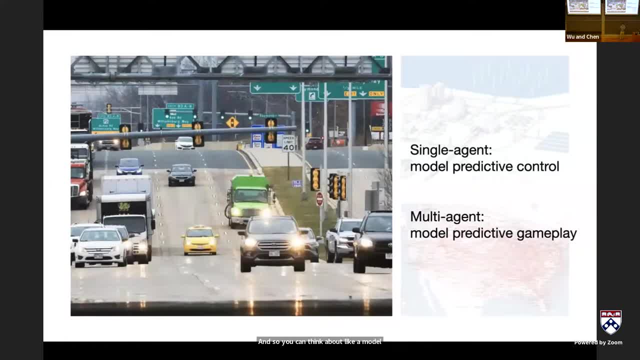 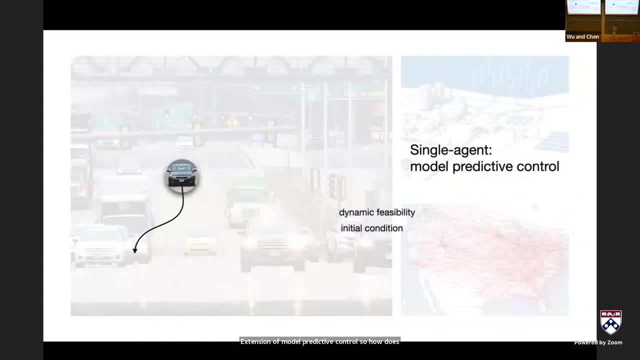 uh, like a, a model predictive game play as the natural end player, uh, extension of model predictive control. So how does this all look? Uh, basically, if you're oops, sorry, if you are right here, if you're this, 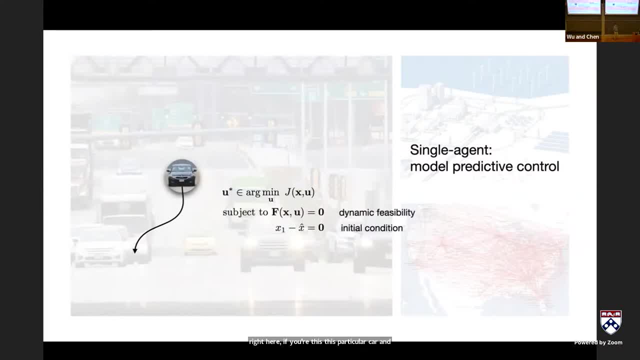 this particular car, um, and you're trying to figure out what to do in the next few seconds. uh, what you probably want to do is, uh, think about some um function J that uh maps your trajectory, your states X and control inputs. 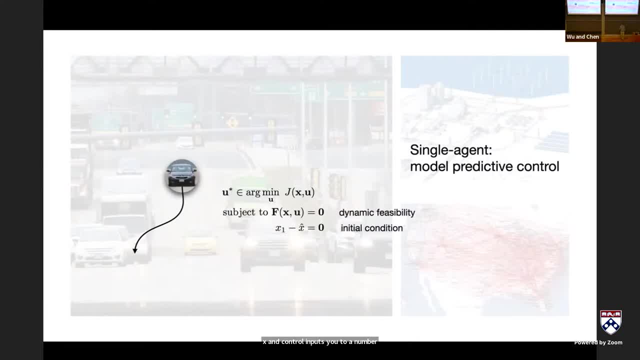 you to a number and you want to minimize that number, You probably have to satisfy some constraints. So here I just wrote down some. you know, physical vehicle, uh, dynamics constraints. That's that first one. Uh, maybe you need to satisfy some initial. 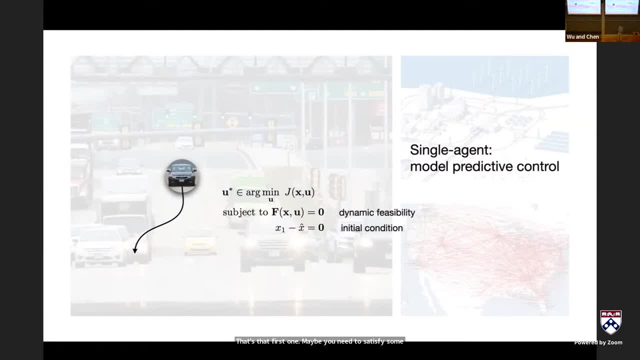 uh, condition. Maybe you know exactly where you are and what your vehicle state is anyway. Um, you want to solve a problem that looks something like this: to determine the optimal trajectory to follow. Um, but in, in reality, uh, that trajectory is going to depend on what other vehicles in the scene. 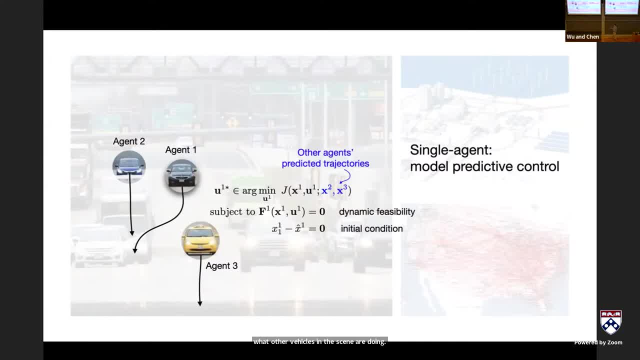 are doing So in particular. you know a really easy way to um see this connection would be to look up at that objective and uh realize that you know what. uh, you know what. the first car. 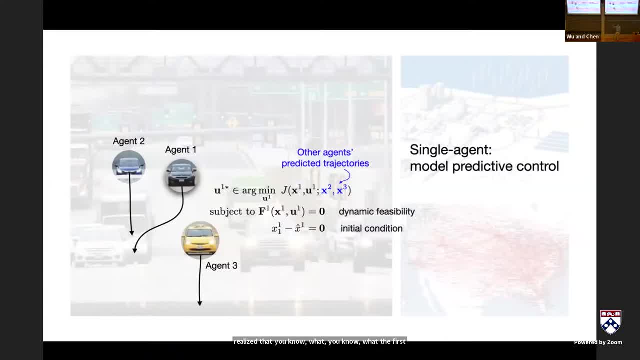 uh, thinks of its trajectory depends on what it predicts those other- you know two other cars in the scene- are going to do in the future. That's the what I've highlighted in blue. Okay, Um, so you know where does the game arise? 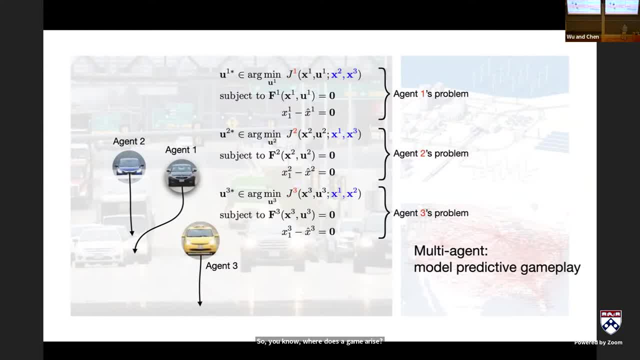 Basically the, the, the game theory kind of framing of this problem would be to say: okay, well, those blue things I highlighted before the trajectories of cars two and three, um, well, really, those are themselves. uh, you know, they arise from optimization problems that are faced by those drivers. 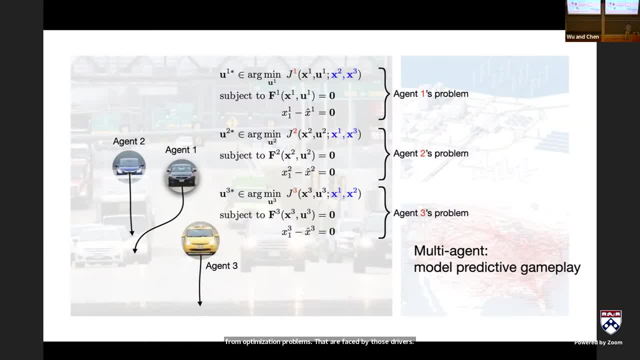 So driver two and driver three are solving the same kind of problem that you know we, the uh autonomous car number one, are trying to solve And all of our variables are kind of mutually coupled and the coupling I've written it down in terms of the player's objectives. 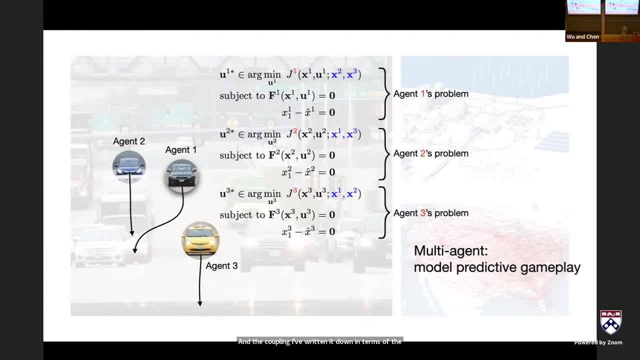 Maybe it arises in constraints too. Um, but anyway, as soon as you take this perspective that uh, the player's decisions uh impacts one another's objectives, um you are, you have a game, Okay, So this is. 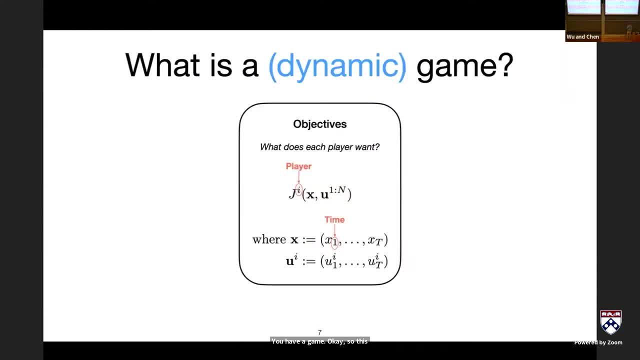 I think, a pretty natural way to see these things arising. Um, let me tell you a bit more about, uh, you know just what are we looking for When we talk about these, these games. So, um, so, any of these games. 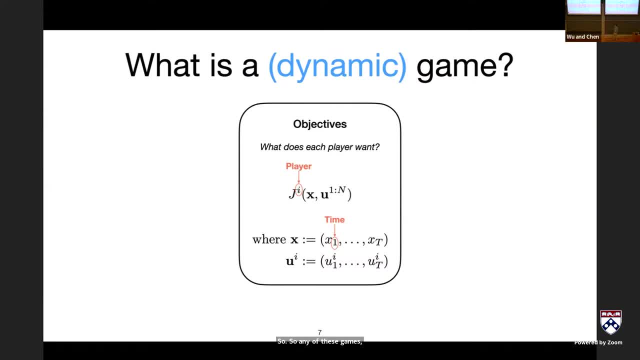 it's like I'm talking about games that are played over time. Uh and um. so every player you know obviously has an objective that they're trying to minimize here. Um, there's a state of the game, Uh. 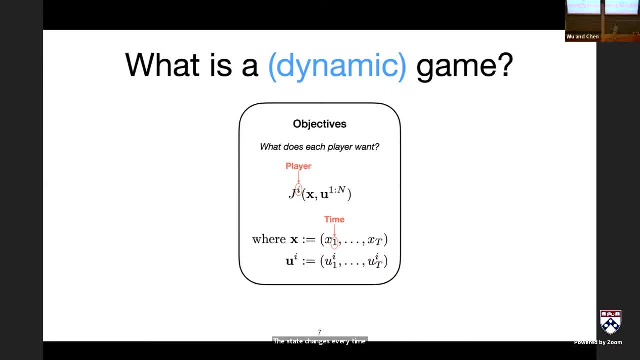 the state changes every time. step. Uh, every player has a, you know, an action that they can make at every time. Um, there are rules of the game, dynamics to the game. So, um, if it's a vehicle, these are just. 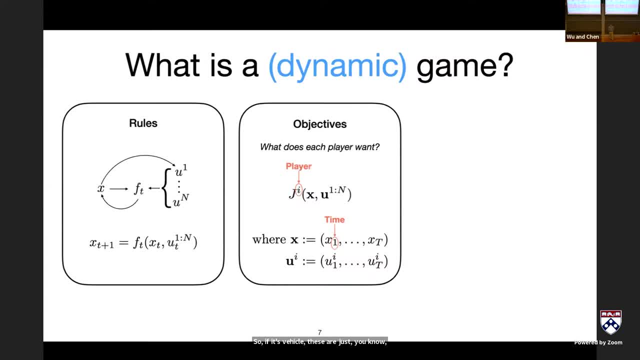 you know kinematics or dynamics. If it's a game of chess, it's obviously the rules of chess. Um, uh. and then the kind of critical part that I'm going to focus on for most of this talk is the information structure. 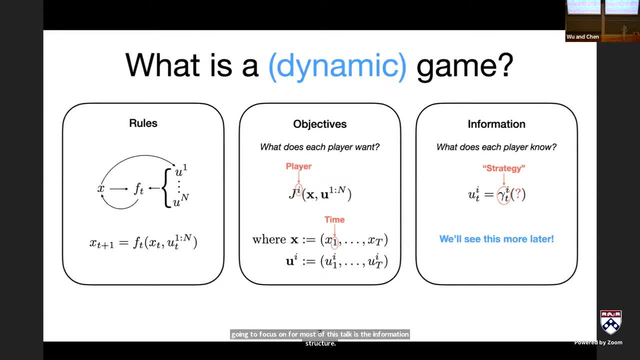 What does every player have access to when they have to make a decision? So, um, so. we'll see a lot more about that later. And then the final question is: what do we look for? So, given you know, if I tell you all three of these things, 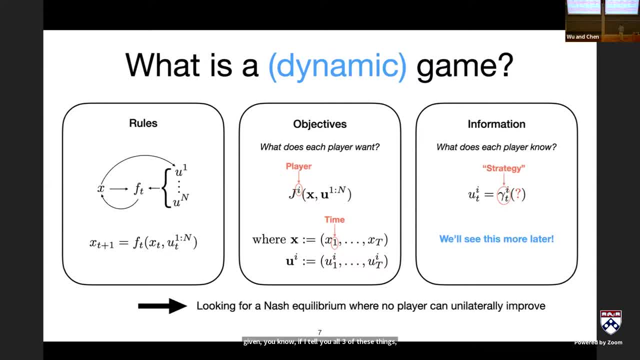 um, what? what kind of solution am I looking for? Uh, so in this talk, uh, we'll be talking about Nash solutions, but I'll actually kind of allude to a few other solution concepts at the end. The the bottom line is: 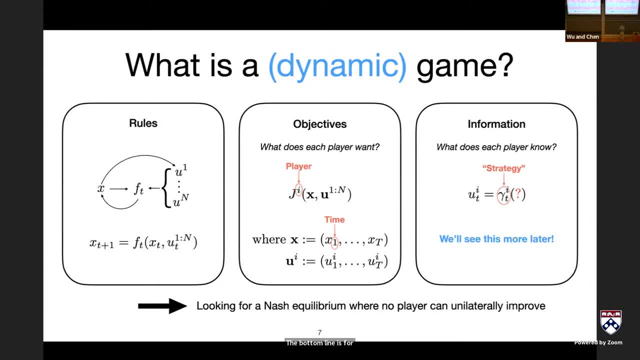 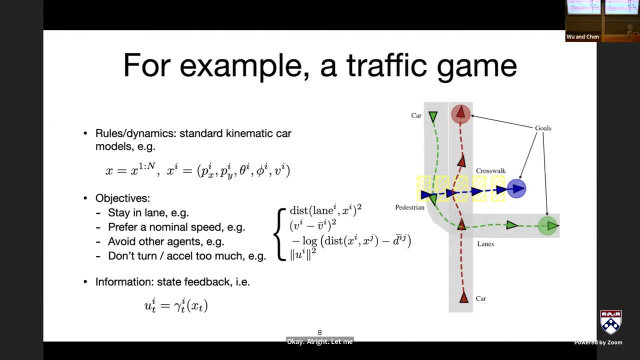 uh, for a Nash solution. we're looking for a point in the strategy space where no player can unilaterally improve. Okay, All right. Uh, let me instantiate this a bit. So, um, if we're in, uh, 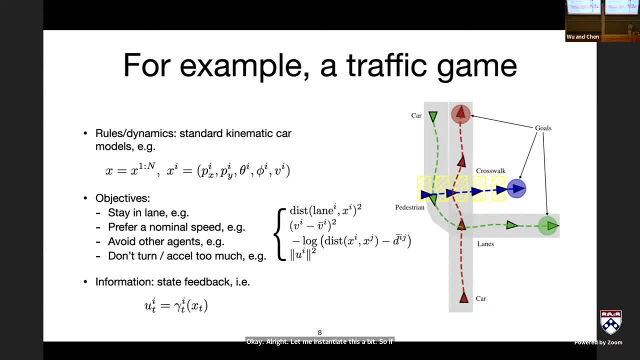 one of those traffic problems. um, you know, maybe the dynamics are just given by the you know some model of the vehicles. So, uh, you could keep track of whatever states you think are, you know, important for that model. 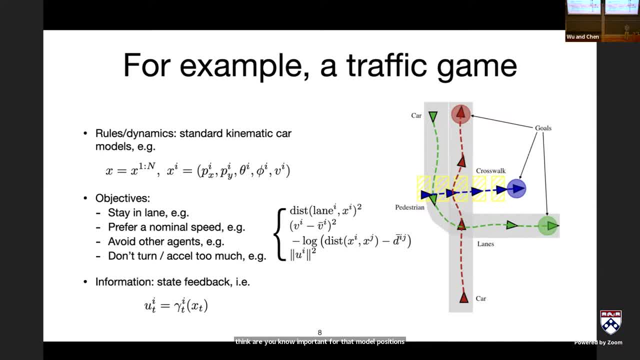 uh, positions, headings, et cetera. Um, you could model every player's objective, as you know, maybe like a linear combination of preferences that I've alluded to here. So like staying in the lane um maintaining a speed limit. 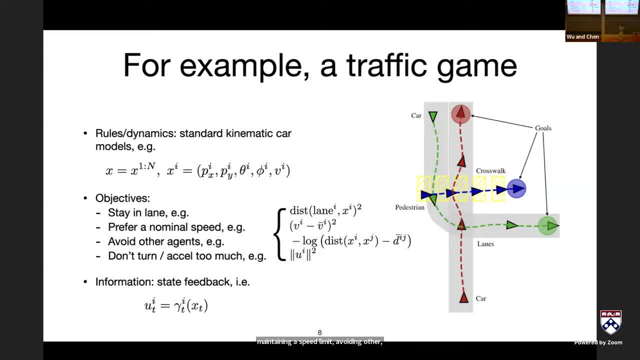 avoiding other, you know, avoiding collisions, things like that. And maybe you can model the information structure uh as state feedback. So maybe uh say every player gets to observe the full state of the game. Where is every other vehicle when they make a decision? 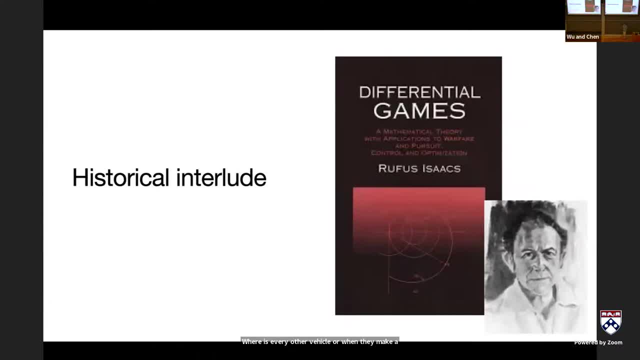 Right, Um, these problems have been, you know, widely studied for a really long time. Uh, and I I find the history like quite fascinating. If anybody wants to learn more about this, this book is, uh like quite good. 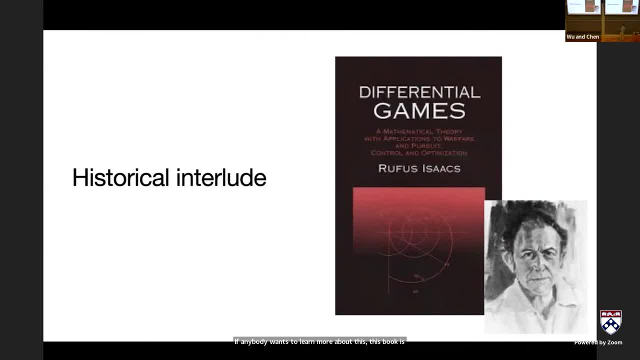 Um, especially the first first chapter or two, I think. But, um, but anyway, this theory all goes back to, uh, a man named Rufus Isaacs who was um publishing, uh, you know, tech reports for Rand back in the late forties and early fifties. 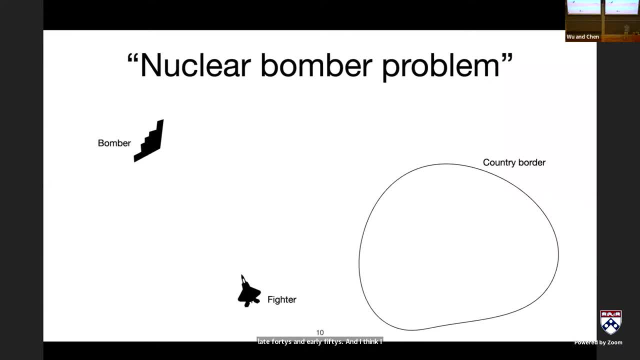 And, um, I think I just can illustrate the basic idea of this early work and kind of two quick, kind of little little brain teasers. So the first one, uh, I think he called it something like the nuclear bomber problem, but 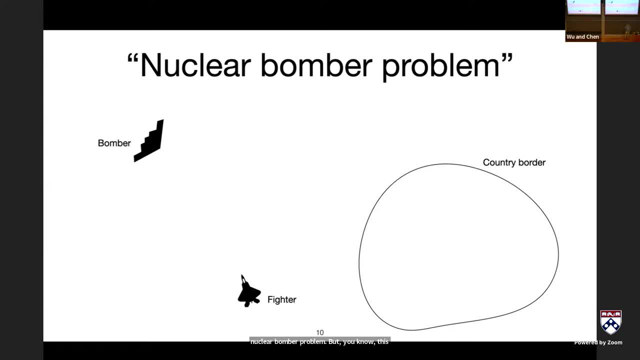 but you know this is late forties, early fifties, Um, so you can imagine what was going on at the time. And and there's a bomber, uh, that's trying to, you know, drop a bomb somewhere in this. 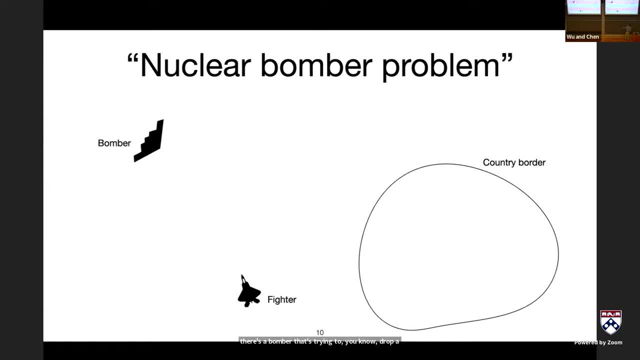 this, you know, near this country And there's a fighter And the idea of the game is: how can the fighter shoot down the bomber as far away from this country as possible? Uh, and you know the other. the bomber wants to do the opposite. 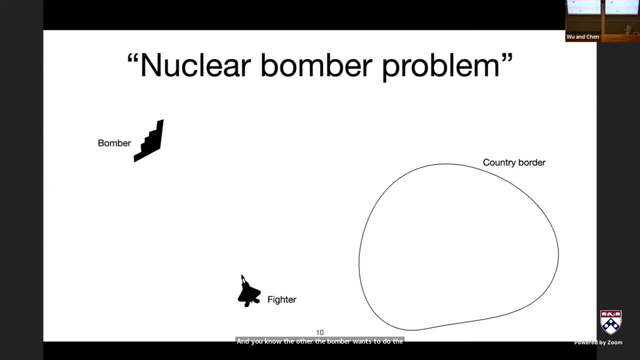 The bomber wants to, to drop its bomb and get shot down as as close to the country border as possible. So, um, so, uh, anyway, what's happening here is, if you think about it, um, and you kind of make very simple assumptions about how the planes can move. 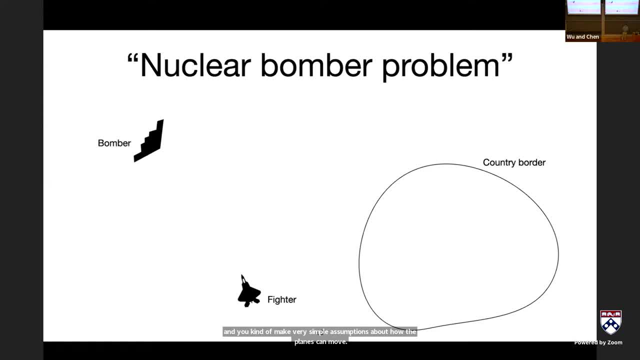 um, you'll realize that there's a very nice geometric solution to this problem, And this is the kind of thing that Isaac's was. um, you know, Isaac's examples were, were like particularly elegant about this that there was. he could often find some. 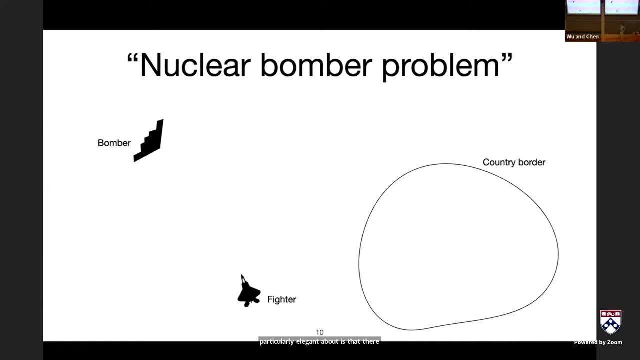 some very nice embedded geometry to the problem, So, um. so in this case, what you do is you basically draw the perpendicular bisector to this line and realize that, okay, at that red point, um, this is the the point at which 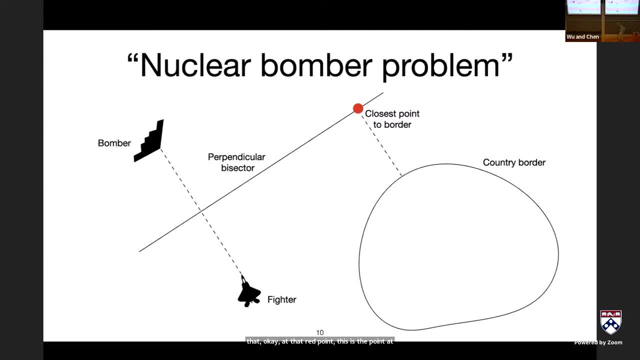 um, you know the bomber and the fighter can get there at exactly the same time, uh, if they're moving the same speed and it's the closest of. you know those points on the bisector to the country. So basically, the best thing for the bomber to do is to just go straight to. 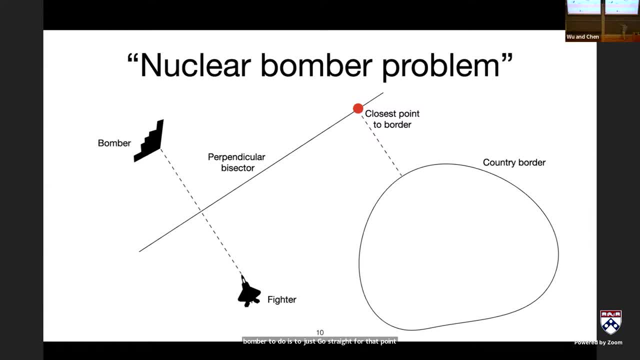 that point The fighter. if the fighter does anything other than go straight for that point, the bomber could get closer. Uh, and so basically the best thing for them to do is just make a beeline there, and you can, and Isaac's basically proves that. 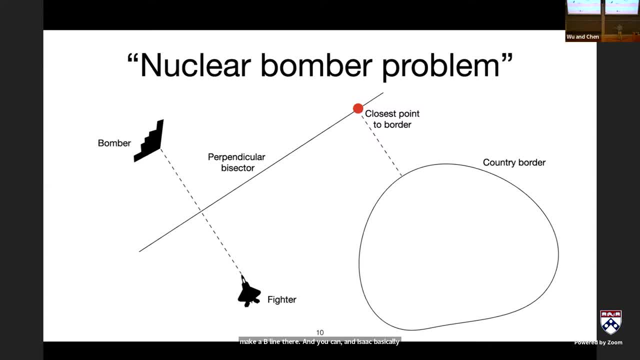 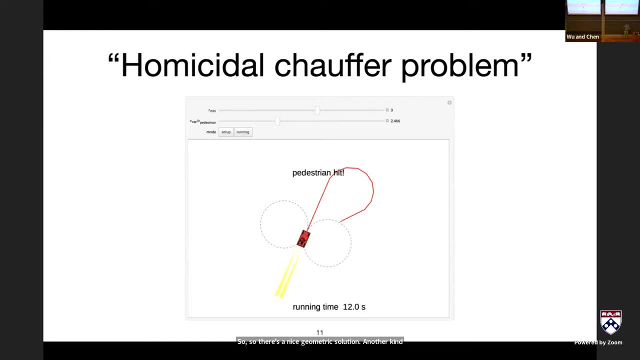 uh, if they do anything other than that, it's exploitable. So, um, so there's a nice geometric solution. Another kind of classic problem with a nice geometric solution is called the homicidal chauffeur problem, where you know, in this case, 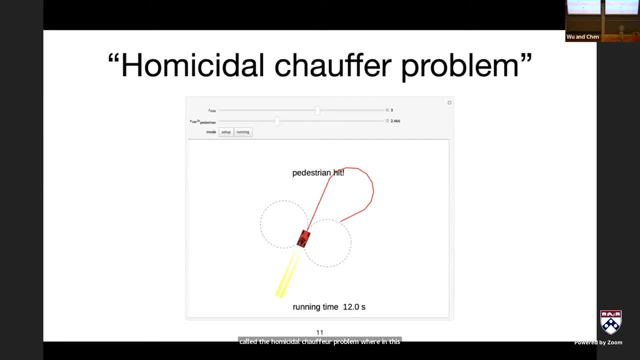 like: uh, it's a lightly disguised version of a missile guidance kind of scenario, but basically, uh, the you know the there's a car that's trying to run down a pedestrian and the car has a heading angle. The pedestrian can run any direction they like. 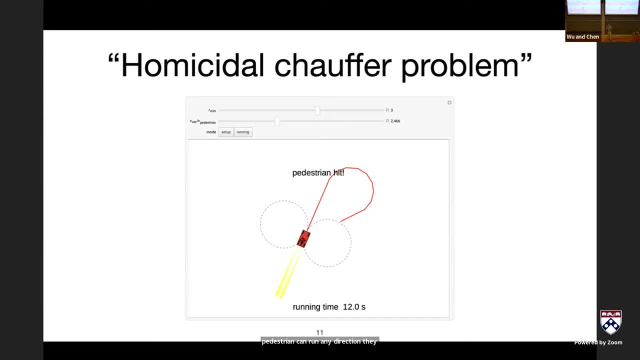 And there's again, like this very cute geometric answer, um to how, how can the car best run down the pedestrian anyway? So so Isaac's basically came up with this theory to describe these problems And because it was essentially the early fifties. 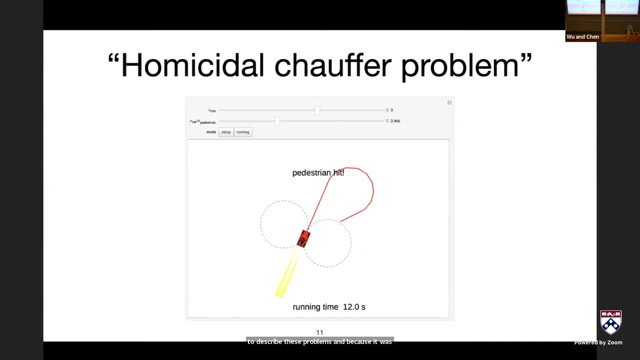 there was not much computation to speak of to solve them, So he was reduced to basically finding simplified cases that afforded a nice geometric answer. And uh, you know, in the general case, what do you do? Uh, basically, what you do is: 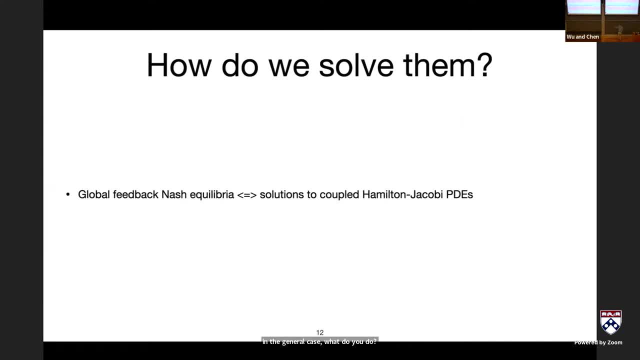 and he realized this, is that the, the kind of global feedback equilibria of these problems are characterized by coupled PDEs. Um, and because there was not much computation at the time, um, he resorted to geometric solutions, although he did characterize. 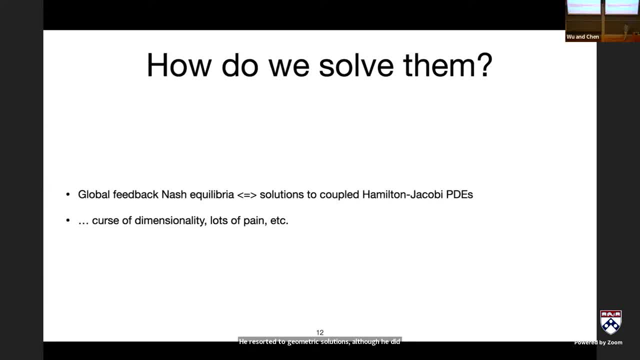 uh, properties of, of solutions to those PDEs more generally. Uh, but, but now it is um. you know we can do a bit better job of solving these problems, but we still hit, you know, issues of curse of dimensionality and become unhappy pretty quickly. 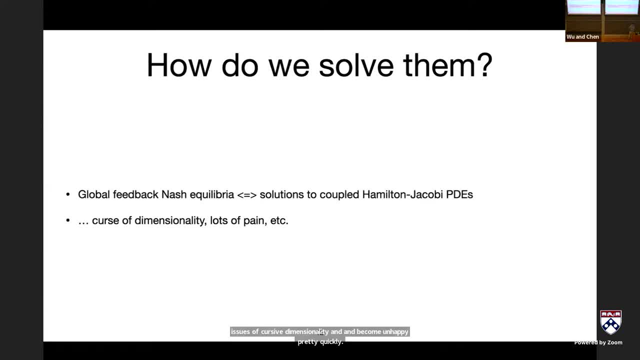 So this is where I guess that the real meat of today's talk starts. What do we do, Like if you, if you are faced with these issues, what can you do? And I'd say the answer that I want to kind of 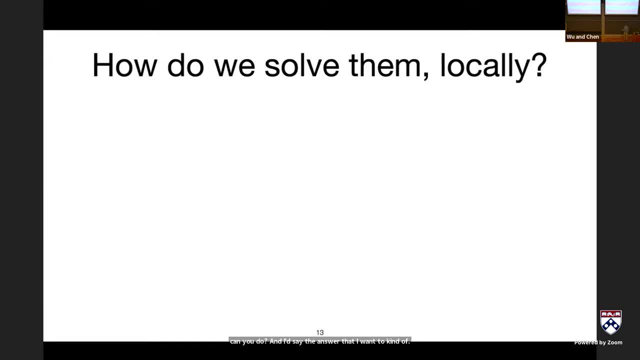 uh, put forward is that you can look for other kinds of solutions, You can look for local solutions. So how do you solve these problems locally? So the way to do that, do this, is to think back to those coupled optimization problems I wrote down at the very beginning. 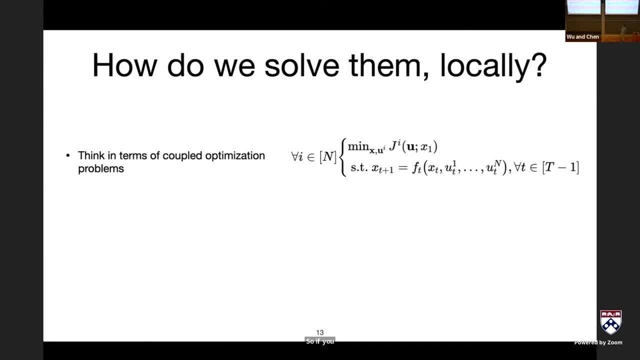 So if you write- didn't write them down like this- um kind of the first intuitive thing that people did was basically to think about some kind of iterative scheme and try to say, well, uh, if, if players two through N have fixed their strategies, 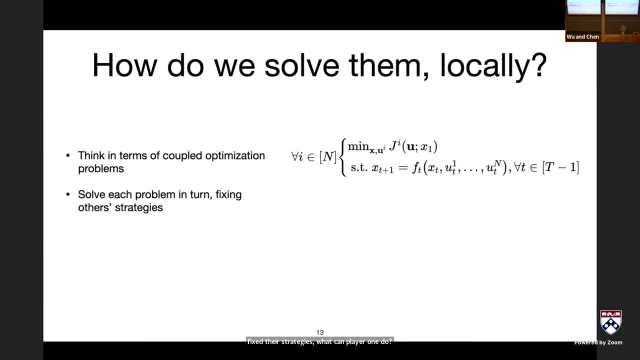 what can player one do? What's player one's best response? Um, and then, uh, player one can declare: this is my new strategy. Player two can say: okay, well, given everybody else, what do I want to do now? 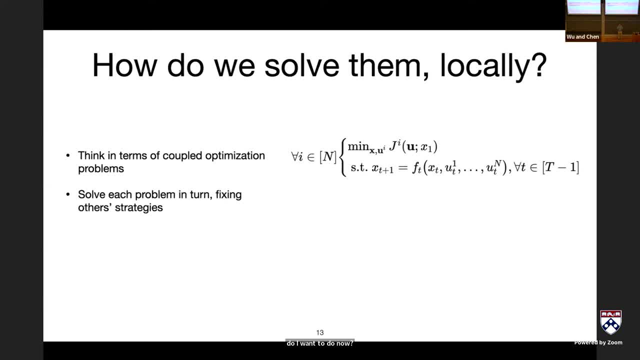 Um, and you can kind of repeat this process. Maybe you can randomize the order. There's all kinds of variants, but that's a pretty intuitive thing that people started doing very early. Um, the issue is that, uh, at least naive versions of this have convergence problems. 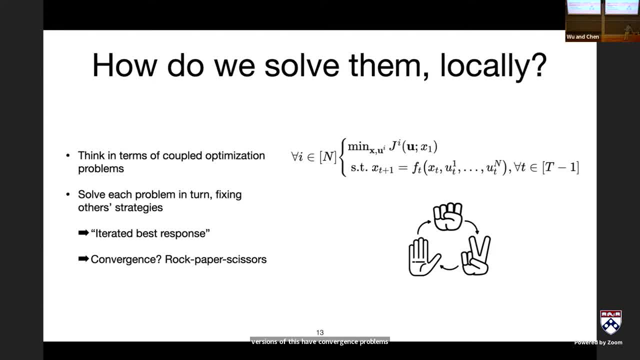 So, um, so you can even just think about rock, paper scissors as like the classic, simplest example of where these kinds of things will fail. If, uh, if I say, uh, I'm going to play rock, then of course somebody else will say: 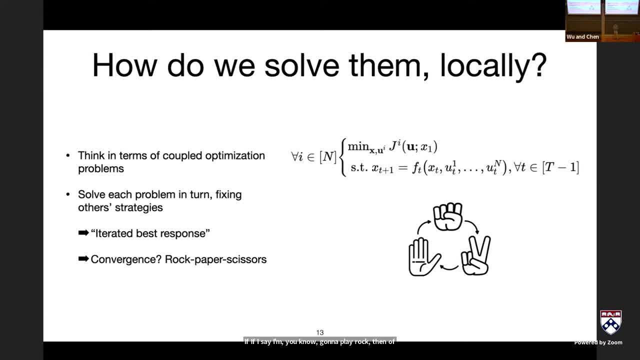 uh, they're going to play paper, and now I don't like rock anymore- I'm going to play scissors and we're just going to end up cycling around and around and around. So, um, there's obviously a lot deeper theory here, and there are cases where these kinds of schemes will work. 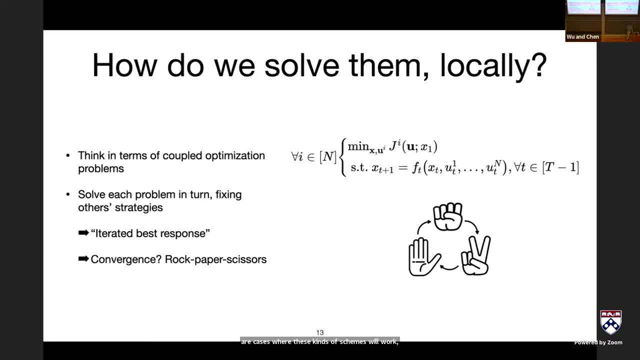 But uh, you know, let's, let's see if we can do something a little smarter. So think back to these problems again. And if you didn't see the for all, I um, and you just saw like one version. 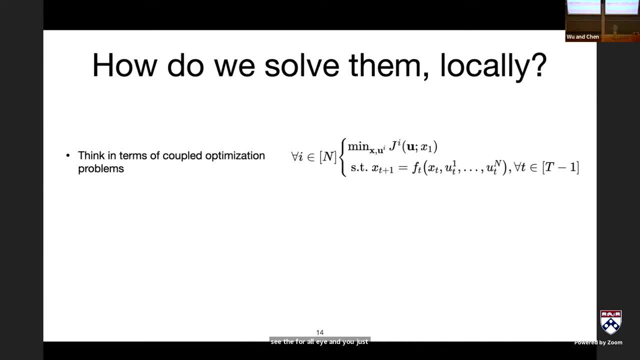 this optimization problem. uh, I guess what would be your knee jerk reaction of how to solve this problem locally. Who's taken optimization class? Nobody, Really, Okay, Uh, how about a constrained optimization class? Yeah, Okay, How about like a little bit more detail? 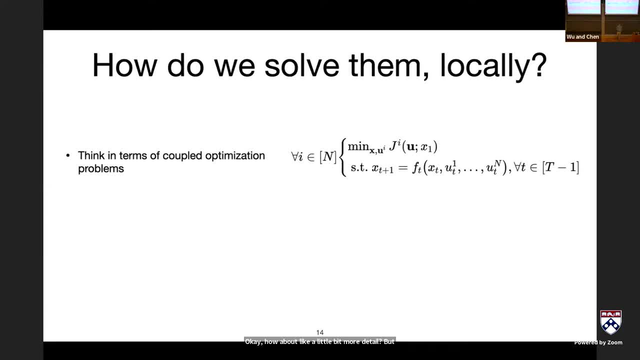 But sure, Okay, Somebody has taken it already, but it's not even necessarily convex. Okay, All right. So that's an algorithm, That's good. Um, but what would you look for, Like w? how would you know that you found the right answer? 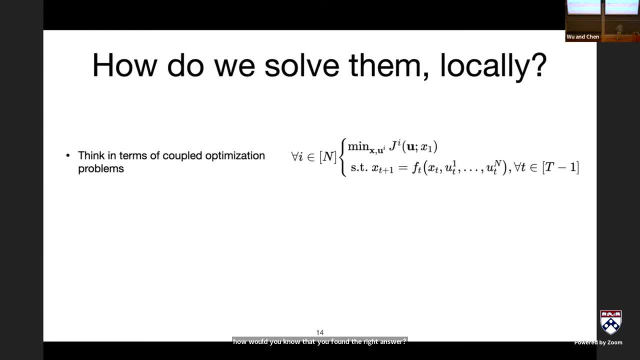 Like, how would you, how would you write down that algorithm? Like what's it trying to do? Okay, I'm looking for three letters. Two of them are the same. Yeah, Okay, You basically write down the KKT conditions for this problem. 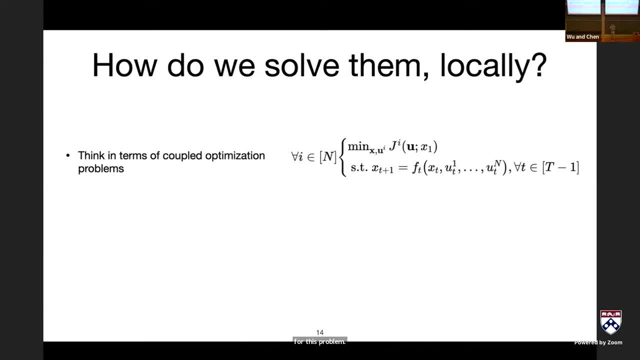 and then you'd try to construct an algorithm that's satisfying those conditions, And then maybe you check the second order conditions too. All right, So here you can do the same thing. You can just write down the KKT conditions for every player and stack them all up. 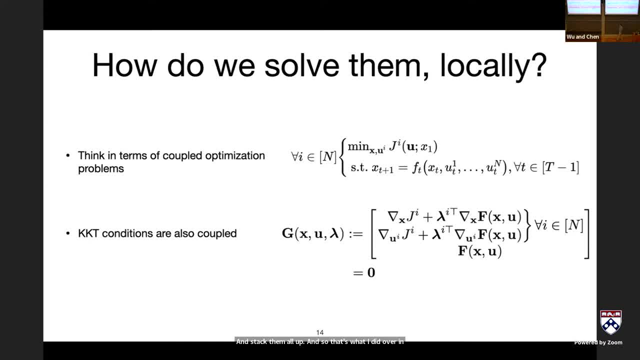 And so that's what I did over in the bottom right, Um and and notice, I guess I'm I'm being a bit, um, intentionally careful here to just include equality constraints. So, uh, you know, I don't have to worry about complementarity conditions or anything like this. 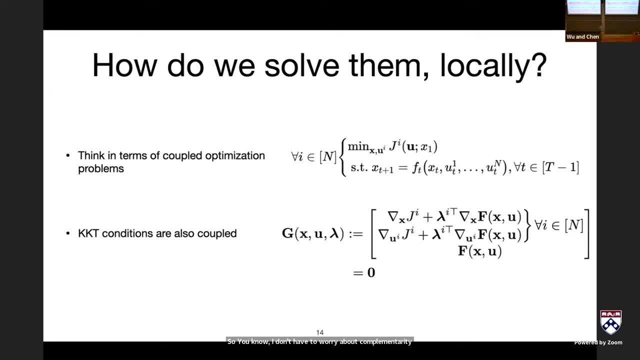 but um, but we can talk more about how to handle those if you like. Um, anyway, if you write all these conditions down, you get basically a big function of the states for all the players. the actions for all the players. 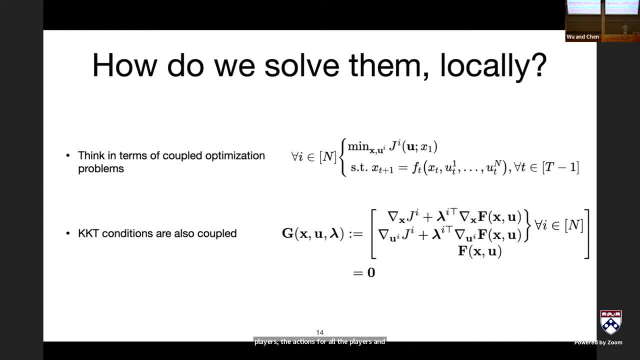 and um this uh, variable Lambda, which is just the background multipliers for all the constraints And this big G thing. you can see how it's made up, but basically it's. you can think of it as just some fairly arbitrary. 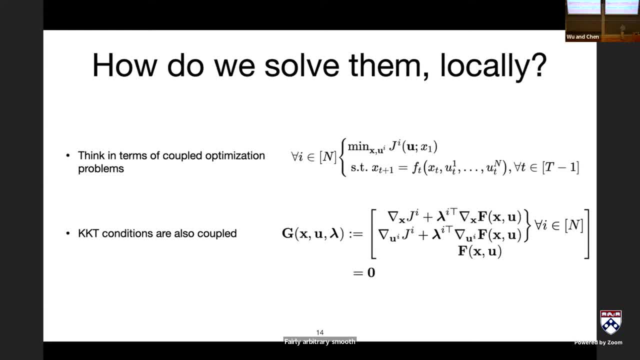 smooth, nonlinear function of all those variables. And uh well, to first order. if I satisfy, G equals zero. if I can find XU Lambda that satisfied this equation, um, I must be simultaneously satisfied satisfying all the players, first order conditions. 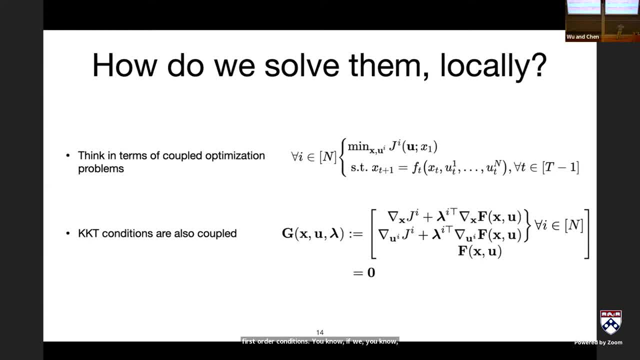 You know, if we, you know squint and don't worry too hard about the second order business, then we're, we're at a Nash solution. So it turns out, you know, basically that's that's, that's something you can do. 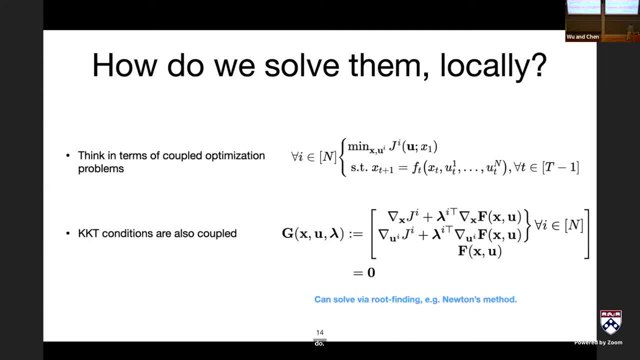 You can try to like use a root finding method, Newton's method or something to solve this system of equations. Um, it could be wildly nonlinear, Maybe, uh, maybe you have to, uh, be very careful with a line searching and trust regions and so forth. 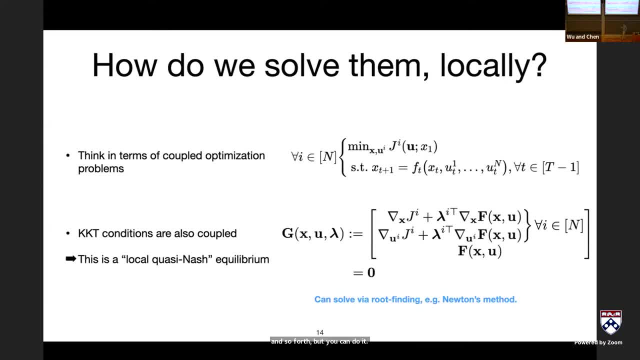 but you can do it, Um, and if you do, you'll find, uh, you know, something called a local quality Nash equilibrium. the local just because it's based on gradients, information, uh, uh, quasi Nash, just because we're only checking. 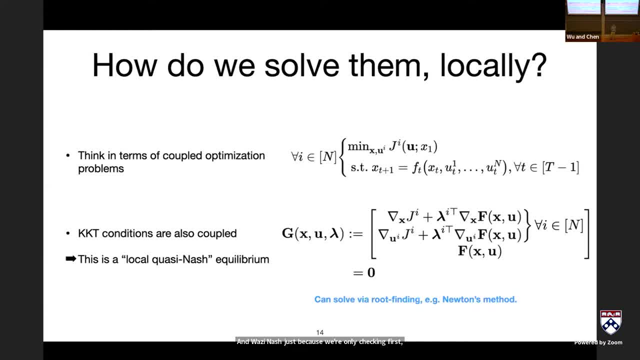 uh, first door, We're only we're not checking second order information. So basically we're looking for critical points for all the players. Don't worry too much. Basically this is a local version of a Nash equilibrium. Okay, So if we kind of take it for granted that for whatever problems of interest, 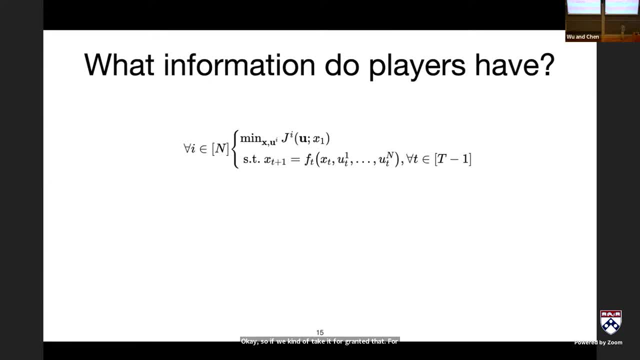 a Newton, Newton style method will work for that kind of scheme. Um, here's the interesting question to me. is suppose I do all of that, Suppose I'm looking at this problem and I've solved it with whatever variants of the algorithms you know. 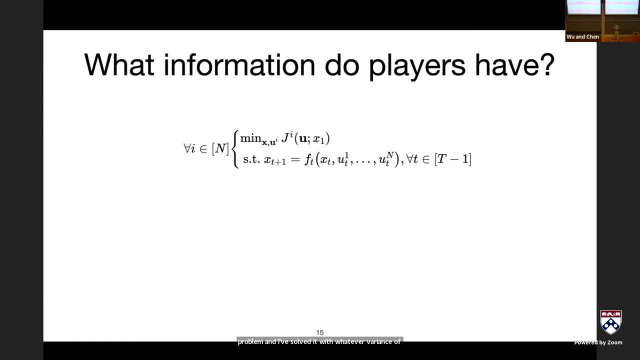 I just discussed. um, what is this inherently encoding about the information that each player knows when they have to make a decision? Let me put that another way: Um, when I solve this problem, I get a trajectory for every player, I get a trajectory of the game and I get a sequence of actions for every player. 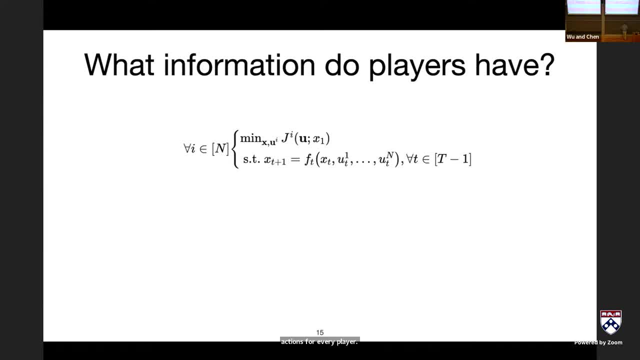 Um that satisfies their optimality conditions. in order for a player to actually execute that strategy, What information about the game do they need to know when they're playing it? Like, imagine this is a game of chess or something. Any ideas? the rules. 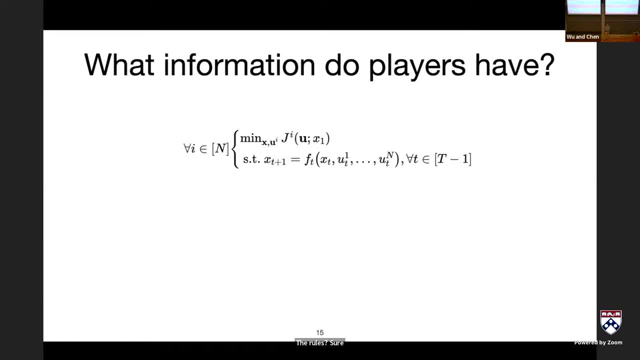 Sure, Yeah, they need some of the state of the board, do they? You'd hope, but do they? Yeah, that's, that's key, Okay so. so what's happening here is, if we solve this, we kind of get an equilibrium trajectory for the game in terms of the states and equilibrium. 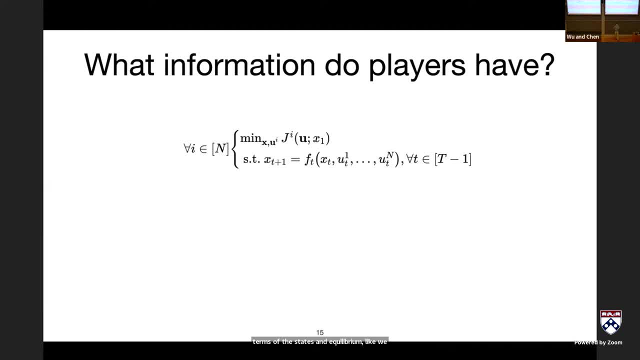 Like, we get state at time one, state at time two, state at time three. Those are decision drives. So so, if we've solved the problem, we have a sequence of states- Uh, that will hit along the equilibrium trajectory. We also get a sequence of controls. 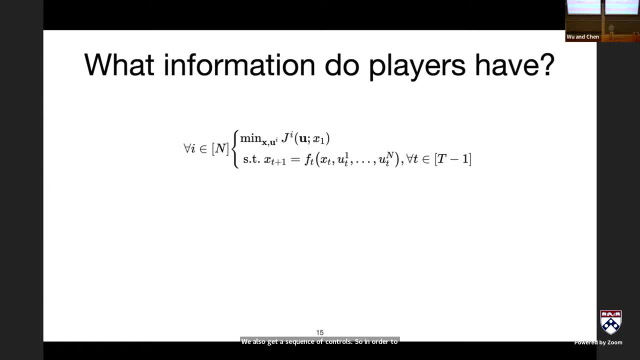 So, in order to actually execute those controls, all you need to know is what time it is, And then you can look up in your sequence of controls. okay, well, uh, my watch says it's time three, so I'm going to play control at time three. 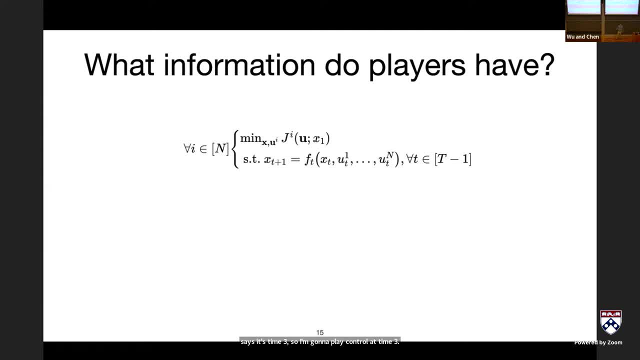 And the state trajectory will follow the dynamics of the game. So that's got a name. This is basically, uh, an open loop strategy that you're solving for Um and for anyone who's got a game, um, or anyone who's got any kind of feedback control experience. 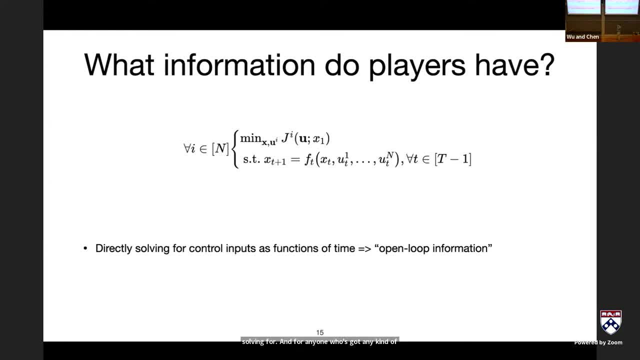 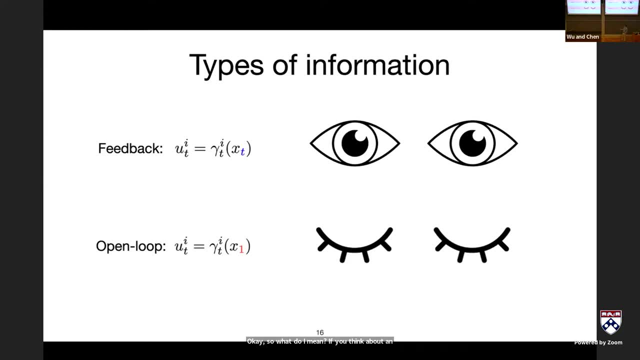 this is kind of immediately problematic, Okay, So what do I mean? Um, if you think about an open loop strategy, it's like at the bottom: uh, it's a bit uh unfortunate- the naming scheme, I think. 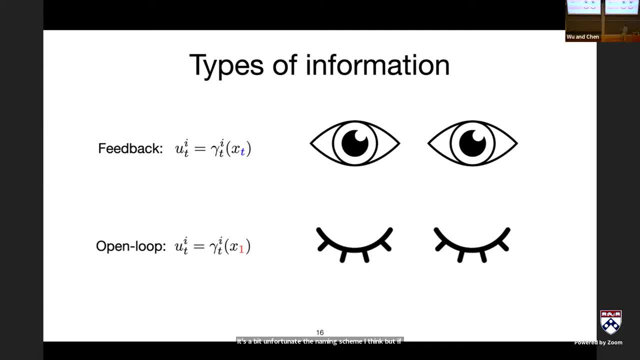 But if you're, if you want to think about what is an open loop strategy, it's basically a strategy that you can play with your eyes closed. Um right, Basically, if I'm, if I've got an open loop strategy, to like walk across the stage and get out of the room. 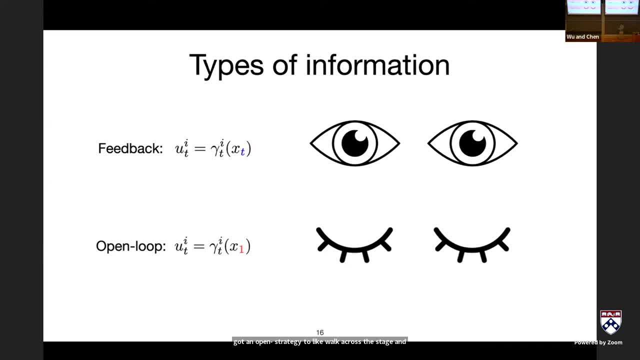 um, you know, all I need to know is, um, the sequence of steps I'm going to make. So I'm going to walk this way with my eyes closed, But of course, I don't know exactly how far it is to the. 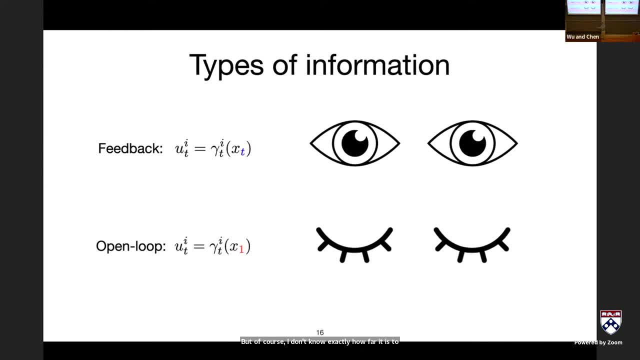 uh, stairs, And so this is a terrible idea to close my eyes while I'm doing this. Um, so an open loop strategy is, uh, a function that maps just the initial condition and maybe it's indexed by the time the subscript there on gamma. 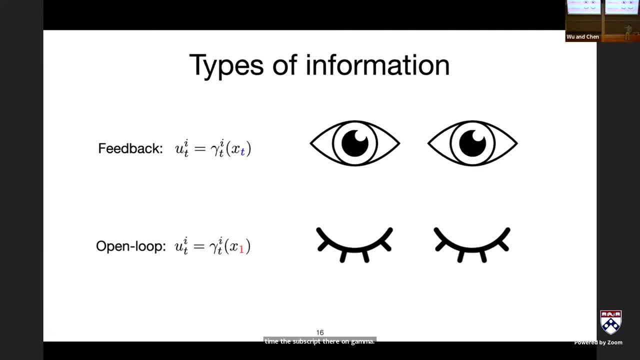 um, uh to an action. A feedback strategy is one that you kind of need your eyes open to play. You need to be able to see the state. So it's a map from uh, the state and the time to an action. 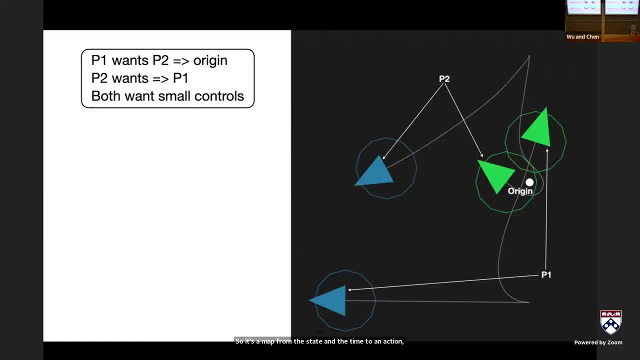 right. Um, eyes open, eyes closed. Let's see an example. Why does this stuff matter? Um, here's, uh uh, just a very toy example of a game where um player one is starting from the bottom. 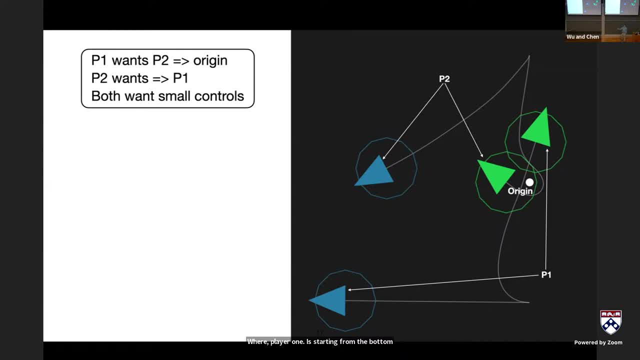 right, And they want to get player two to go to the origin. Player two, uh, is starting from way up here And, um, player two wants to approach player one. player Two just wants to be close to player one. 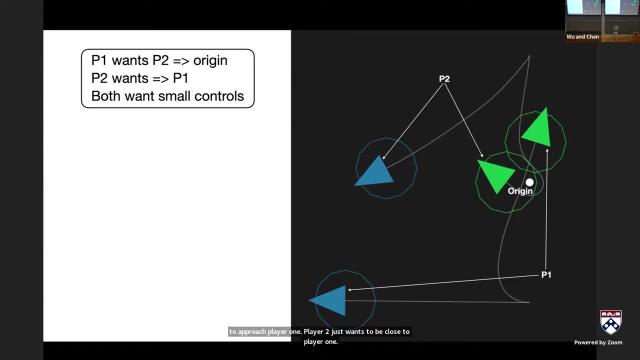 Um, both are lazy and don't want to apply a lot of control inputs. You can think of this: uh, you know, you can kind of write these objectives down as quadratic functions And maybe let's imagine that the the dynamics here. 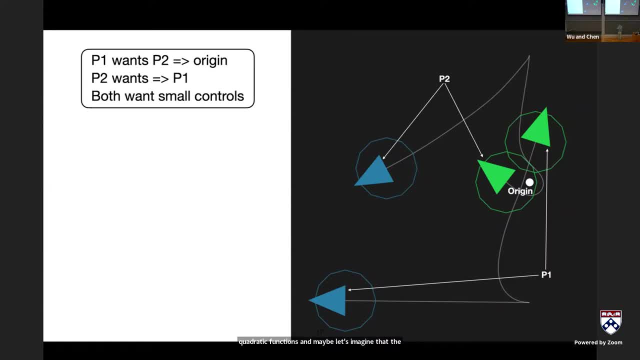 um the rules of the game. the dynamics are like uh, cars driving, So there's a heading and um uh, players can choose their turn rate, something like that. Um, I've shown you an open loop, equilibrium. 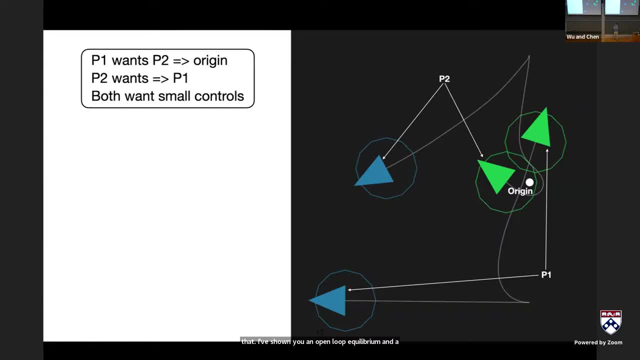 and a feedback equilibrium in different colors. Any any guesses as to which is which- by the way, both are unique in this case- lose open loop. Why? Uh, overshoots What I mean. it doesn't even get close to the origin. 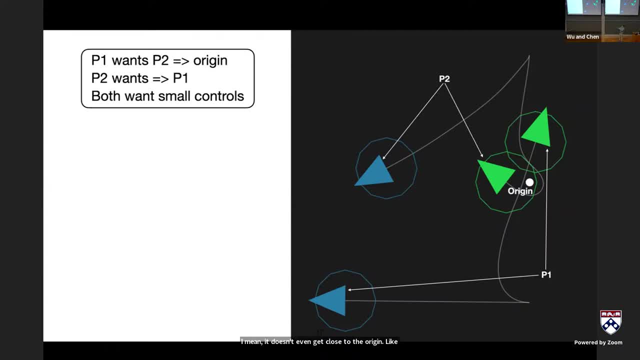 Like this guy's not even. it's more than just overshooting. You're right, actually Blue is open loop, but, um, I wouldn't really think about it as overshooting anything. What's what's happening here? Sorry? 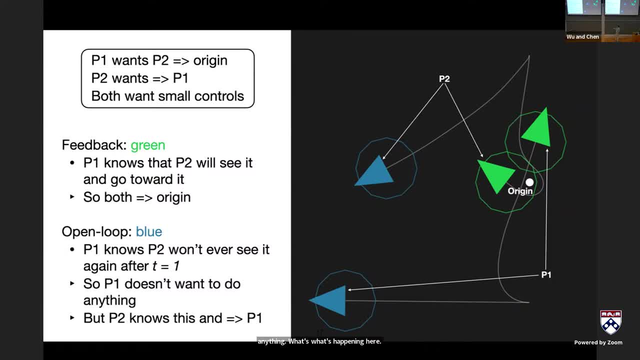 let me. So what's happening here is that in blue, player one- uh, that's the bottom guy- knows that nothing it ever does will get seen by player two, because both have to choose a strategy which only depends on the initial condition and the time. 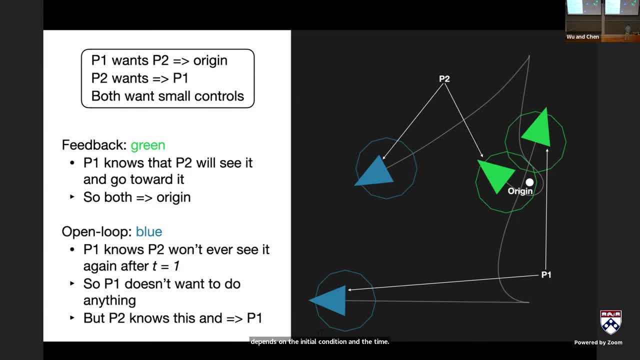 So player one knows, uh, that nothing it does will ever influence player two. So, uh, because player one wants player two to go to the origin, uh, it can't influence that component of its cost, Um, but it can certainly choose a small control. 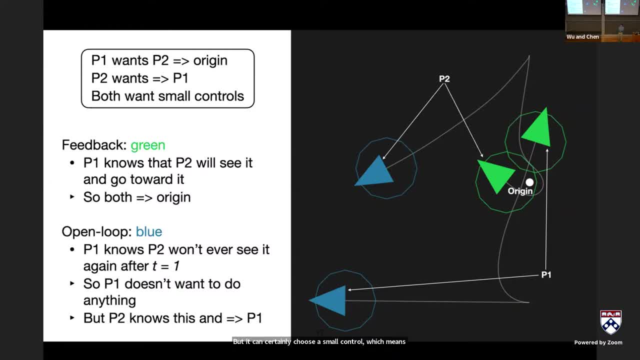 which means it can not yaw at all, And since it started moving that way, it's just going to keep going that way. Um, Similarly, player one- uh knows that's player two. Sorry, Player two. player one started oriented this direction at a certain velocity and basically it's just going. 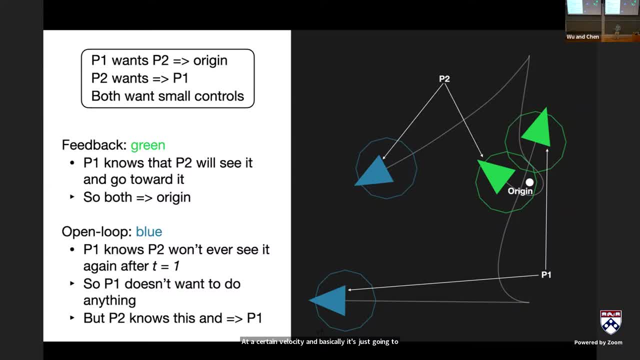 to make a closest approach. So that's the open loop equilibrium and the feedback one is maybe the more intuitive thing. It's player one knows that player two is going to get to see the state in the future. so player one knows: ah, if I go towards the origin, player two is going to want. 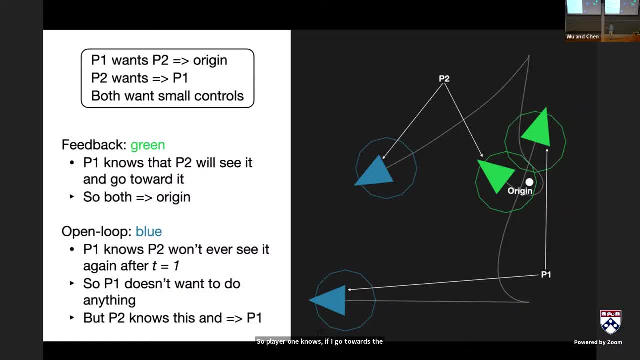 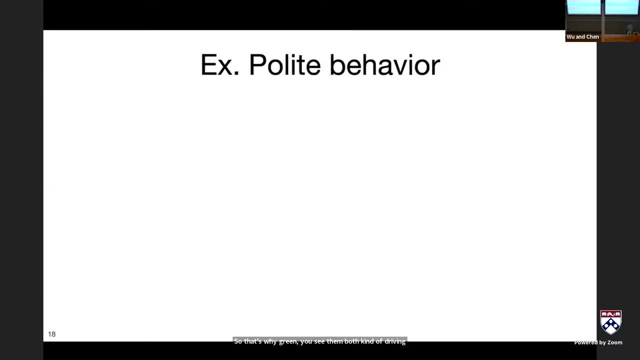 to get close to me and we'll both end up at the origin. So that's why the green, you see them both kind of driving towards the origin. Okay, so another example. um, let's say I'm working at a self-driving car company and I want to make my car be polite to others. How can I encode that kind of? 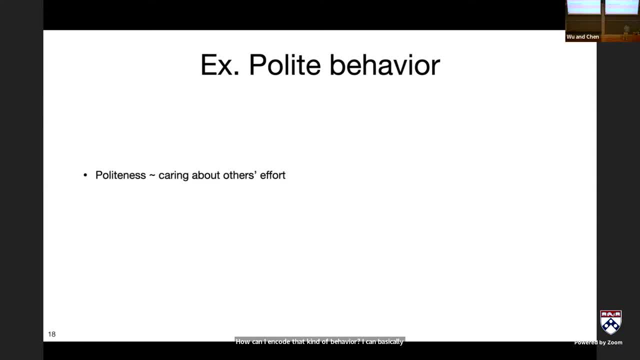 behavior. Well, I can basically penalize my car for other players control effort, right. so if they have to decelerate very quickly, they have to apply a large input, then I can penalize myself for that. So, like, maybe this is a dumb way to do it, I can take whatever cost I had this j1 tilde. 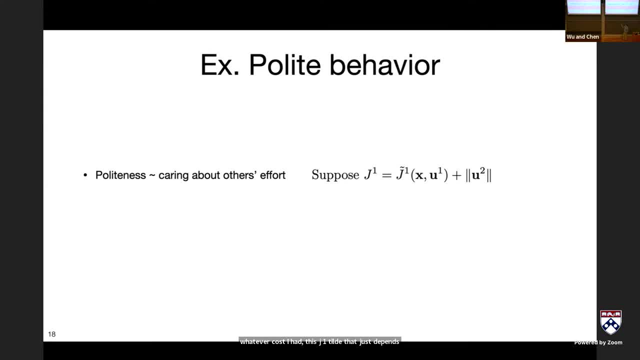 that just depends on my input and the state, and I can add, you know, some norm of player two's input In open loop. this is not going to influence the equilibrium at all, and here's why All you need to do is write down the optimality condition for player one. so I basically write down that. 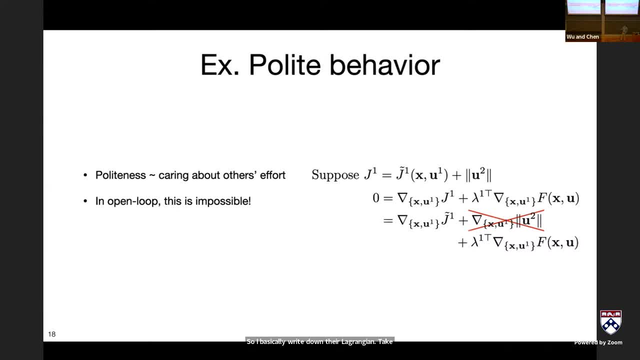 they're Lagrangian- take its gradient with respect to their primal variables. and I see that this term- you know basically the norm of player two's input- has no dependence on either the state or player one's action in open loop, so that derivative is zero and it disappears. so that's why, basically, 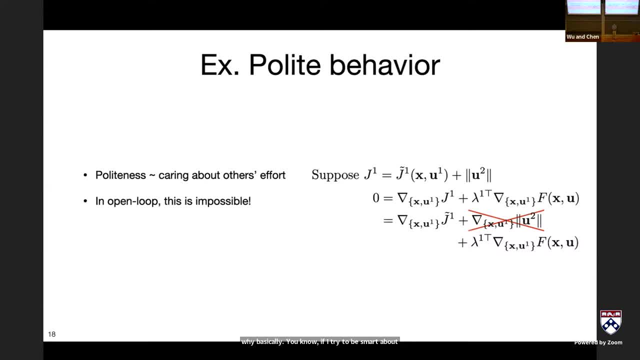 you know, if I try to be smart about encoding a lightness this way, it's just not going to work. so I have to be more clever in feedback, though that derivative will not disappear, because what's going to happen is that player two's action in the future is going to have to be more clever. 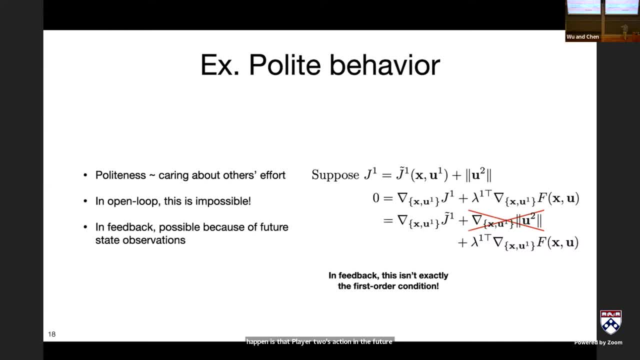 depends on the state in the future which depends on player one's action now. So that derivative with respect to player one's action now is non-zero. Okay, So all this is basically pointing to the fact that the structure of information available to the players 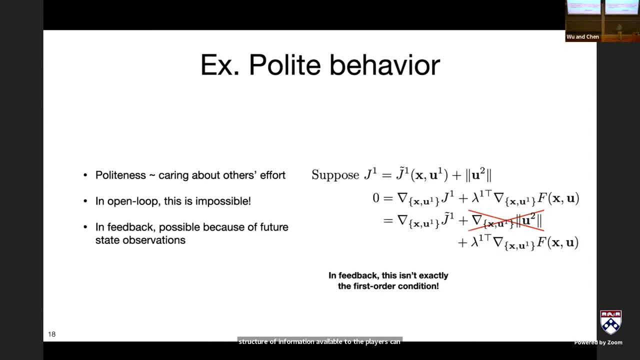 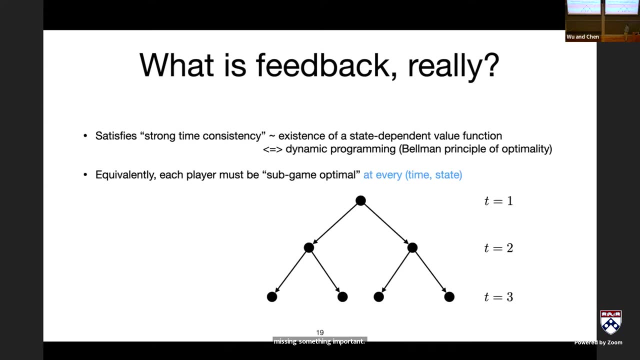 can really influence the equilibrium, And if you naively just follow your nose and write down the KKT conditions and go for it with whatever algorithm you like, you could be missing something important. So what is feedback actually doing? Let's be a bit more careful. 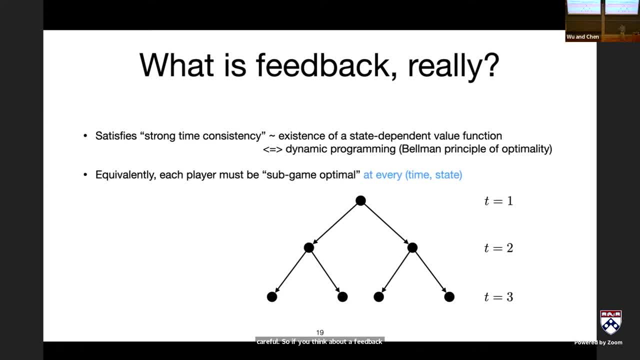 So if you think about a feedback equilibrium of a problem, it could be an optimal control problem, a game regardless. you are basically saying that you need to satisfy a time consistency property, a strong time consistency property, which I think is best understood as just the existence. 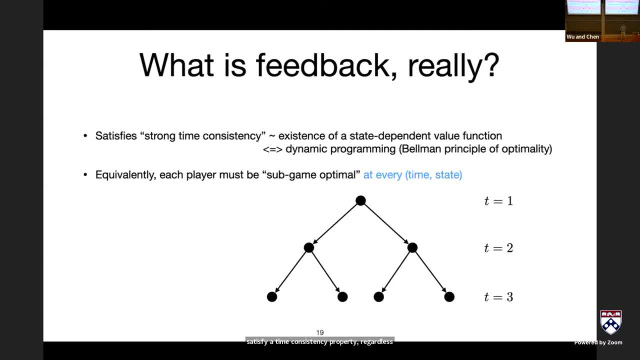 of a dynamic programming solution. So if you write down like a kind of an extensive form of a game or just a tree, what this is saying is you need to be able to work your way backward from the bottom to the top and constructs players, optimal strategies. 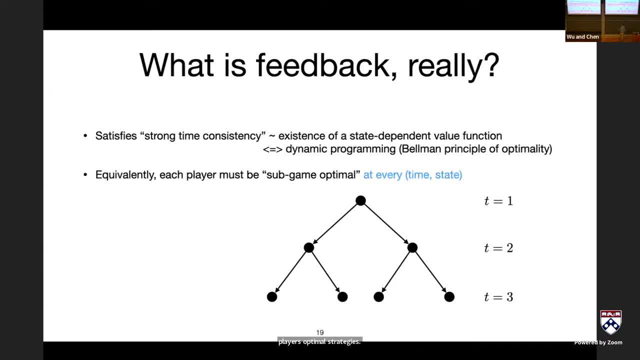 or equilibrium strategies. that way, And if you do it that way, you'll automatically be satisfying whatever feedback conditions you require. There's another way to understand all this, though, which is also, I think, pretty useful, which is in terms of what's called information sets. 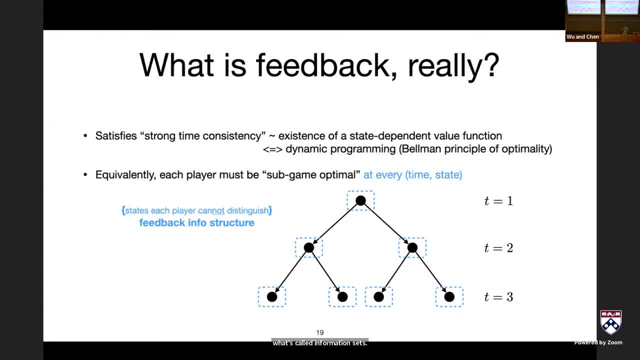 So if you look at a kind of textbook on this, what they'll often do is they'll augment the kind of tree structure this way and start adding sets that look like this, And the idea here is that every boxed state or set of states, 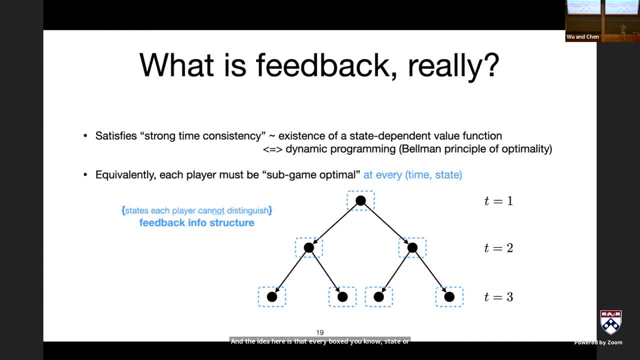 is just the set of states. it is a set of states which a particular player cannot distinguish them up. So, in particular, a feedback information structure is one that looks like this, where the players can distinguish exactly what the state is at every time. 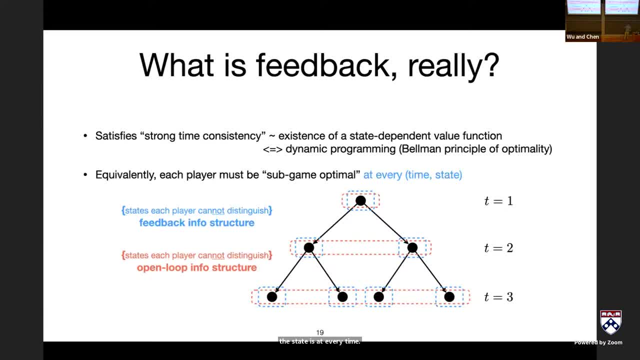 Okay, an open loop information structure would be this one, which is to say, at time one, both players know what state it is, but at time two, they have no idea what state it is. All they know is what time it is. 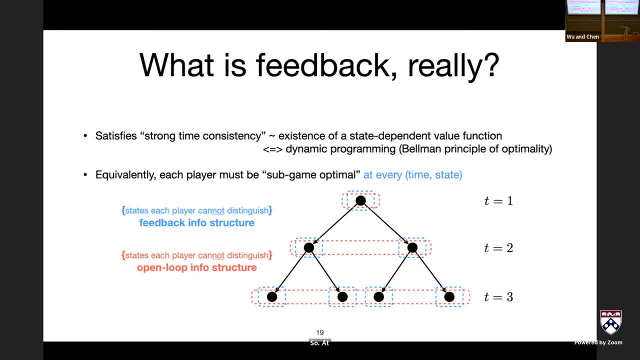 So at time two you see that the red box includes both possible states, which is saying that the players can't tell which one they're in. They can't distinguish among the states in that box. Okay, so sometimes that's useful to imagine. 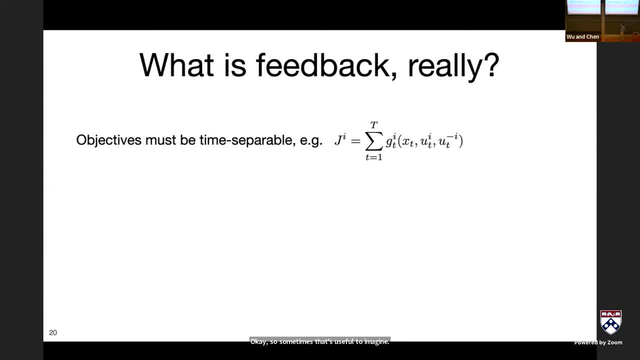 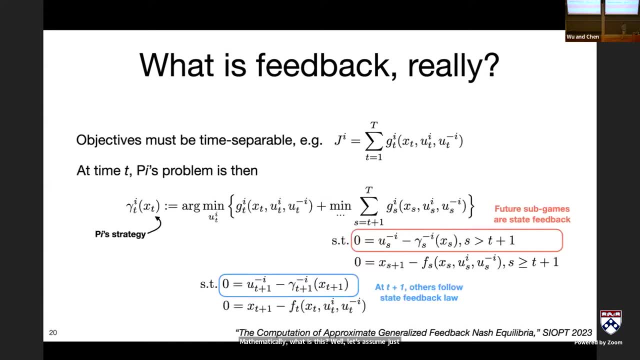 Mathematically. what is this? Well, let's assume, just for the sake of argument, that player's objectives are, you know, sums of other functions over time. I can then kind of just transcribe that exact condition of strong time consistency this way: 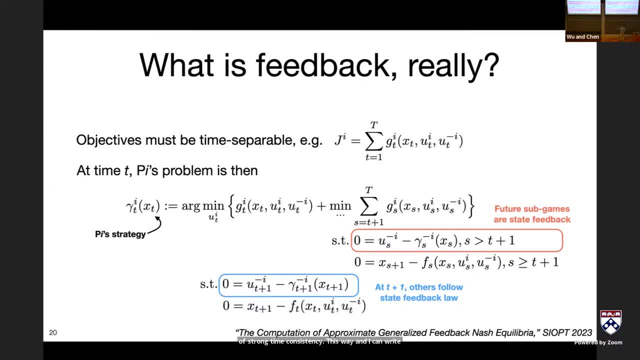 And I can write down at some arbitrary time, little t player i's strategy as a function of the state at time t And I can write it just. this is gonna look very familiar. This is essentially me just unrolling like a Bellman. 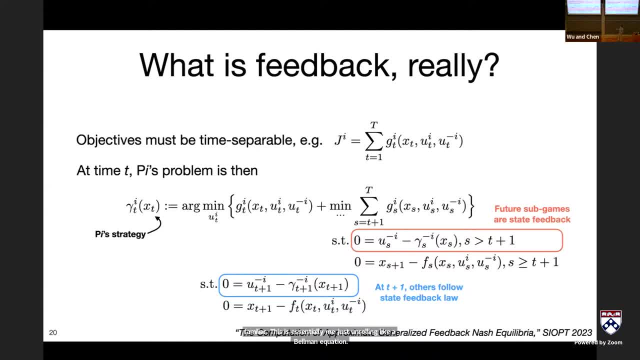 equation And I can say: well, it's the cost that I accrue right now plus the optimal cost to go in the future for each of these sub problems. So right now and in the future we have to satisfy dynamics of the game, satisfy the rules. 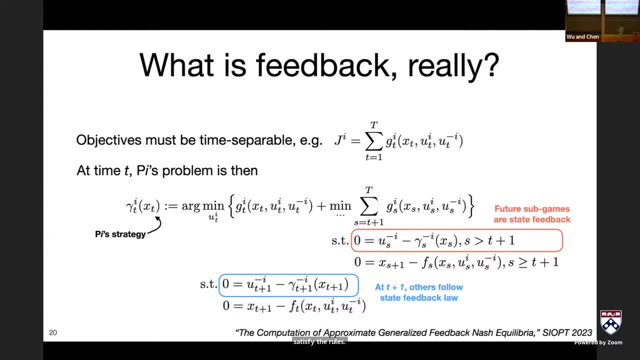 But crucially in the future I have to be also satisfying these kind of like I have to be choosing actions according to these optimal strategies, Like I can't just choose any action I like, And so these box constraints, these are very important. 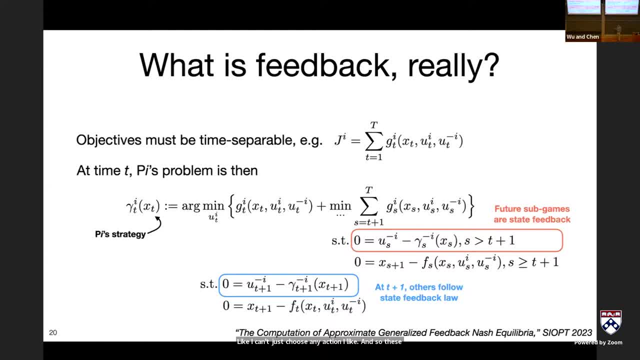 These are the things that encode feedback equilibrium structure, right? So in other words, actually what happens is, if I remove those box constraints, everything will collapse and we'll get back to exactly the problem I was saying, Where you can stack up the KKT conditions. 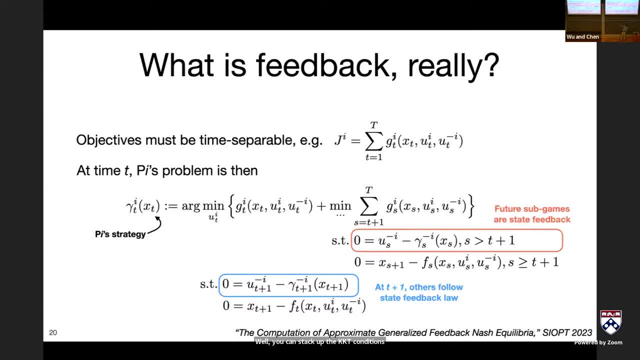 and find a root and everything will be fine. So if you remove those box constraints, there is a Display function that alters single comments. So if you remove those box constraints and other commands, every you'll be fine. So if you remove those box constraints and other, 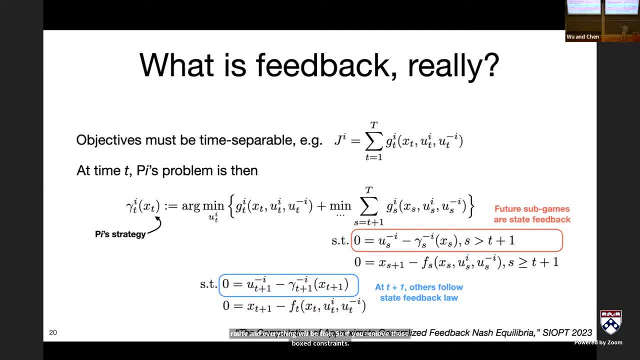 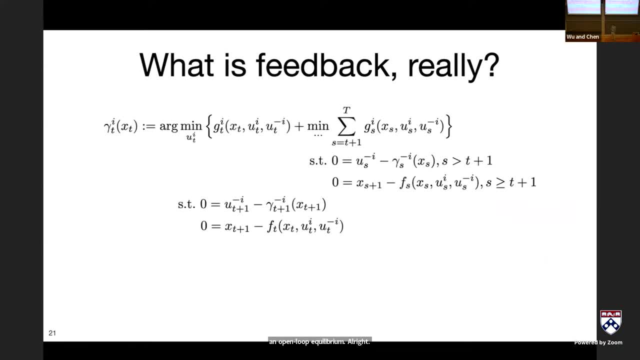 constraints, we get back where we were before and we'll get back to an open loop, equilibrium. So right, this is where we were. What's happening? I'm saying that the thing on the left, this is player i's strategy at time t as a function of the state at time t. I'm saying that well. 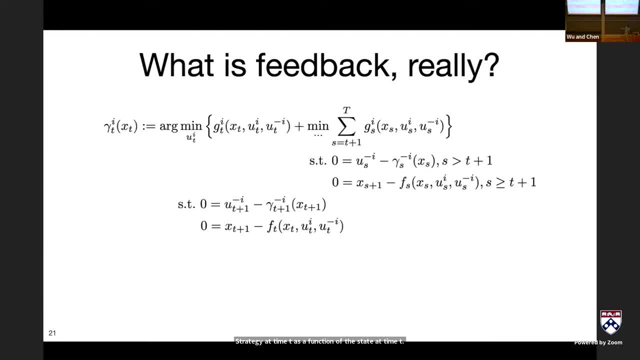 this itself. this is a function. It's implicitly defined to be the solution map of an optimization problem And it's recursively defined. So that means that there's a lot of nesting going on, And it's no surprise, because I was drawing out this tree earlier. So there's a lot of 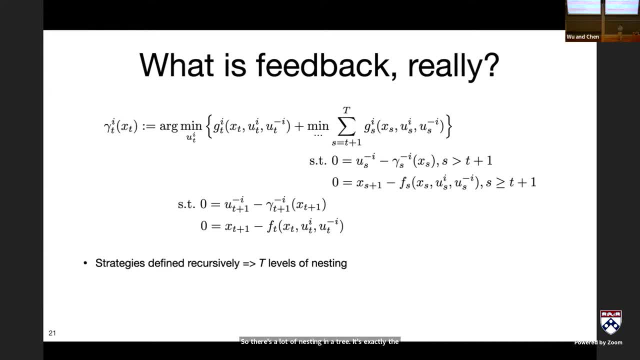 nesting in a tree. It's exactly the same, And so if there's capital T time steps to this problem, you can look in the top of the sum. then there's that many levels of nesting And at each level there's nt. 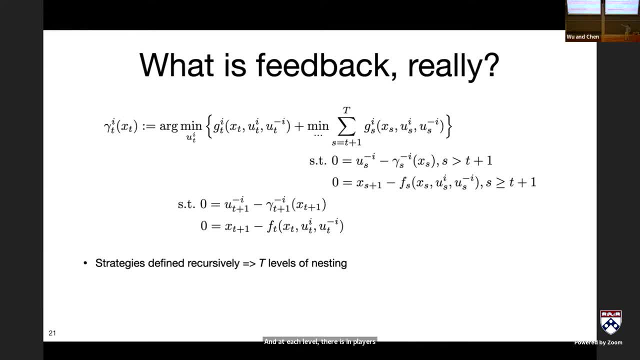 players And they're all coupled together. That's what's happening here. So I'm saying the action for any player other than i must be equal to the output of its strategy. All right, And so think back to writing down KKT conditions for this problem, If you're. 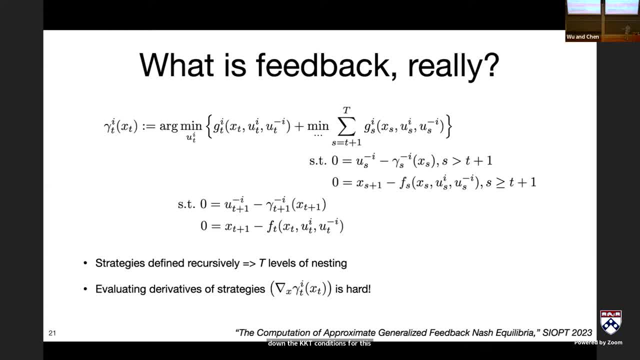 going to write down the KKT conditions for this ridiculously nested problem. it's going to get gross very fast, Because what you're going to need to do is encode derivatives of all the constraints with respect to the primal variables. So when you write out, transcribe this, you're going to need to write down a Lagrangian. That's. 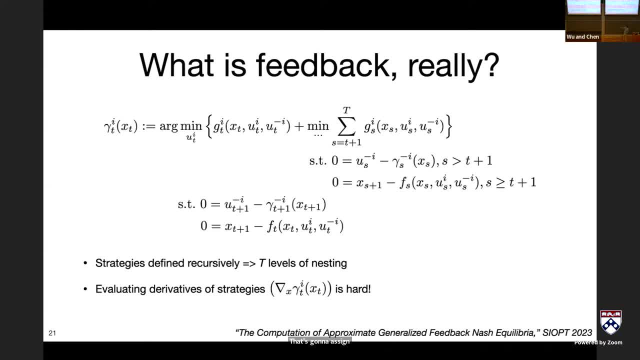 going to assign multipliers to all the constraints, And then you're going to take the radiance of the Lagrangian with respect to the primals. So you're going to end up needing those kinds of derivatives, But they in turn they're recursively defined. So to evaluate this derivative you need the. 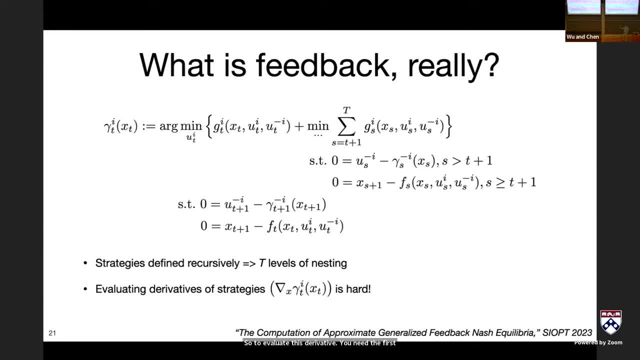 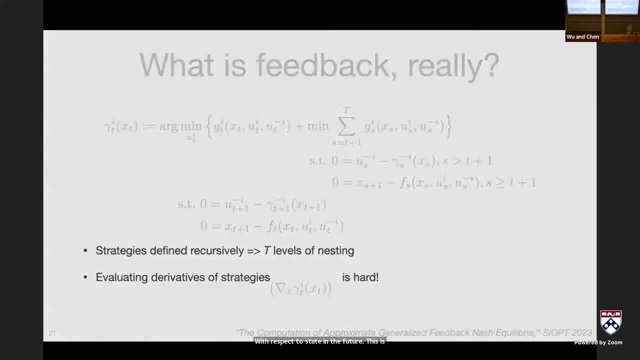 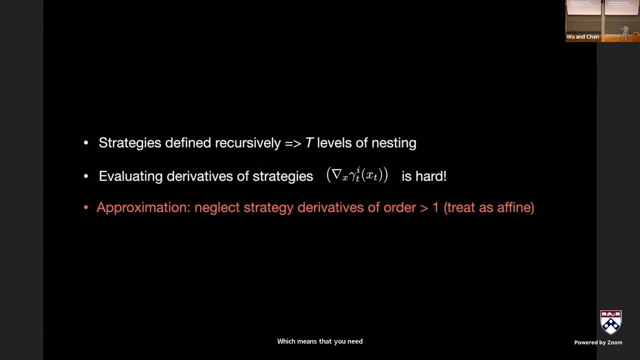 first derivative of a strategy for all the players in the future with respect to state in the future. This is all nesting in a very gross way, Which means that you need T orders of derivatives to do this write, Which is going to get horrible. 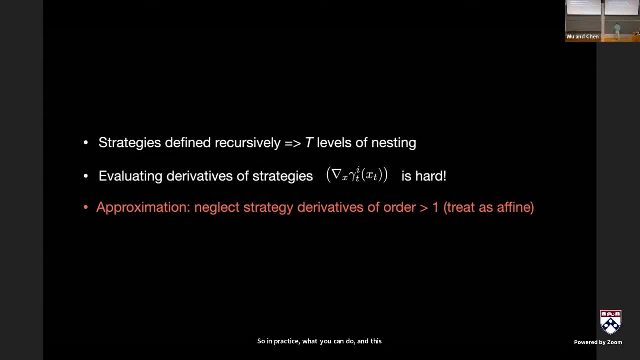 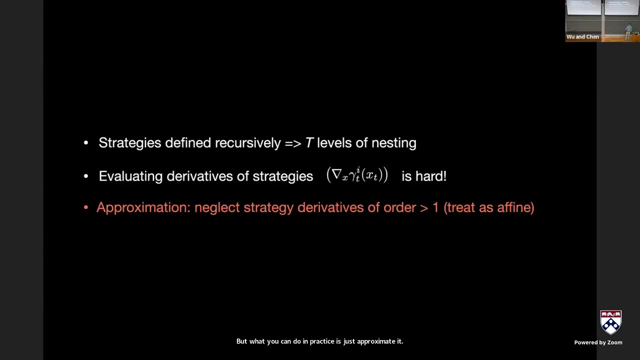 So, in practice, what you can do- and this is- it's taken us a while to get here, But approximate it- Just pretend that all the players are going to have to follow affine strategies And if you do this, all the high-order gradients, information disappears And what's. 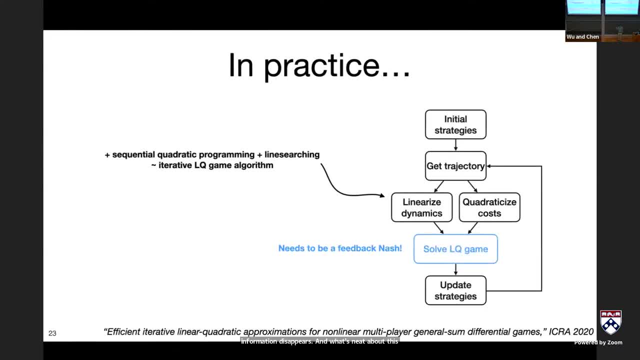 neat about this is if you follow your nose and write it all down carefully, this algorithmically looks a lot like sequential quadratic programming which, if you've taken your optimization class this is like a classic way to solve any equality-constrained optimization problem, convex or otherwise. 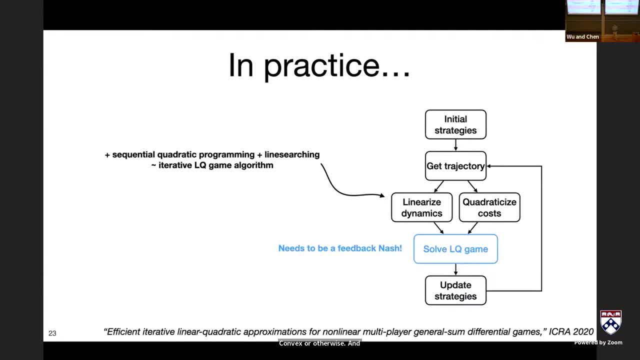 And arrive at a local solution. There's all kinds of great literature to you know. ensure that you are always finding the sent directions towards local solutions. I mentioned blind search and trust region methods. Those are some of the classics You can also handle. 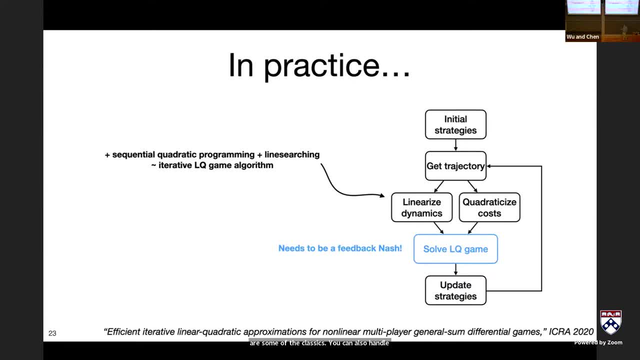 inequality constraints. There's all kinds of good methods for this. So we were very excited to realize that basically making that exact approximation gives you something essentially sequential quadratic programming for these feedback problems. And the other cool thing is that when you kind of write down the kind of algorithm, 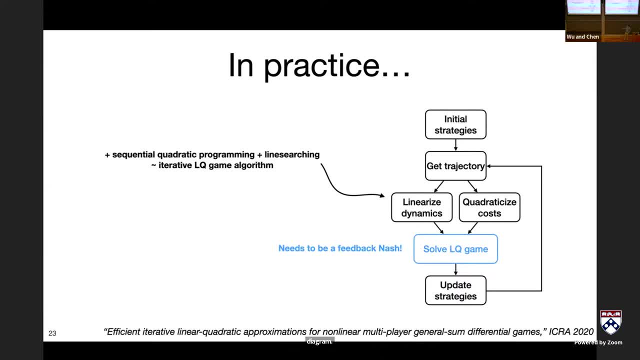 block diagram. everything is very easy to do And it all relies on being able to solve a linear, quadratic version of the game- linear dynamics and quadratic objectives- And that happens to be something we've known how to do since the earliest reference I know of. 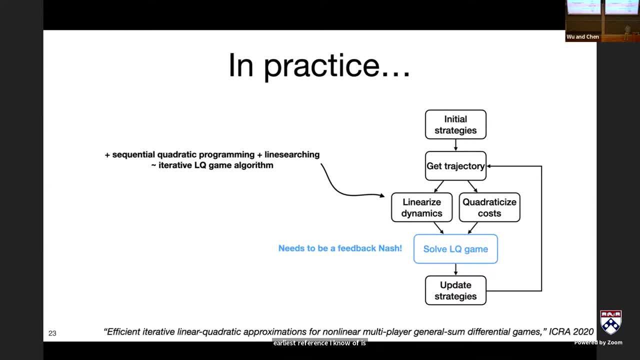 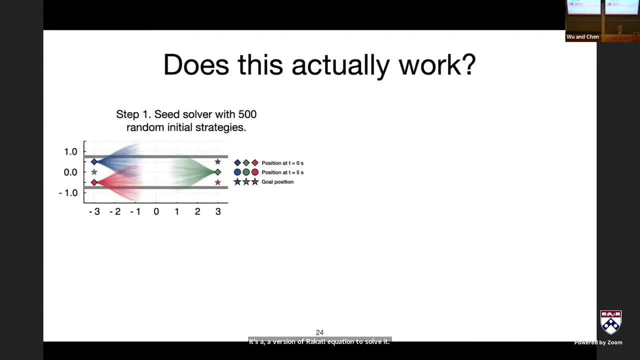 is 1969. that solves that problem. It's a version of a Ricotti equation to solve it. Okay, So it's very fast to solve And it actually works. So you can do this. This is just like a quick Monte Carlo study that we ran very early to just see how well it worked. So you 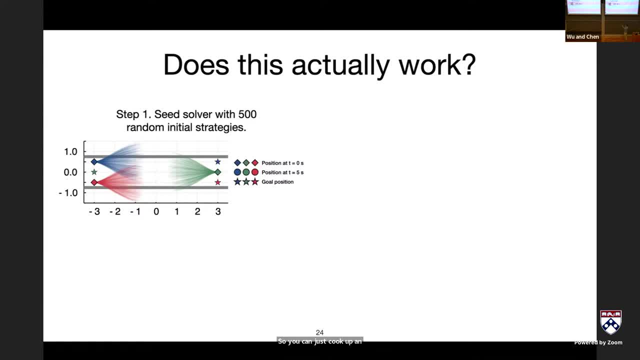 can just cook up an example. This is a three-player game. Everybody's trying to cross a crowded hallway without getting too close to each other, And what we did is just started from 500 random initial strategies for all the players And for each of those 500 things. 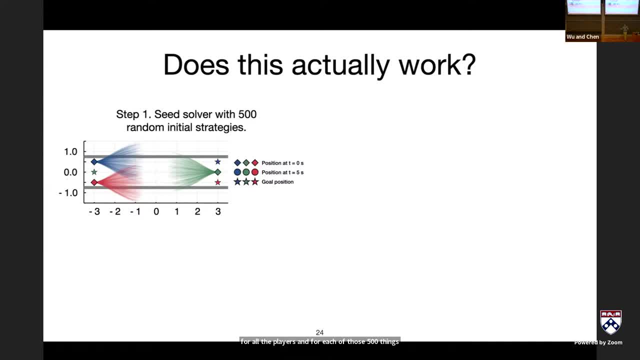 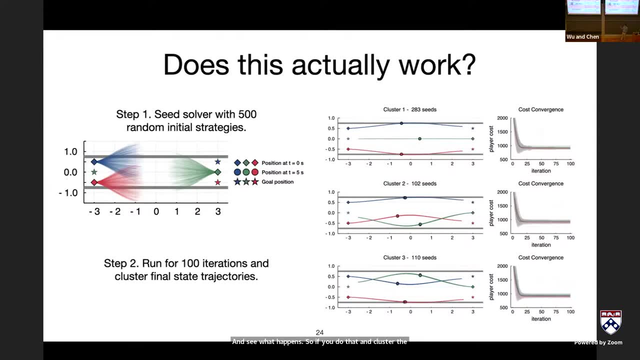 just run the solver for 100 steps, Okay, And see what happens. So if you do that and cluster the results- just kind of k-means kind of thing- you immediately see three clusters, And so here I'm just showing you the trajectories in each cluster and the corresponding like convergence of every run. 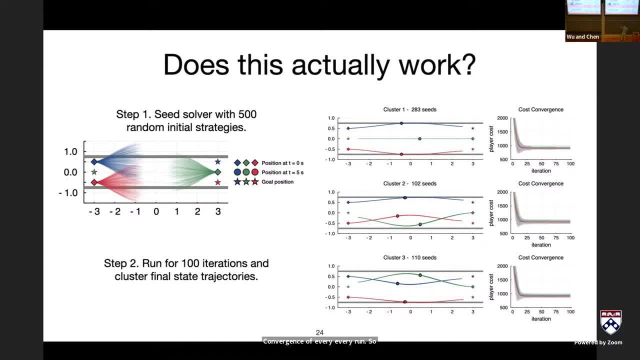 So convergence is very reliable. The clusters, each equilibrium. it seems to be three equilibria of the problem And they're encoding extremely intuitive behavior. In the first one you can see that the players are. you know, outer players are kind of hugging the wall and 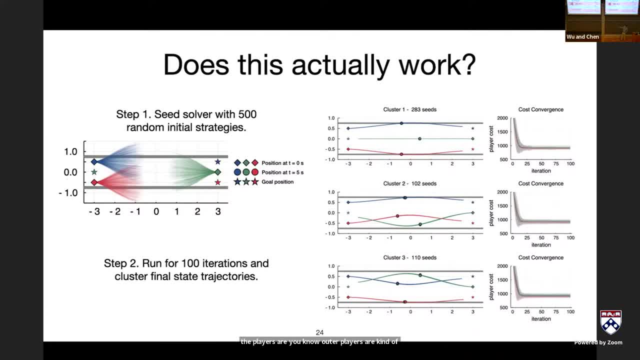 letting the middle guys sneak through And in the others they're mirror images of each other, where middle interchanges place with one of the top or the bottom. So this was encouraging, Also kind of one of the most fun things I got to do near the end of my. 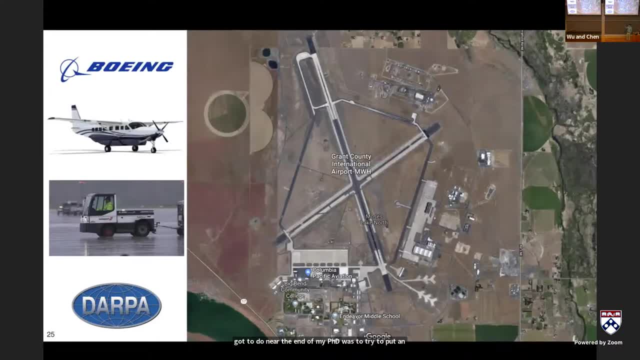 PhD was to try to like put an early version of this algorithm on a test aircraft just to taxi around an airport, avoiding runway intruders and things like this. So we posed all this And so this is kind of the end player trajectory games and solve them easily, real time And 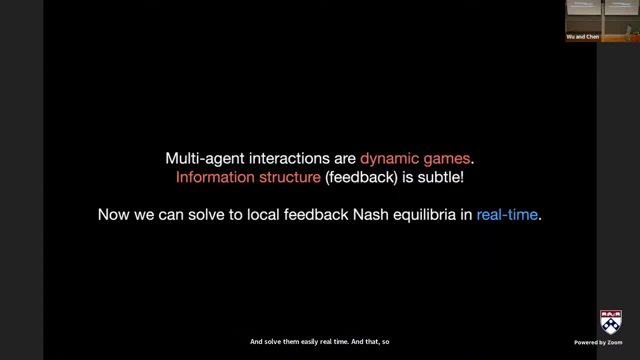 that's so anyway. kind of watching that happen was super fun. Okay, So where do we get? Multi-agent interactions are very natural to write down as dynamic games, but the information structure that describes those interactions is very subtle and it arises in these weird ways in 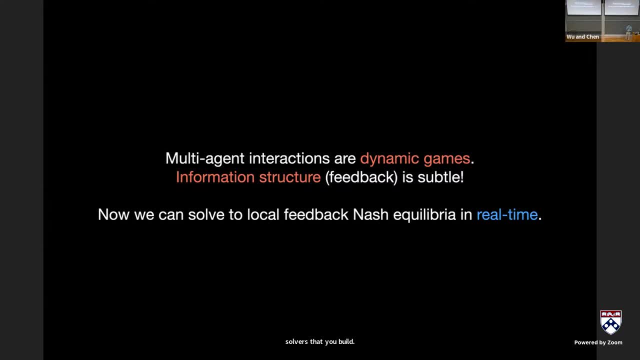 the solvers that you build. So if you build a naive solver, you can end up solving for the wrong equilibrium And, as we saw in that, that example of like driving towards the origin, they can be wildly different. You can have wildly different equilibrium. 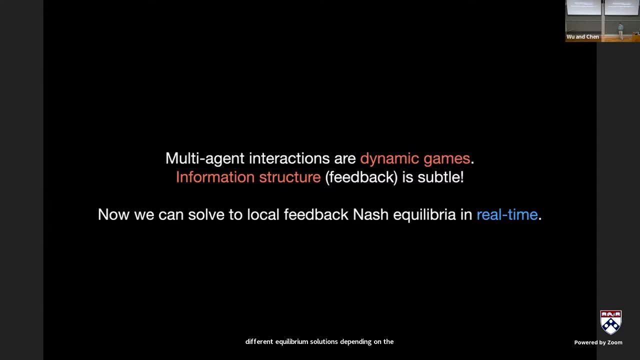 solutions depending on the information available to the players And if you, you know, choose a solver that goes for the wrong solution, I don't care how fast you run it. You know you can run this in a receding horizon loop as fast as you like, it's always going to. 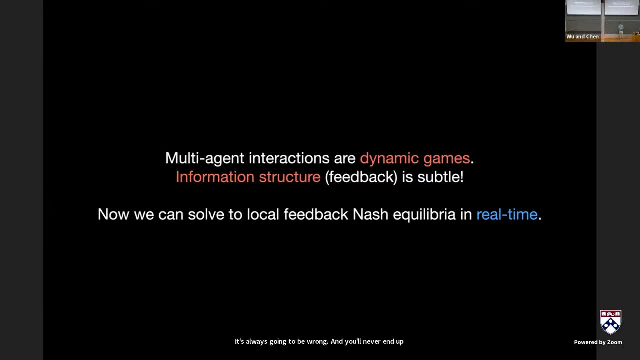 be wrong and you'll never end up going the correct direction. So so that's, I'd say, like the, the major message here. If you know what, what information is available to each player, even if it's got this nested structure to it, there are nice approximations that we show you can make that allow for real. 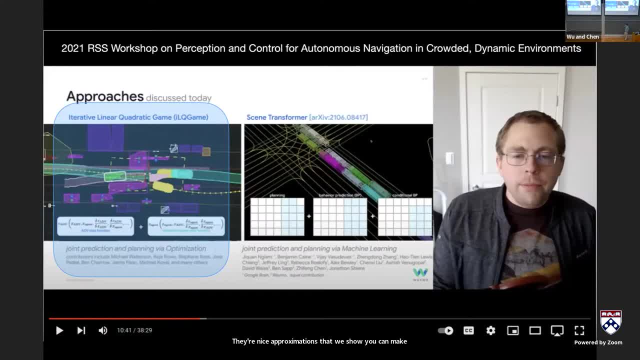 time computation. Okay, And I was. I was kind of talking about an early version of this work back in like 2021 at an RSS workshop And it was. it was kind of especially neat to see that the the speaker right before me is from Waymo and they were actually trying. 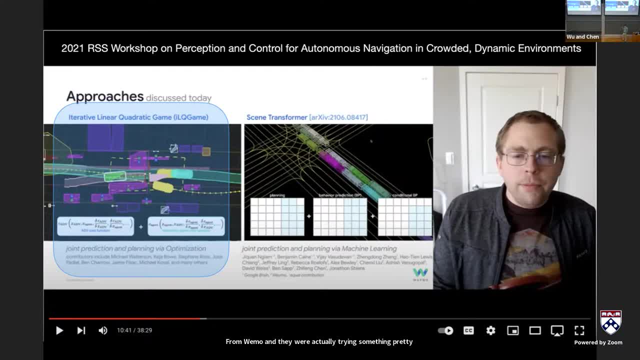 something pretty similar on their car. So I guess the point I'm trying to make is just that These ideas of modeling interactions among drivers on the road- it's something that people in the industry care about too, And you know they had done their own version- I actually 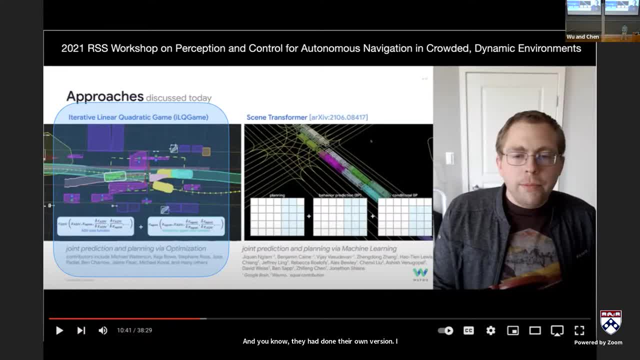 I happen to know a little bit more detail about it, that I can answer some questions offline maybe, But but there were some some subtle differences between what they ended up trying and what I just showed you. anyway, All right, So I think we've got just enough. 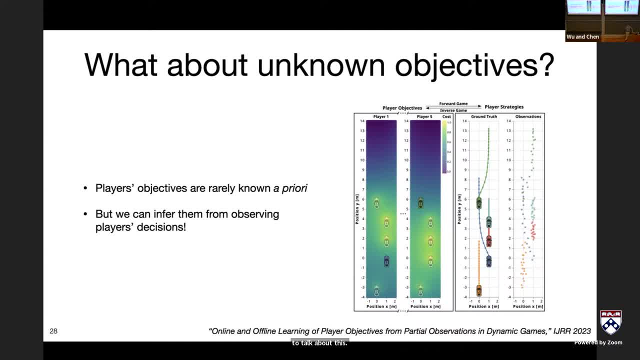 time to talk about this, So I want to. I think we've got just enough time to talk about this, So I want to. I want to, now that we understand a bit more about what these games are, what they look like, and 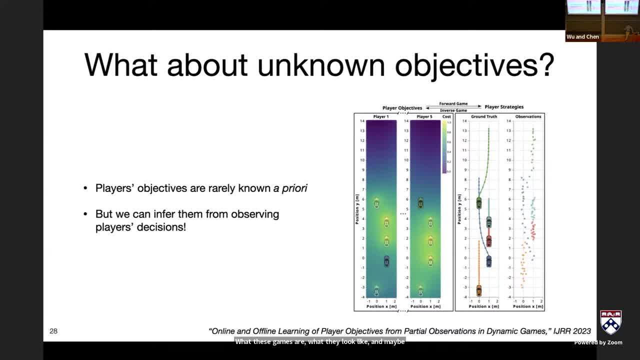 maybe some of the kind of key ideas in solving them fast. Let me pick on the kind of the dual problem, the inverse problem. So everything we just talked about assumes that you know all the players know everything about one another's objectives. That seems kind of unreasonable. 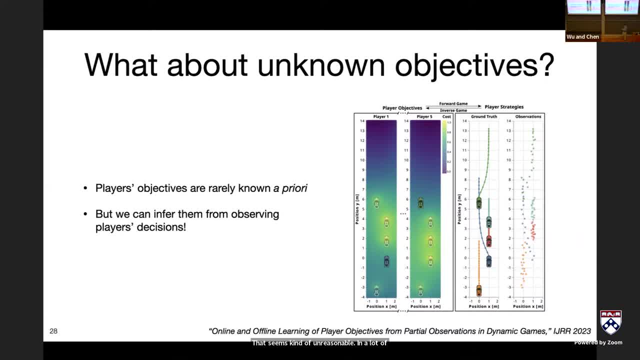 in a lot of circumstances, Like if I'm driving on the road, how do I know exactly what lane change somebody else wants to make? Or you know how distracted they are and maybe they they are going to not even see another player because they're on their phone or whatever. 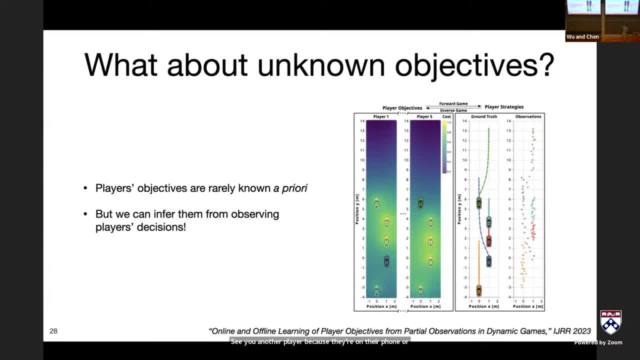 So so we thought about this problem, And some of the, I guess, work we've been doing in the last couple of years has been trying to show conditions under which you can infer those objectives from watching strategic play. So here's an example of five cars on the highway. 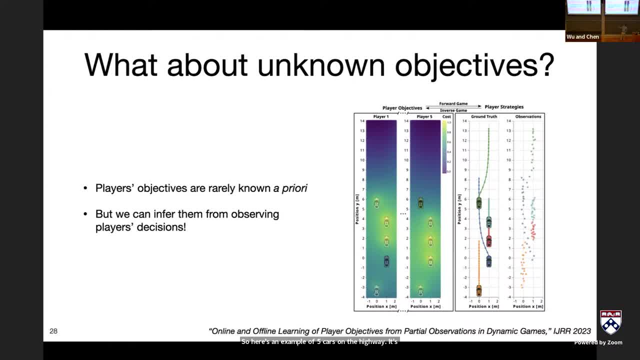 It's obviously simulated And we see the like. imagine, you see like a noisy measurements of all the cars position over time. for a few seconds, Can you back out all the way to the left? Like, what were the players? objectives, What were there? So here's a heat map of 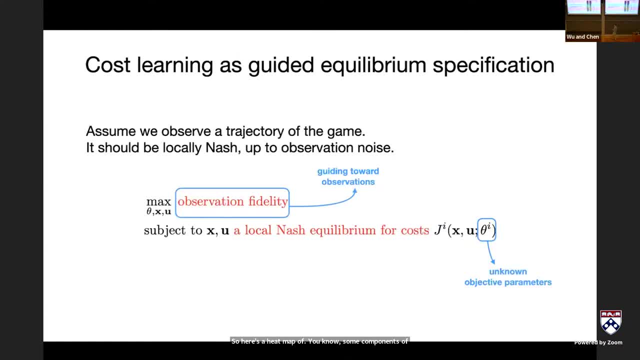 you know some components of their cost. So the way we've kind of developed to think about this problem is to think about it as an estimation problem. So there's some parameter of the objectives that we don't know and we would like to estimate from data. So you know the 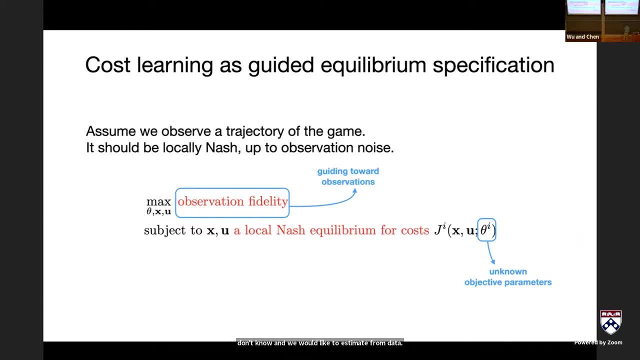 simplest starting point would be to think about just some kind of maximum likelihood. you know, map estimation problem, whatever you have, but but basically try to maximize the some measure of observation fidelity, subject to the constraints that correspond to equilibrium conditions. So basically, we know that these cars are behaving strategically. we know that. 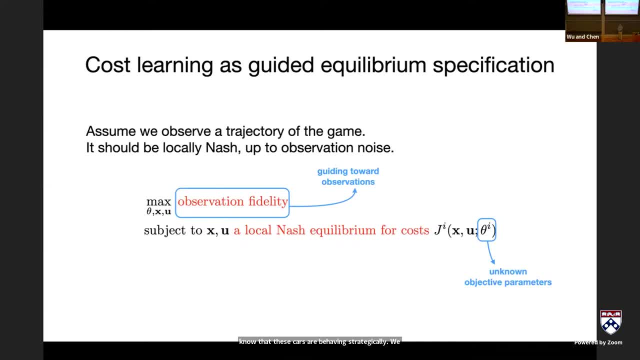 they are trying to optimize for something. we just don't know what it is. And how can we encode the fact that they are optimizing for something when we're inferring their objective? So so we basically just embed that as a constraints And if you transcribe, 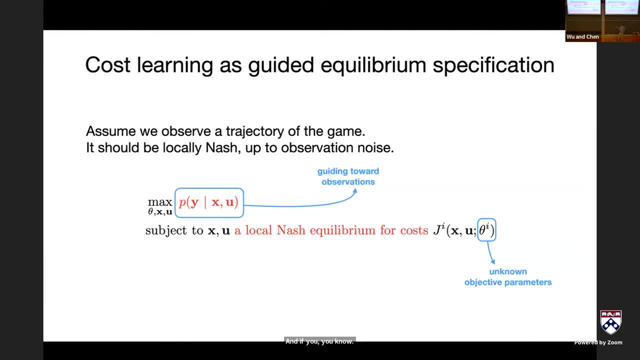 what are these things Actually? well, if it's a maximum likelihood problem, I want to have some kind of sensor model that allows me to establish the likelihood of a measurement from the vehicle state and maybe what they're doing. And we just showed how you can transcribe. 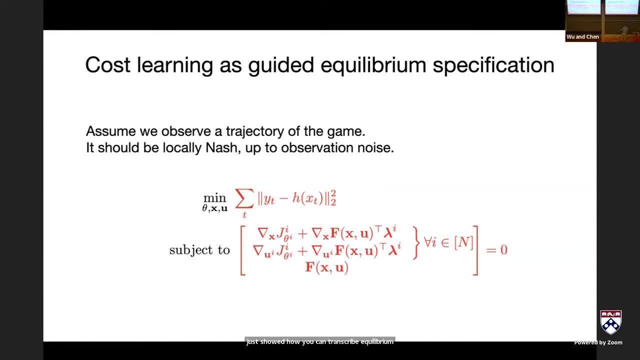 equilibrium conditions into equality constraints or maybe complementarity constraints in the constraint, in the, you know, more complicated situation. So so here those are the open loop KKT conditions for all the players, and you can just stick them right here. And if 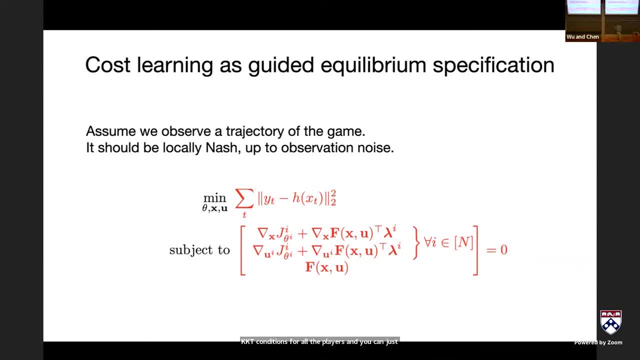 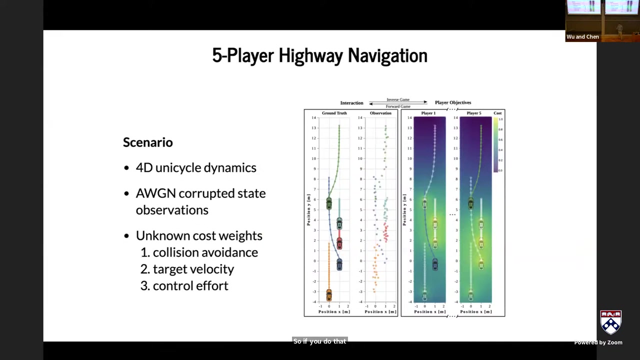 you do that, you end up with just a, you know, non linearly squares objective with these potentially wild, non convex equality constraints. Okay, But sure, you can still deploy your favorite root finding algorithm to to solve this problem. So if you do that, what? what happens? like, again, presuming the algorithms work appropriately. 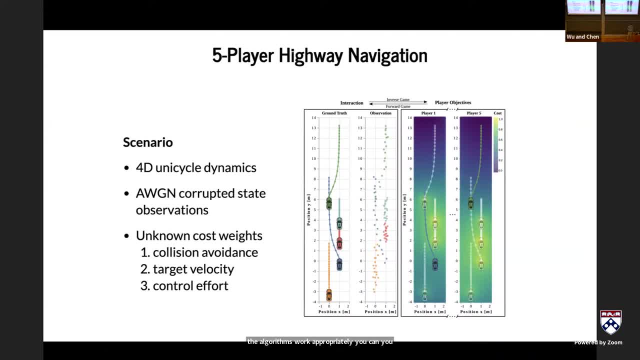 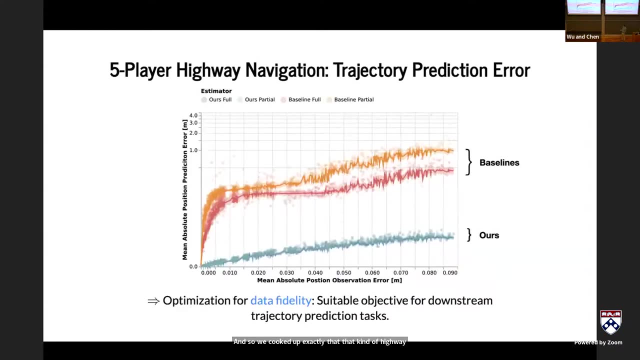 you can, you know, get them to converge reliably. Then we were interested in understanding what is this added structure of the strategic behavior assumption actually by you for estimation, And so we cooked up exactly that, that kind of highway. So we have this parallel. that is the driving example I showed you before, and and the punchline. 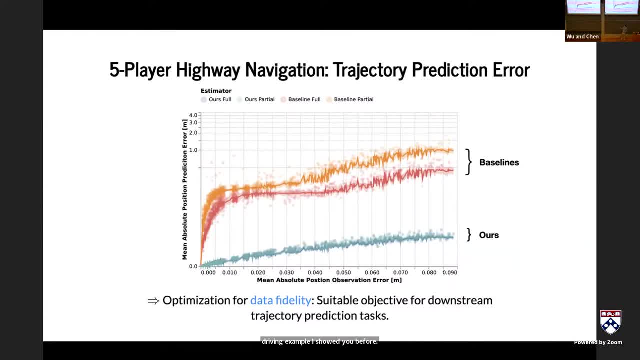 is that, if you like, don't really do much, don't really use this assumption to the players are strategically, you know, optimizing for these unknown objectives. you're very susceptible to noise, So that's what this plot is showing kind of the observation: noise is on the horizontal. 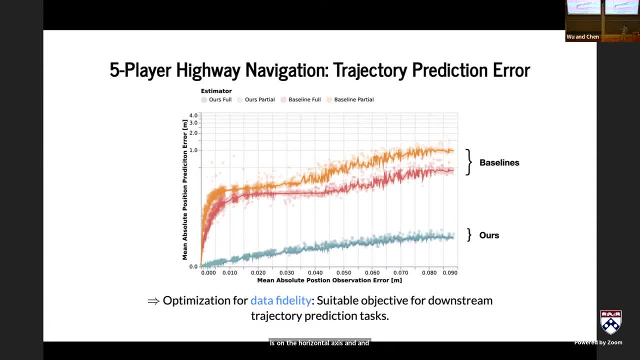 axis and and the kind of prediction accuracy, estimation accuracy, is on the vertical axis And you see that. you know it's a log scale And so the averaged is grinded down to even this one. Now, like I said, it's on the horizontal axis, But you can see that that's, it's not. 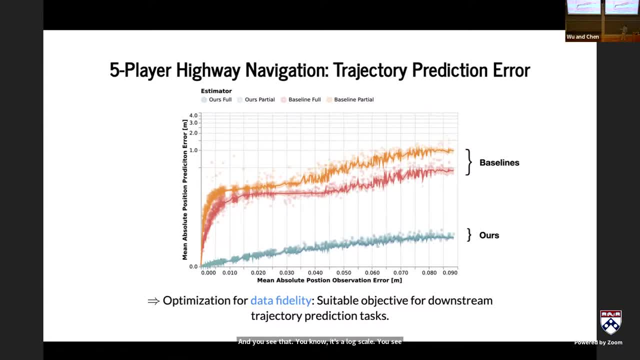 scale, you see that you quickly get separation between these existing methods that don't account for the game theoretic structure and the problem I just showed you. If you solve the problem I just showed you, even though it could be horribly non-convex- 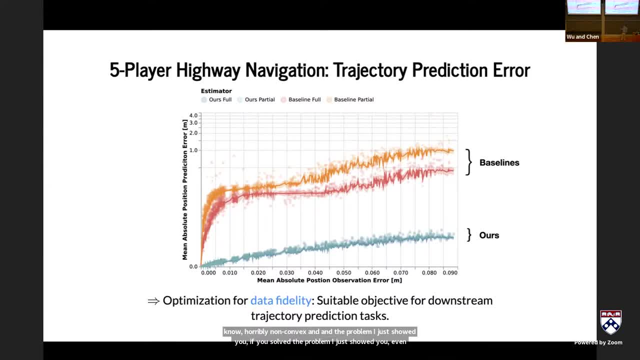 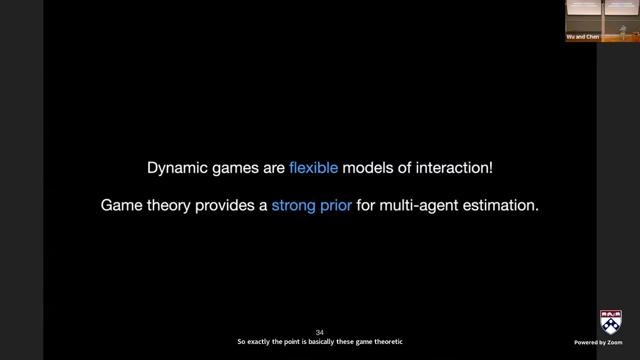 and you're finding a local solution. we'll basically squeeze more data, more juice, out of the data. Think of it almost like adding a prior. So exactly the point is basically, these game theoretic models can add nice prior information for estimation. I would say. 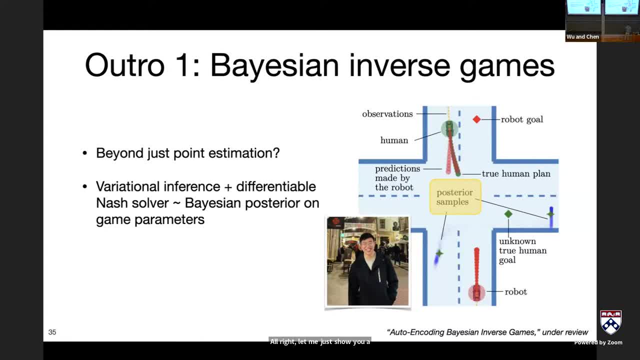 Let me just show you a couple other kind of quick outros before we close and take questions. So the thing I just showed you about maximum likelihood estimation, I think you know. the obvious question that I had for like a year or two after this work was, is there. 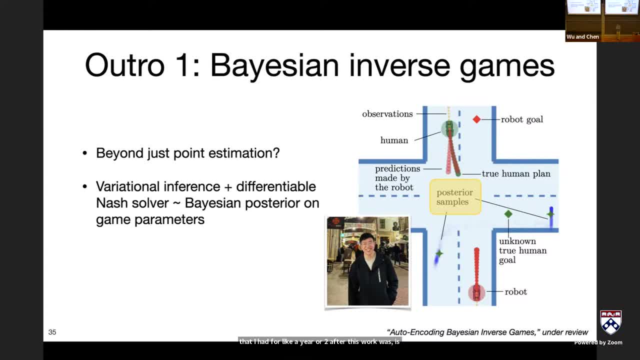 a better way to handle kind of distributional uncertainty Is there? like a Bayesian take on this. The short answer is: well, yes, you can do this, But what you have to do is be able to account for, you know, wildly non-Gaussian distributions. 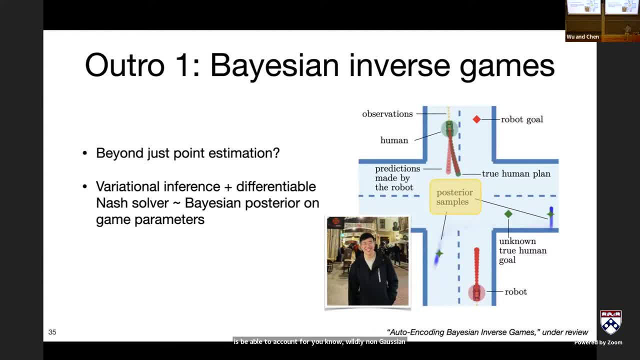 on the unknown game parameters. And to do that, fortunately you know, there are, you know, machine learning tools to do this right. We just basically coupled, like a variational inference technique that you know is super common in generative modeling, with a version of the game solver I just showed you. 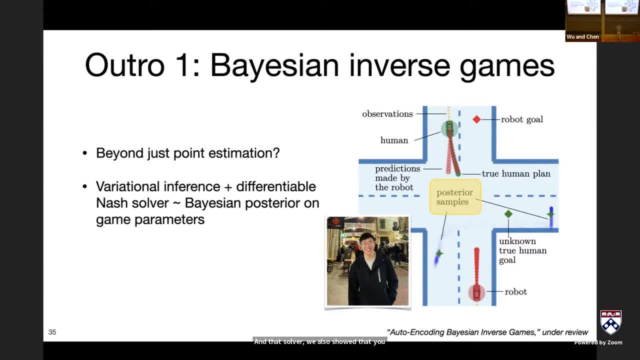 And that solver. we also showed that you can implicitly differentiate its solution with respect to the game parameters. And that was the kind of additional missing piece. And because you can do that, you're able to kind of stick it in as a layer in a neural 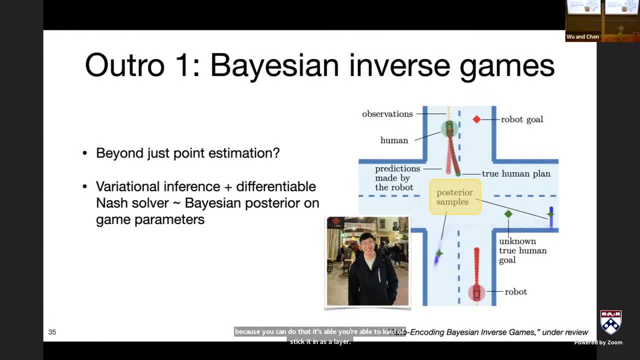 network and diff back through it, So kind of train the variational autoencoder with it. So the kind of short version of all of that is to say that here I'm showing you an example with an intersection, There's two vehicles and the unknown parameter of the objective is: what is the which points? 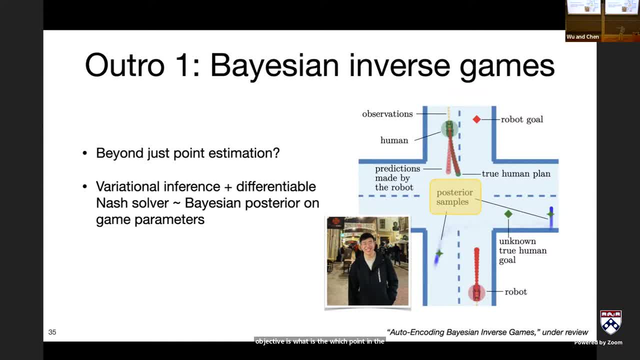 in the intersection is this player's desired goal position, And we basically allow that hidden parameter to just be a point in R2.. So it's continuous, And what the neural network has learned to encode is a distribution that you know basically says: OK, well, if they're in this configuration, I know that this car either wants to go somewhere, 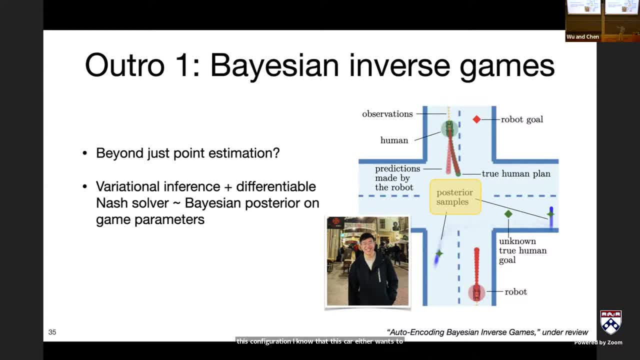 in this lane or somewhere in that lane. We do this from a bunch of data of watching people drive And then just show how you can couple a planer to it. So that's one thing you can do. Another thing that I think is kind of interesting is to say that 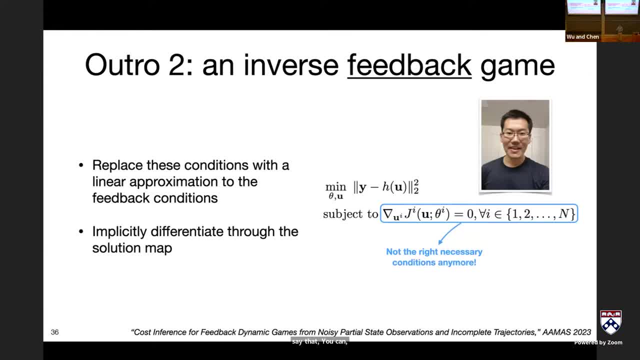 You can. so you know, most of the first part of the talk was showing you how to encode feedback structures. Well, you can also do that in inverse problems. So we showed how you can take that maximum likelihood problem and basically just erase the constraints and replace them with the much more complicated KKT conditions of the 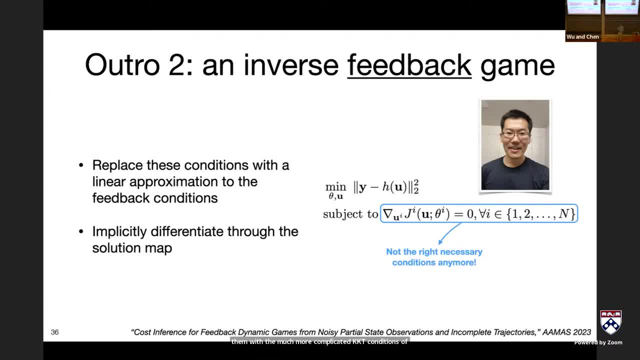 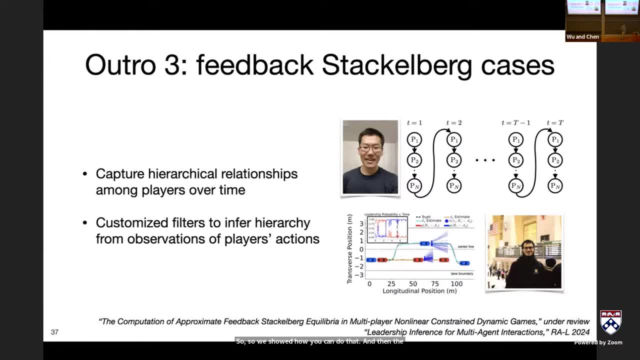 nested feedback problem and simplify them to a level where a solver can actually handle it. So so we showed how you can do that. And then the other last thing I want to mention is Is that all of today's discussion has been about Nash equilibria, either an open loop, 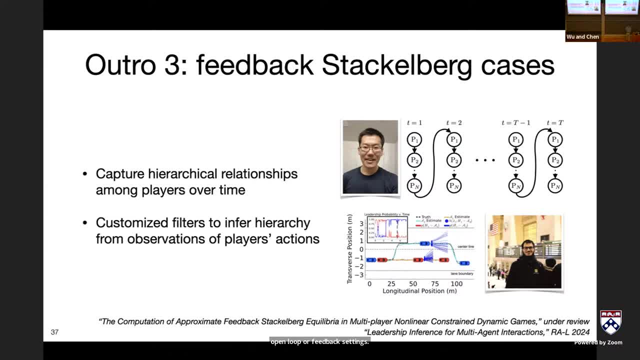 or feedback settings, But we can basically basically play the same games, Same tricks for solving Stackelberg problem. Stackelberg equilibrium concept is kind of encoding a hierarchy among the players. So here I'm showing you up here, just that player one influences. player two: who influences? 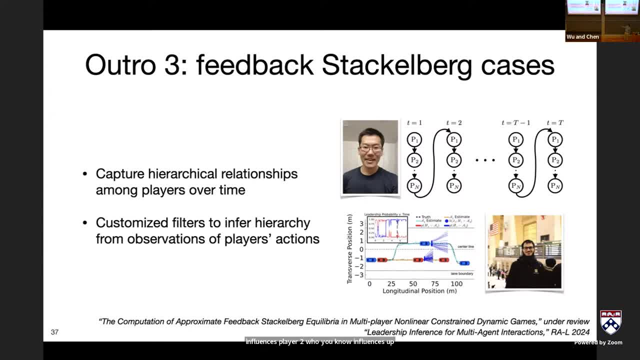 up the player and at time one and then at time two, it's the same thing. So there's an order of play And those kinds of problems are. you can immediately see that they're also nested and because you know there's still nested problems, we can start to play exactly the same tricks. 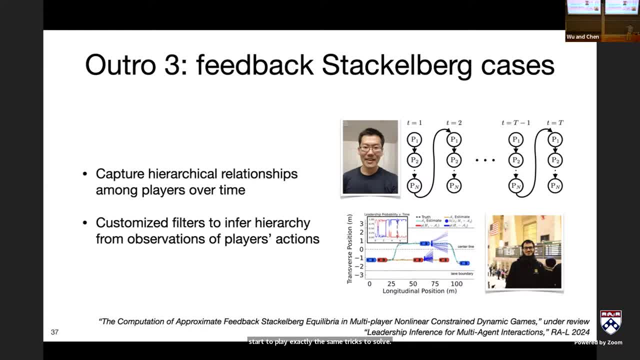 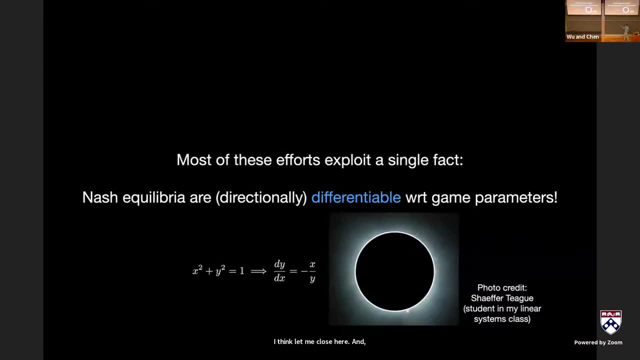 to solve, And you can even do inverse problems there. You can even try to infer what the hierarchy is among the players by watching them play, So so that that's also work we've been up to recently, I think. let me close here and just tell you like the the big punch line of that. 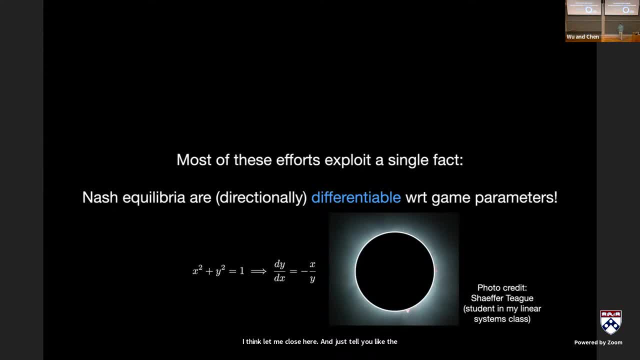 That last line of work. most of what we've said is just that a lot of the the algorithms here are enabled by the fact that equilibrium solutions of games are at least directionally differentiable with respect to their parameters. So, and, and you know, kind of goes back to high school calculus. 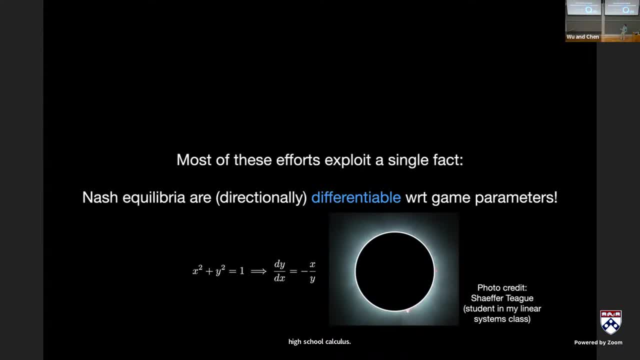 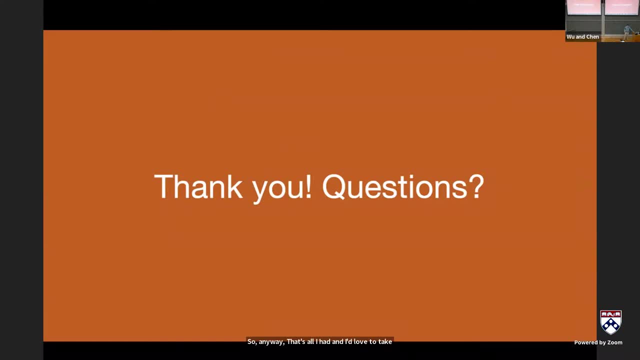 So, anyway, that's all I had And I'd love to take questions. Okay, Thank you for the talk. So question on the Stackelberg equilibria: How would you suggest we think about sort of these, formulating these like hierarchical? 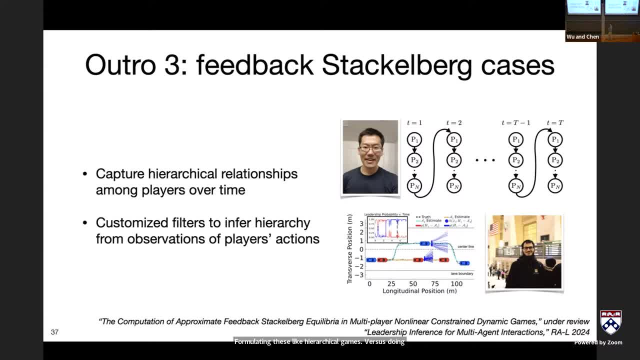 games versus doing something like a hierarchical reinforcement learning setup. Should we? are they fundamentally different problems Or should we think about them as different formulations? I guess- I guess I would go Back to you- is like: to me are they different problems? 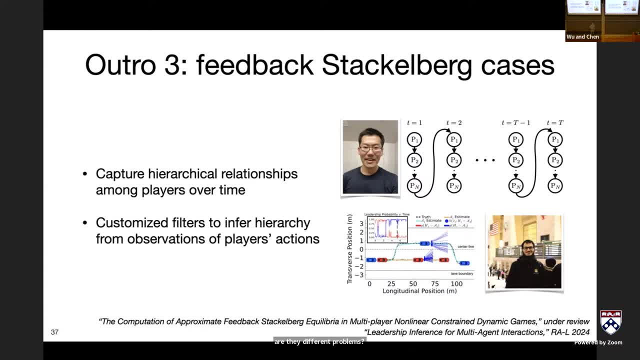 That's the first question And I guess I don't know exactly which you know hierarchical reinforcement, learning problems you're thinking of. But if they're the same problems, then I would say that you know they may have particularly different structures that make, or properties which make, different algorithms, more or less. 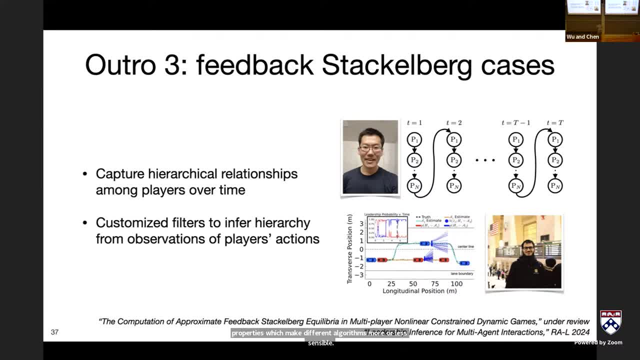 sensible. So, for example, everything I've showed you is has been a deterministic problem, whereas typically in reinforcement learning cases You're interested in stochastic dynamics and maybe stochastic policies. So if that's an important character of the difference, then if that's an important distinction. 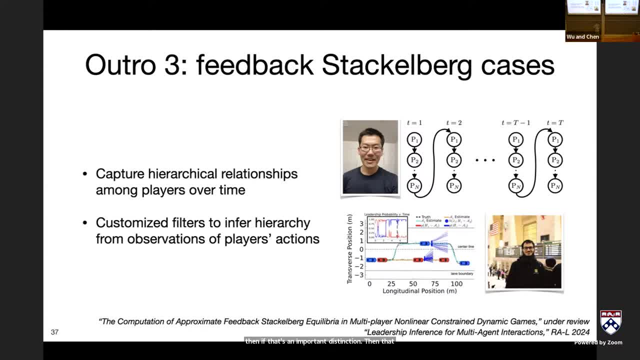 then that should have some impact on the algorithm you choose Or another. another thing would be: often in reinforcement learning, algorithms are designed so that they typically don't require like an analytic model of the dynamics or the constraints of the objective. Like if you talk to a reinforcement learning purist, I think they'll- they'll kind of want. 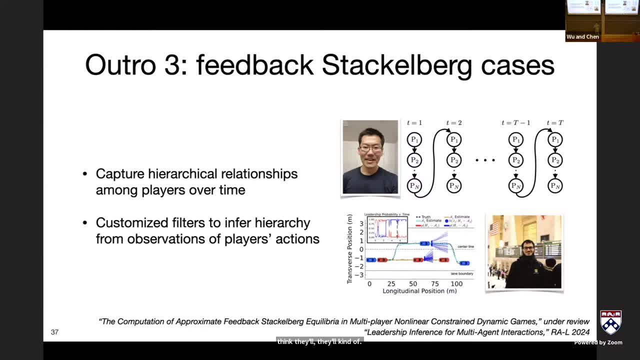 You to design an algorithm which doesn't require foreknowledge of those things, whereas everything I've showed you is basically been assuming. hey, yeah, I know exactly what the dynamics are and I can differentiate through them, I know exactly what the constraints are, et cetera. 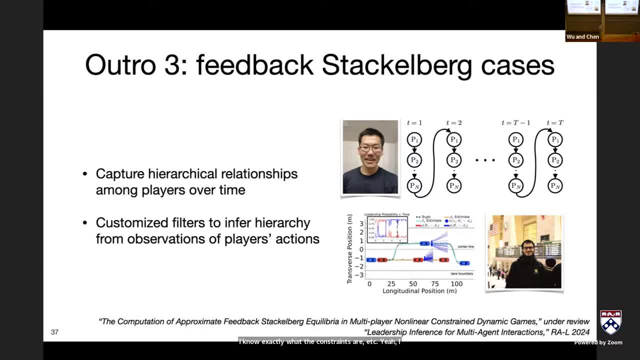 I don't know if that helps. but yeah, sorry, George, to build off of maybe the partial observability work, Your environments are all assumed to be static. if your environment were to start changing and you Not, and they not be agents that are changing? 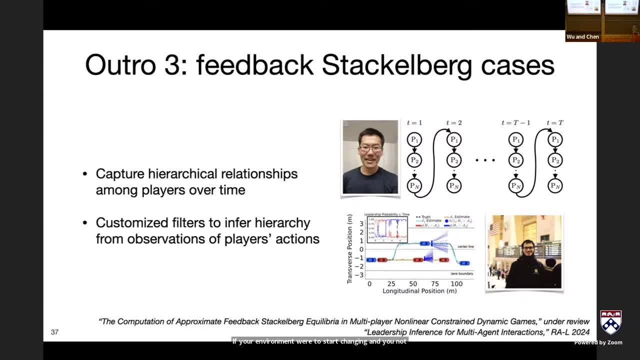 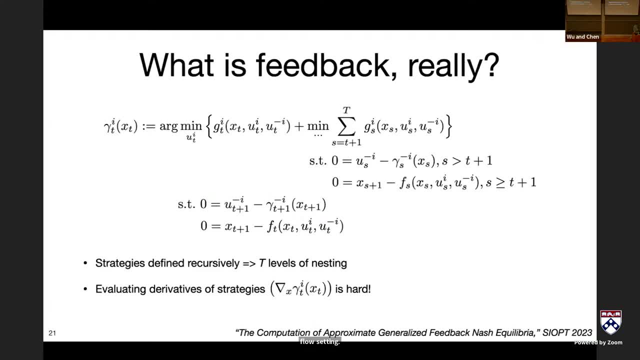 Yeah. so let's say you have boats and now you're in some type of flow setting. Does that feed into these dynamic game formulations? well, Is there a constraint there that maybe you didn't talk about, but that it could fall into it? naturally? 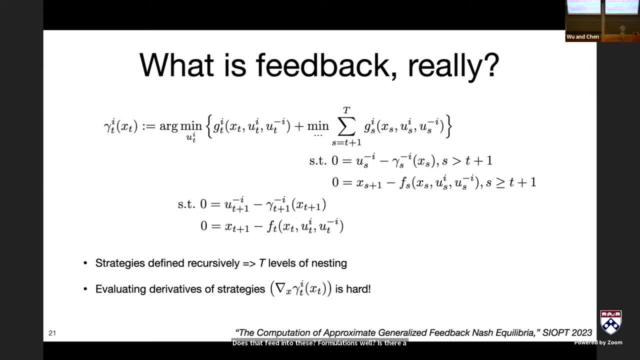 OK, sorry, I think what you're getting at is: do the can the dynamics of the game be time vary? Is that essentially what you're asking? Yeah, yeah, yeah, Yeah. So look up there All the F's. Those are the dynamics. 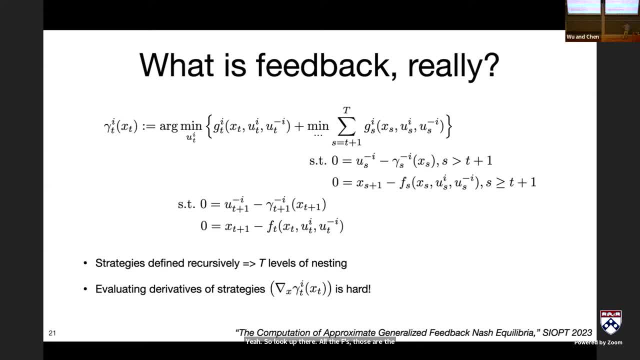 And I've subscripted them with time, So you can have whatever arbitrary time dependence you like. Yeah, I mean you have to know what it is, but but yeah, yeah, yeah, Thank you for the talk. first of all, just out of curiosity. so I was wondering whether 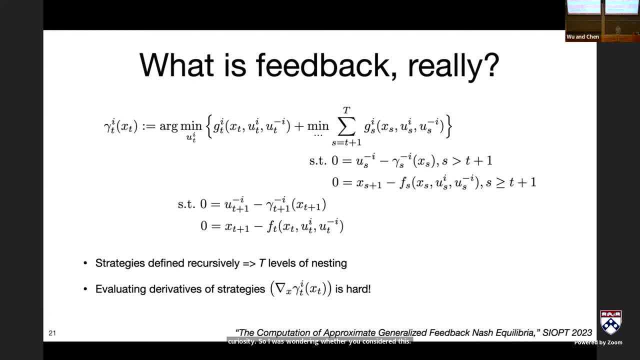 you considered this: corner cases where open loop, Open loop strategy can be a best response to a feedback strategy. Oh, that is a good question. So I can think of, for example, a couple of examples. let's say, let's say I'm a crazy. 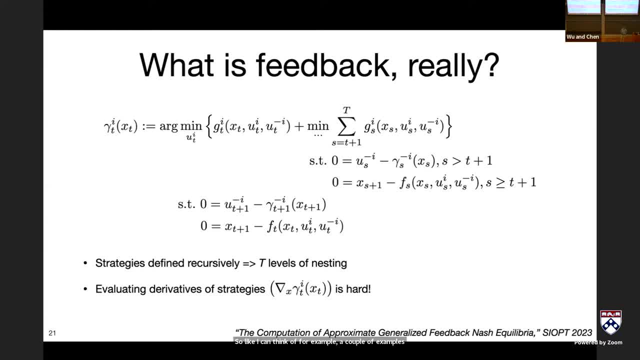 person and I just want to show I'm on the road, on highway, on a straight road, and I want to arrive at the destination as soon as possible. Yeah, And I say hey, my gas pedal got stuck, Yeah, And I pulled off my wheel. 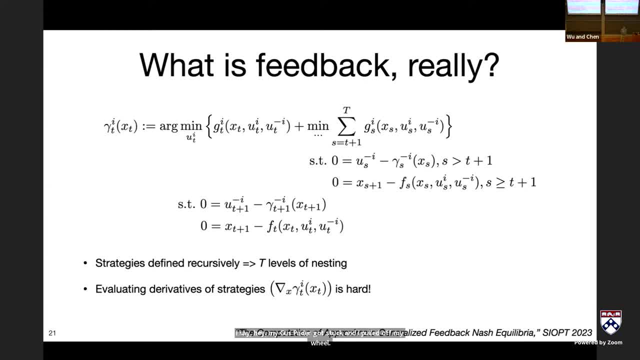 Yeah, Okay, And I communicate that. I say, oh, like, stay away from my way and otherwise we will crash. So the best response to that such of open loop strategy, as far as I can see, is just stay away from the way. 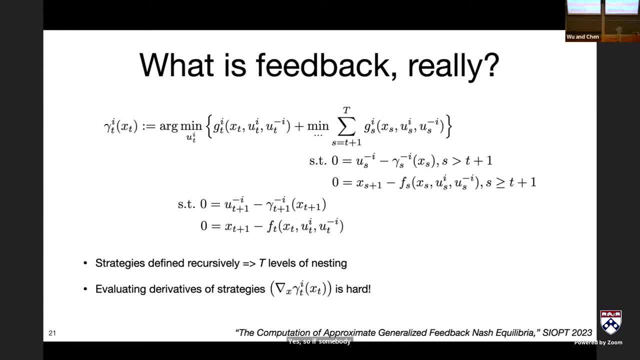 Yes, So if somebody declares an open loop strategy, then there's no reason. I mean assuming the problem is deterministic- then there's no reason you would need feedback. So you're totally right. But the equilibrium you would find would not be a feedback equilibrium anymore. 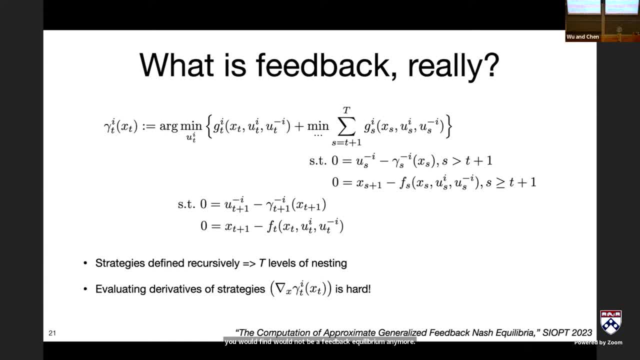 So I think all you're kind of getting at is like: well, what if? what if the game is actually just not a feedback game? But I can assume that if it's two player games, you're right, But if there are multiple players then it could be still some of them needs to. 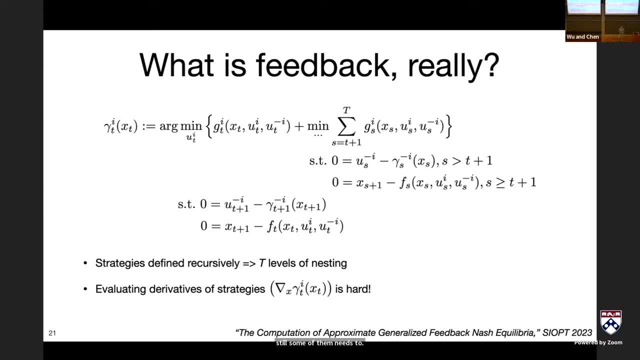 Play open loop strategies. So it is possible that an open loop strategy Actually hold on? Yeah, Excuse me, So it is. I think it's possible for some of them to play open loop strategies and some of them play feedback strategies. Let me not say something wrong. 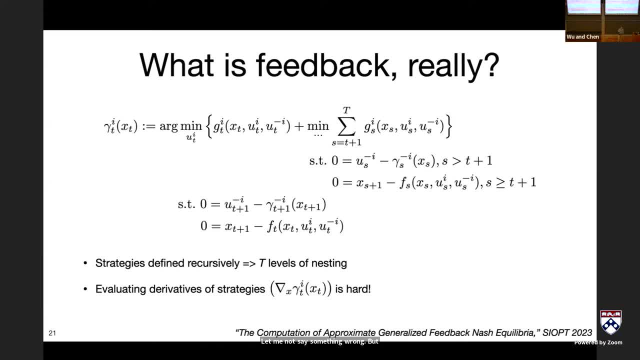 But the concern I would have is whether an open loop Description of a strategy- Sorry, Okay, There's a. let me back up for a second. There's a concept which goes by the name of a representation, So you can have two strategies which, when evaluated along a particular state trajectory. 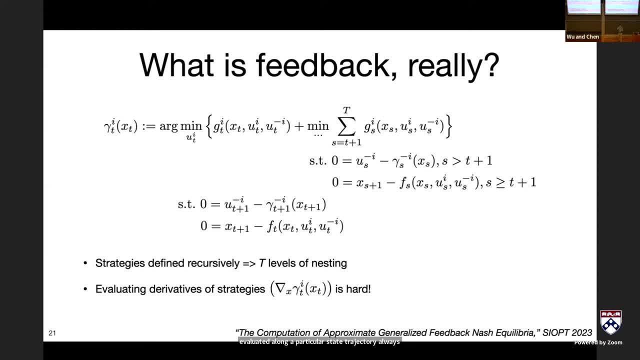 always give you the same sequence of controls, So those would be called representations of one another. So think of them like a description of an equivalent class, equivalence class. So If you knew the equilibrium trajectory of the game, You could certainly construct an open loop strategy which recovers a player's actions. 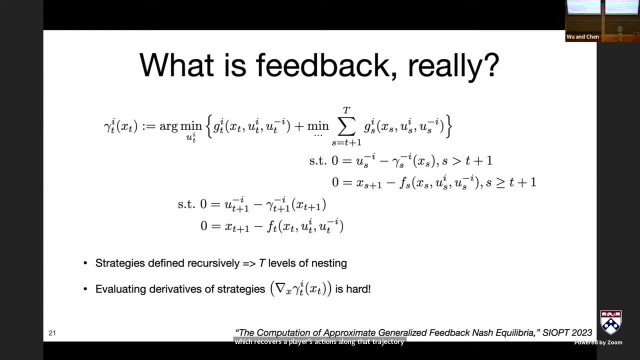 along that trajectory. But that representation of the trajectory, my sense is it would not satisfy strong time consistency. So that would be my immediate concern. But don't quote me. Okay, Yeah, Okay, We'll go with one from Zoom. Edward asks: 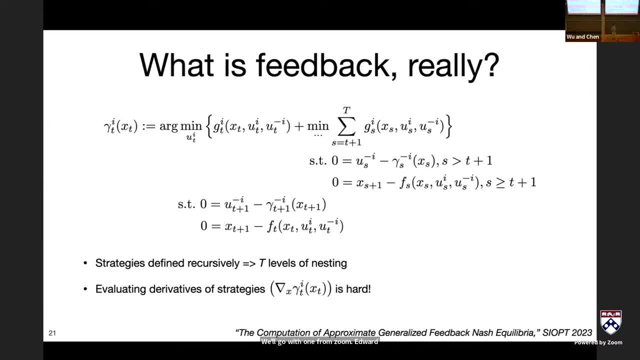 Can the insights here be used to analyze single agent scenarios? So, for example, in model based RL, could you view the joint optimization of learned dynamics in the policy as a game? What was the first part of the question? Can the insights here be used to analyze single agent scenarios? 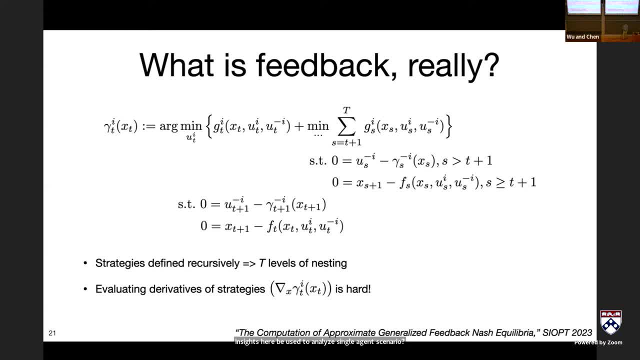 Oh, I would say yes, But. but in single agent scenarios things are a lot simpler. So in particular in single agent determinations, Deterministic scenarios, you can prove, it's actually very easy to prove- that the open loop solution, the trajectory of the open loop solution, exactly recovers the same trajectory. 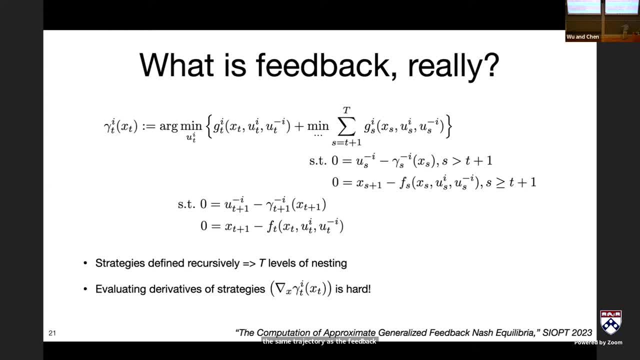 as the feedback solution. So that's why, if you think about it like an LQR problem, you can write it down, write down a Ricotti recursion and get back all the feedback controllers and then evaluate from a particular initial condition and get a trajectory. 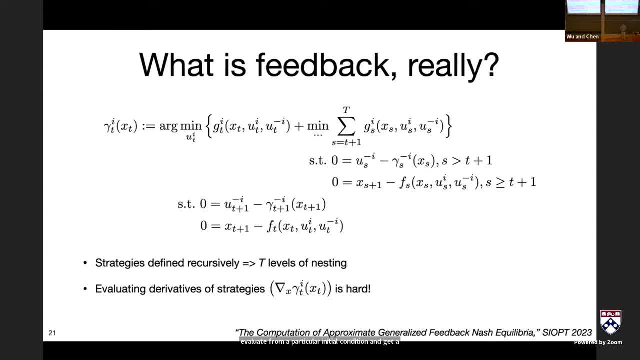 You'll get the same trajectory in the same sequence of controls, as though you just written down a question- It's a very dramatic program- and solved it So. so what I would say to this question is basically that in a single agent setting, as long as it's deterministic, you don't need to worry about all this garbage about feedback. 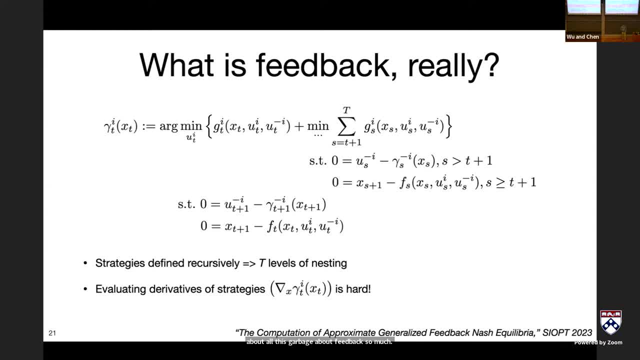 so much, as long as you're writing it down as an optimization problem like this. Now things get more subtle if there's stochastic dynamics or observation noise or things like that. Maybe that's maybe what the question is getting at. I'll ask the dual question. 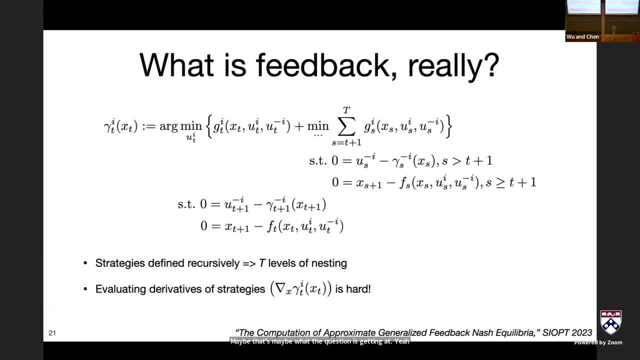 Can you give us a sense, David, of how things scale with respect to horizon and number of agents? Yeah, yeah, So good question. I guess I don't actually have this written down as like: what would a Newton step look like? 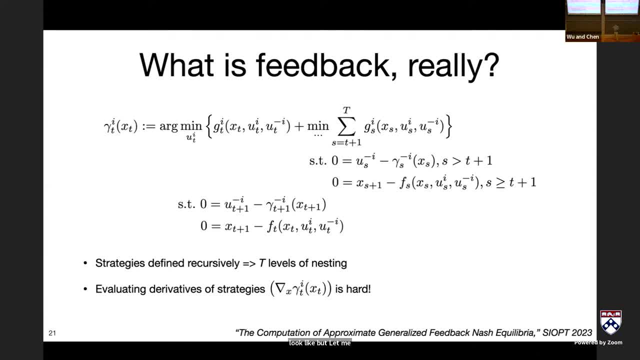 But let me not bother winding back the slides. But basically what you would do is you would write down the data. What you would do is you'd write down the KKT conditions of this problem And then, if you're taking Newton steps on those equations, the complexity would essentially 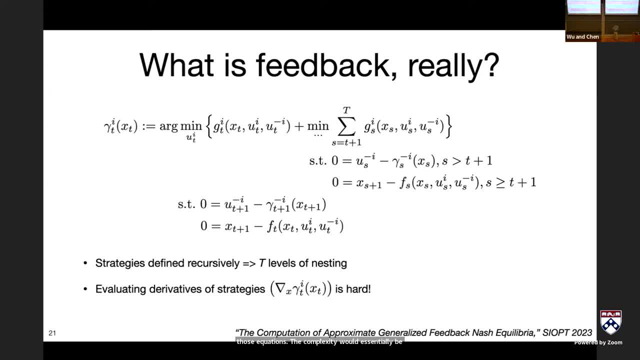 be determined by how hard is it to solve for a Newton direction. So basically you need to solve a linear system of equations to get the direction that you're going to step all the variables. That's what determines the complexity And basically that complexity is the same as you'd get in any optimal control problem. 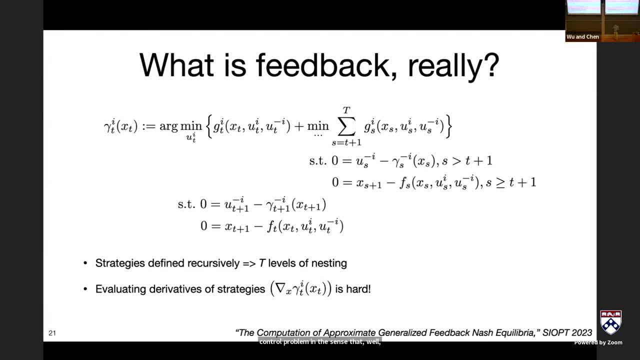 in the sense that, well, in the worst case, it's cubic in the size of the matrices involved. So what's the size of the KKT system? It's the number of variables on each, more or less, And so that's basically going to be like, so that the size would be linear in the number. 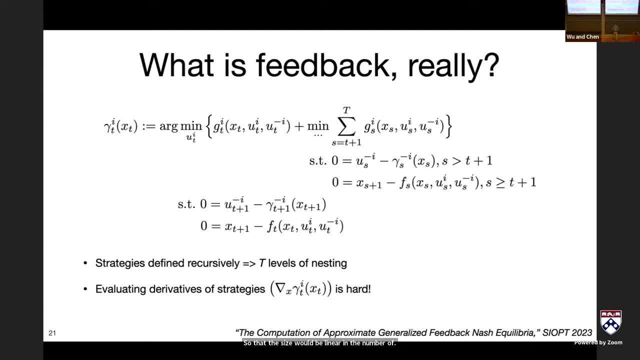 of players, because the number of controls and the number of states would be linear there and then cubic in that. But there's so anyway. It's still polynomial, But there's sparsity, which is nice. So when you write down the Jacobian of the KKT conditions of those things, it actually 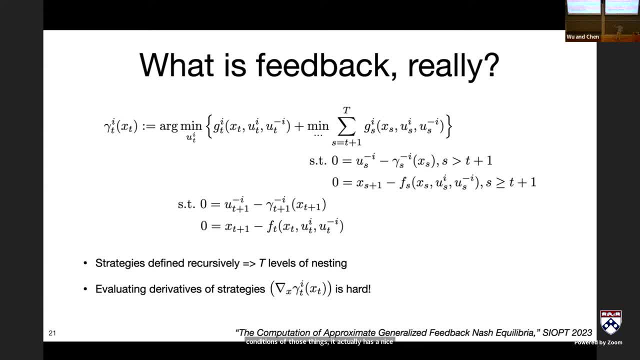 has a nice banded structure, And so you can exploit that. So it's actually not quite as bad as cubic. There's one other thing I was going to say that I forgot. But yeah, But the point is it's polynomial. 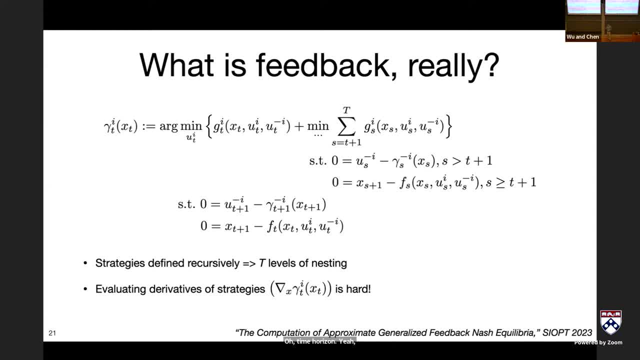 Oh, time horizon? Yeah, So just like a Riccati recursion. Yeah, So you can basically have this clever matrix factorization that makes everything linear in the time horizon. Yeah, There's a second part of Edward's question from Zoom. 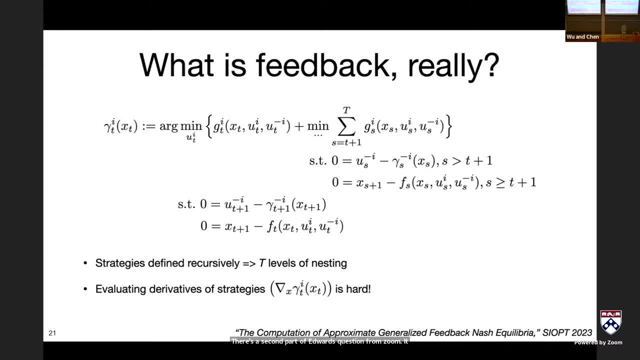 It says on open loop versus closed loop strategies. we find that open loop deep neural policies tend to generalize better than closed loop policies. By ignoring the inputs, they naively ignore all distribution Shift errors. What are your thoughts on addressing generalization or bringing insights into deep neural network? 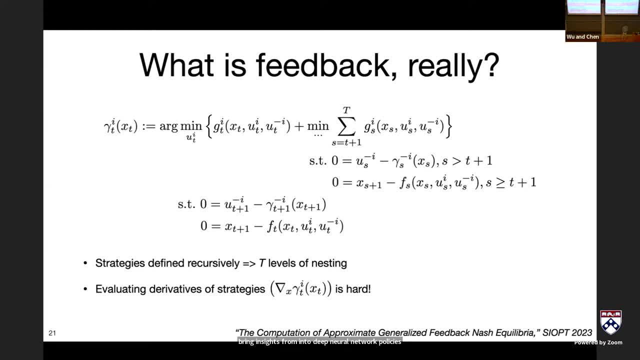 policies, Wait. So the premise here is that a deep network that's mapping from the initial condition to an open loop sequence of actions is going to generalize better than something which is mapping from the state at any given time to an action at that time. 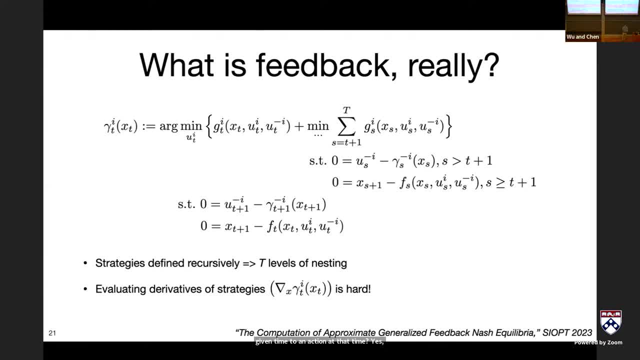 Yes, It's going to generalize in the sense of if I change the dynamics a little bit, or something like this: Yes, I believe so. Okay, I guess I'm not. This is a surprise to me, So I guess I don't have any particularly intelligent thoughts about it, but I guess I would just 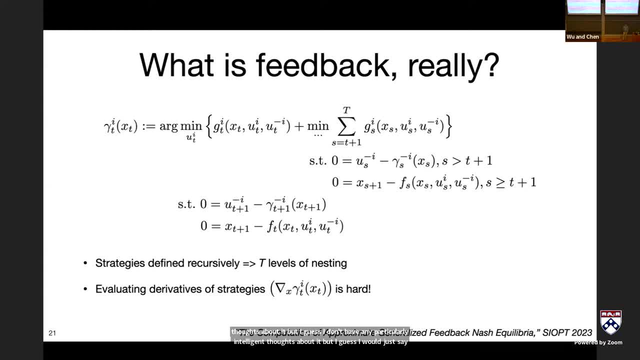 say I'm surprised. Yeah, Thank you. Yeah, But I'd love to learn more about it, if there's a reference or something. One question for me: Are the GTs assumed to be strongly convex in the use? What if, for example, the arguments have multiple solutions? 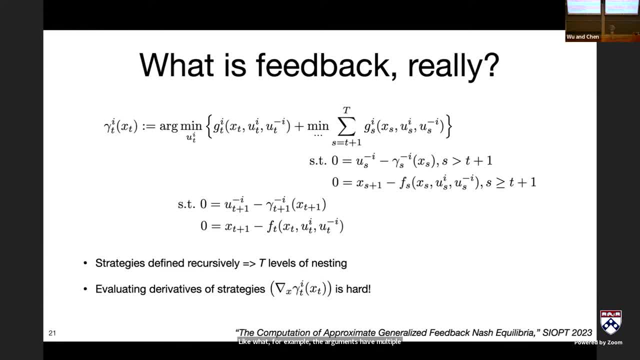 Oh yeah, I'm glad you asked. There's a. As you can imagine, there's a lot of caveats. I skipped a lot of details. For example, I never even told you what this thing would exactly converge to. So yeah, 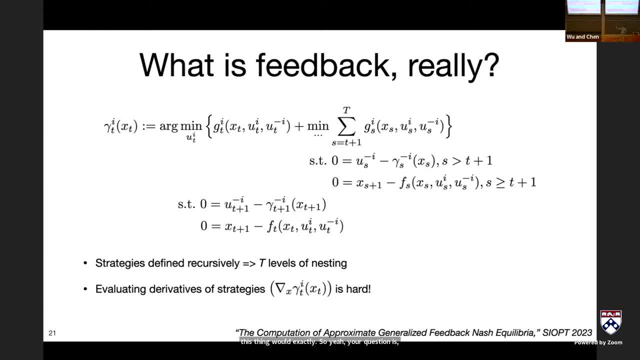 Your question is: what if this argument is generally a set and I've naively written as though it's a singleton? So yeah, So in practice, you totally don't need to require everything to be strongly convex And what'll happen is, as you're solving these. 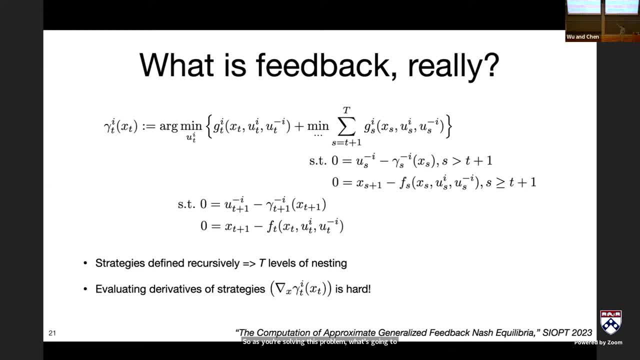 So, as you're solving this problem, what's going to happen is that if something is not strongly convex, you'll end up finding Newton will find you a solution, whatever regularized version of Newton you choose, And we've just been rolling with that. 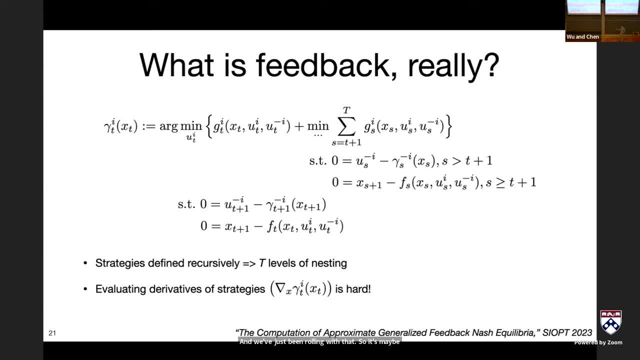 So it's maybe not a particularly Compelling fully fledged answer, but I would say, numerically speaking, it's not a problem. Yeah, I guess I could also ask one If you're in a setting where There's a collection of 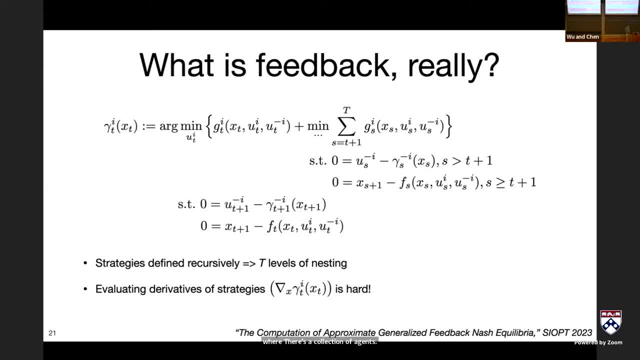 Yeah, There's a collection of agents following some optimal policy and then you introduce some new agent. Could it simultaneously learn the objectives of the existing group and then play some optimal policy itself? Yeah, So I guess there's maybe both active and passive versions of that question. 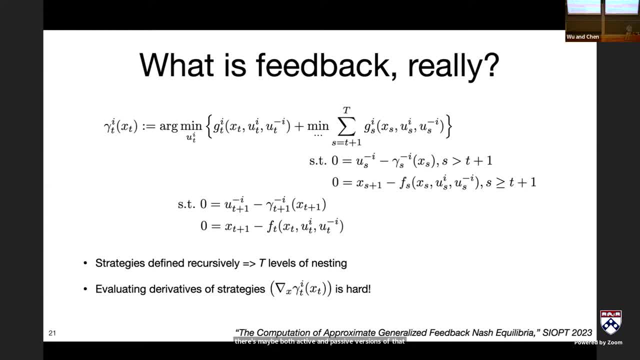 Can somebody actively suss out what is this other guy- new player- trying to do and then react? That's a much harder question, But I think I've not seen any particularly compelling good answers to- although it's interesting. What we have done is address the passive version of that, which is to say, let's say that I've 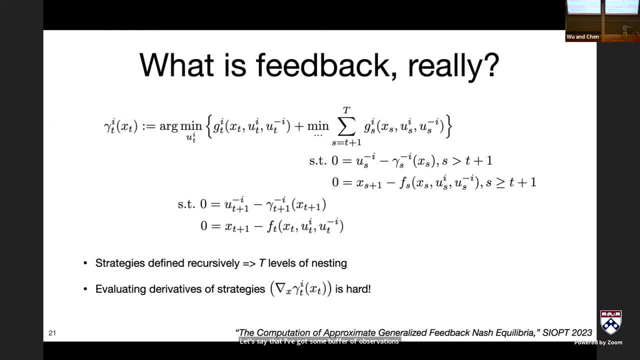 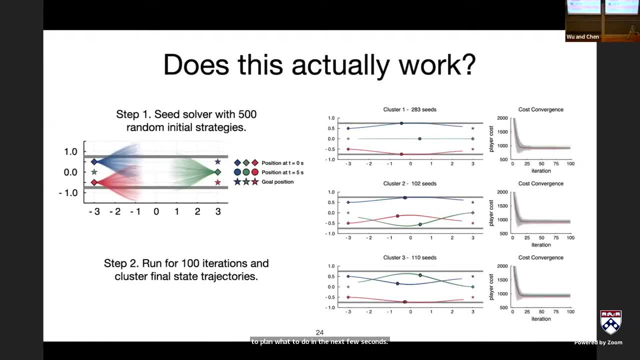 got some buffer of observations I've taken in the last few seconds and I'm also trying to plan what to do in the next few seconds. What you can do is write down a version Excuse me, A version of Excuse me. 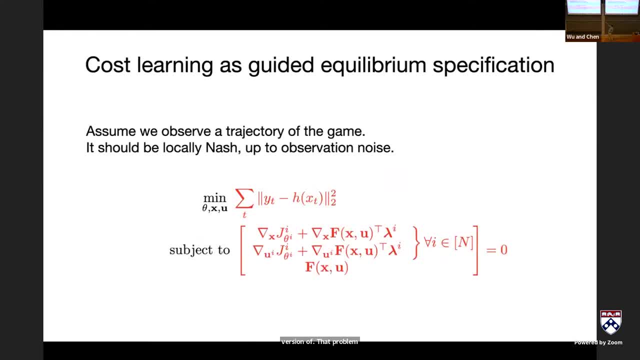 A version of a problem where here, what I'm saying is just imagine that sum over time to be like time from beginning of my observation buffer to the present, But imagine that the constraints are dealing with states and controls from the beginning of the buffer through the present into the future. 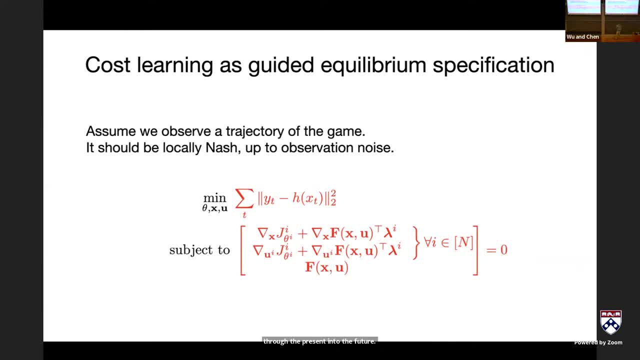 So if you do that, what you're saying is that I'm trying to be faithful to the observations I've received in the past, which include something about this other new player, And the constraints are saying every player was acting strategically in the past, but 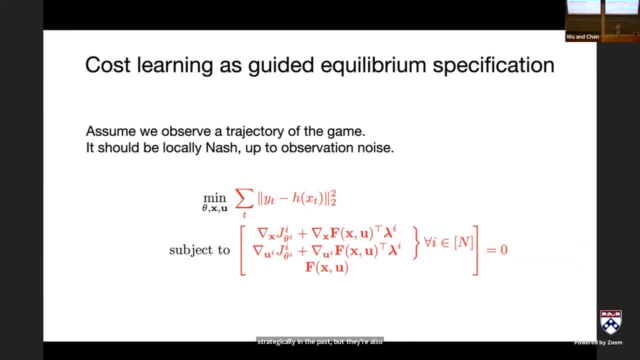 they're also saying they're going to continue acting strategically in the future And the theta variables that were kind of the unknown parameters of their objectives, including the new player, those influence both the past and the future. So you can kind of predict- I mean literally in the NPC, kind of sense you can predict. 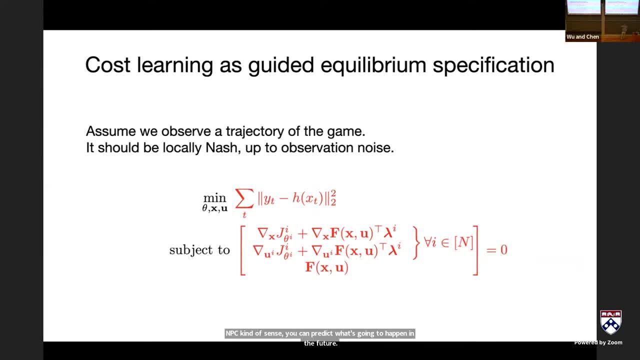 what's going to happen in the future? Um, You can predict it automatically to your estimation of the past, so you don't have to like separate estimation and control in the same sense. Yeah, Okay, Sure, So when we are assuming each agent will reach a Nash equilibrium policy, how well. 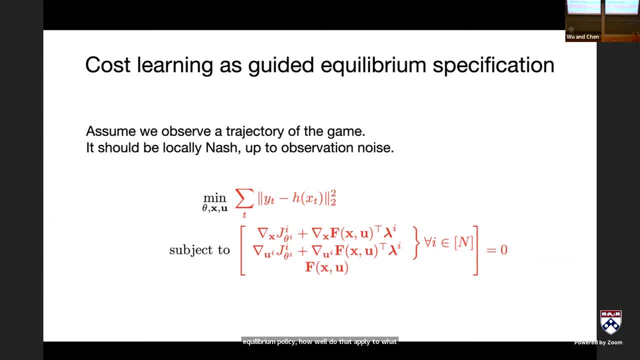 does that apply to what happens in reality, say in the future? Yeah, so the question is basically, you know, are these Nash or other equilibrium concepts really accurate descriptions of how people behave? And, yeah, unsurprisingly, like a lot of people have asked this question over decades. 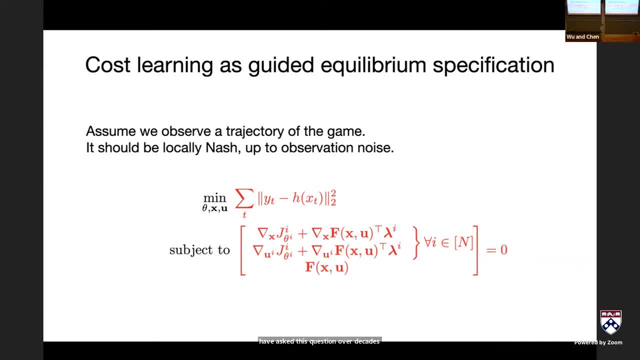 And so the short answer is yeah, there are different equilibrium concepts that do try to account for, like bounded rationality or yeah kind of other issues here. So just one that comes to mind is: there's some nice work coming. 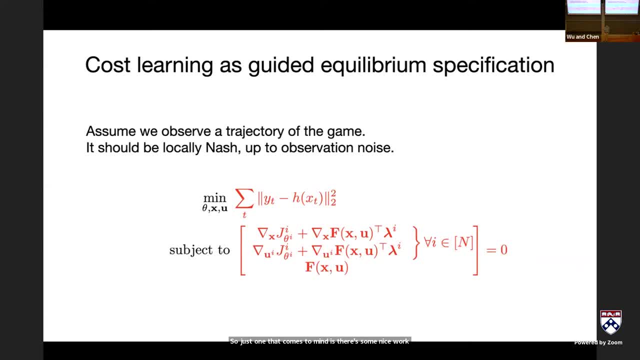 It came out three years ago. maybe that was addressing like a bounded rationality, equilibrium concept. So what you can do, What you can do there is you can say: take the original Nash problem and then also imagine that every player gets to select a stochastic strategy and give players a bonus for acting. 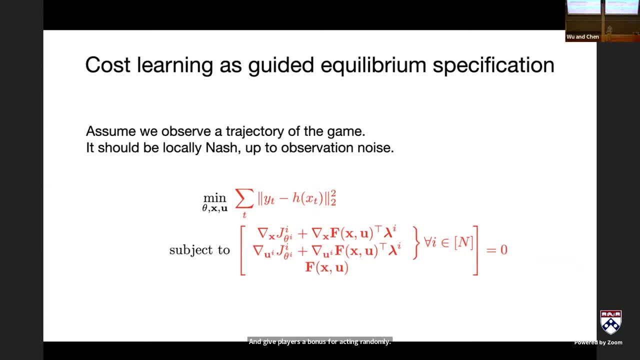 randomly. So some measure like the entropy of their strategy or something like this That you know, subject to whatever distributional assumptions you put on it, that thing can have a very nice clean equilibrium condition, Yeah, And you can solve it kind of with similar Riccati recursions. 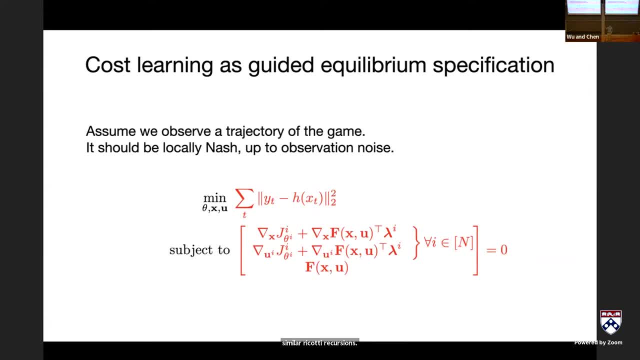 So I mean with again a lot of caveats, But that's a paper I remember that was kind of trying to address that issue. My own take would be to answer: To really do justice to that question requires probably more data and more experimental ability. 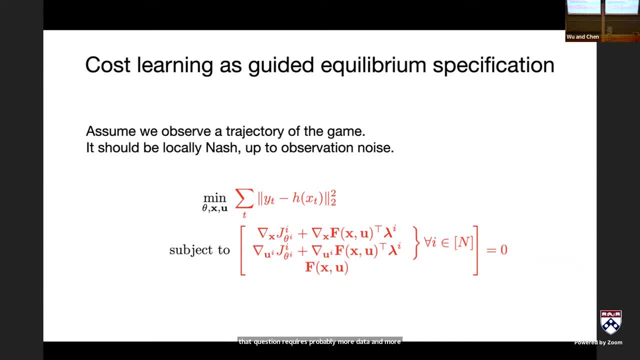 than you know I or probably most other academics would have. So there's data sets out there for you know, recording like Waymo computers. Yeah, So you know like you can put like a bunch of real cars in different intersections or 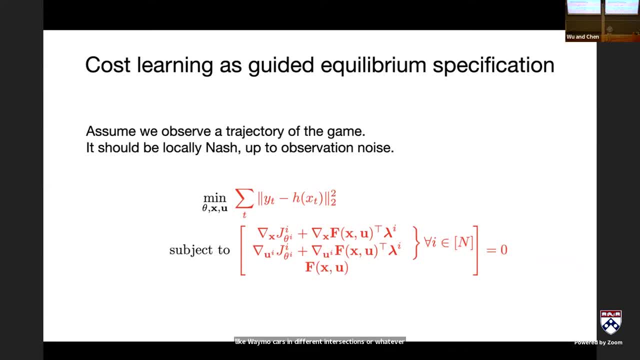 whatever. But the trouble is that those are pre-recorded. They're not like. Like I can't go in there and say, well, what if I had done this other, different thing than what the car actually did in the data set? 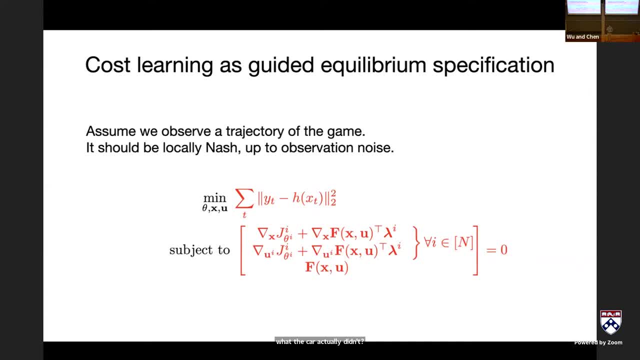 So I don't have the counterfactual And I don't know of any data set that could possibly have that information. So people try to train- you know neural network models- to predict other players' actions, And then it's kind of a chicken and the egg problem. 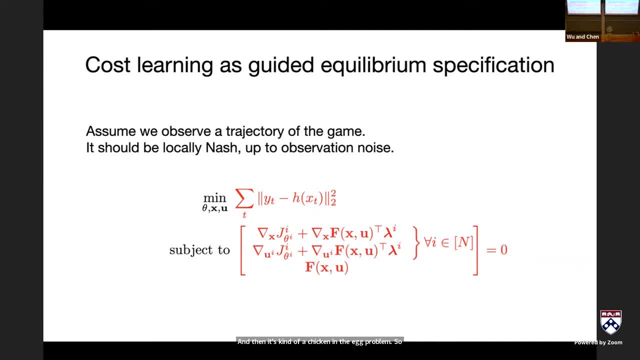 So I've kind of been, I've been very unconvinced by like generally the outlook in that space. So anyway, long story short, I've like thought hard about that problem and come to the temporary conclusion that I don't want to think about it anymore. 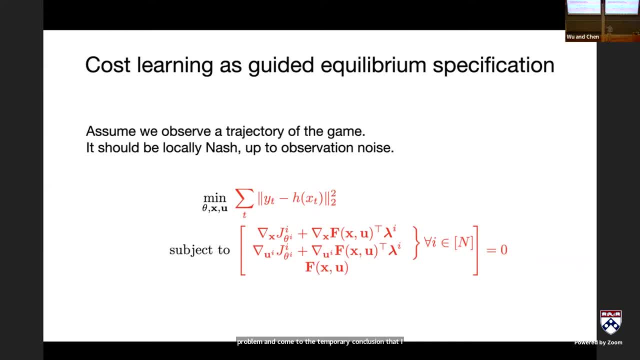 And I just want to trust the decades of, you know, people in economics and other game theorists that have concluded that this is a decent enough model. Yeah, Yeah, Yeah, Yeah, That's pretty good. Thanks for sharing that, Yeah. 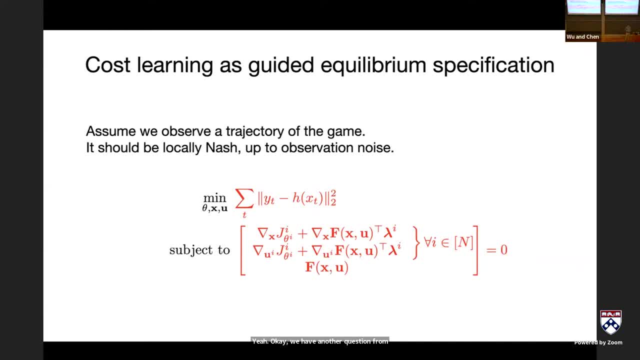 Thanks, Thanks for having me. Yeah, Yeah, We have another question from Zoom, from Austin, that says: how stable are the computed policies when other agents play nonoptimal policies? How stable are the computed policies when players deviate from equilibria? 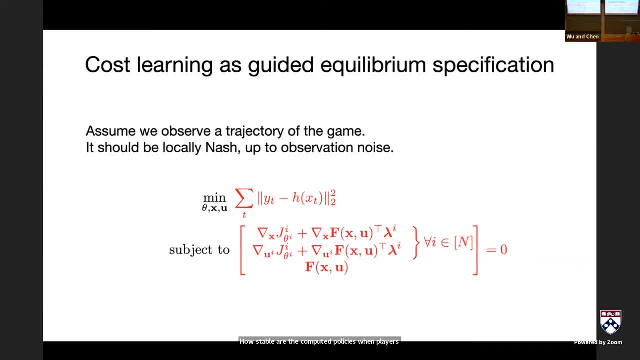 So yeah, so this is a great question. I guess the real answer to this question is: they're very stable. if this is a zero-sum problem, If this is not a zero-sum problem, then they can be Right exploitable. So yeah, that's the answer. Yeah, Oh, let me actually say one more thing on 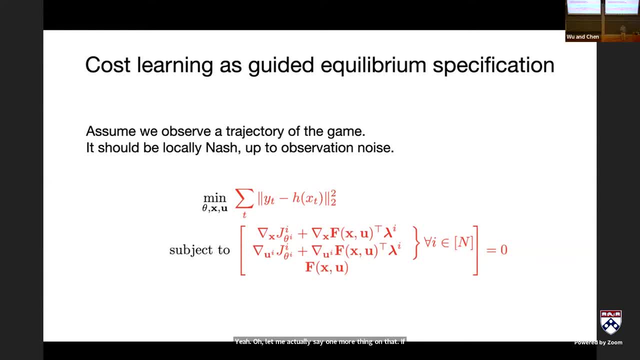 that If it is a zero-sum problem, it's probably not too hard to imagine that if player one has a nice beautiful convex objective with respect to its variable, I mean, depending on the situation, it's probably not hard to imagine that player two's objective becomes. 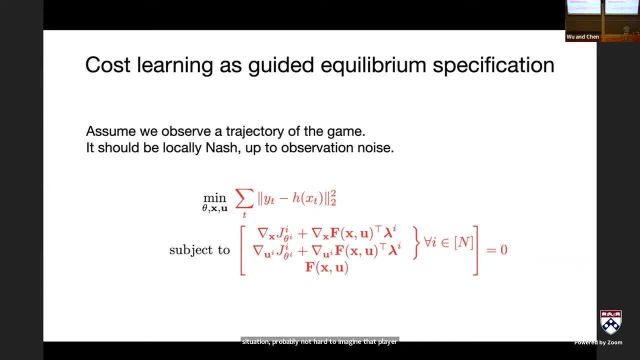 concave. if they're wanting opposite, things Depends, But that can cause numerical problems. So I would say, like the methods I've shown you are not like they're looking for first-order stationary points And so they can be susceptible to kind of curvature issues that really arise. 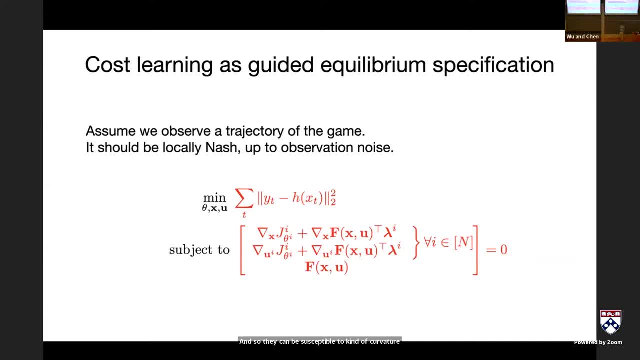 in zero-sum problems. Yeah, Thank you, David. This was typical, David. Yeah, Thank you. Very, very substantive but limited. Okay, Well, thank you very much. Yeah, Yeah, I try not to over-claim anything. No, I cannot ask any reasonable question. 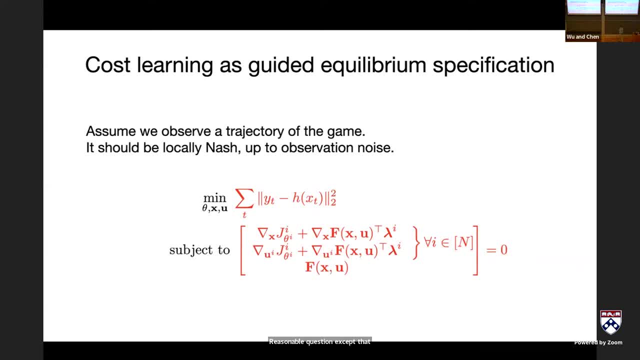 except that saying what are the limits? Oh, there are so many limits, So many limits, Like where to start. The first place I would start is like everything I told you about is a local solution. So you know, I would. 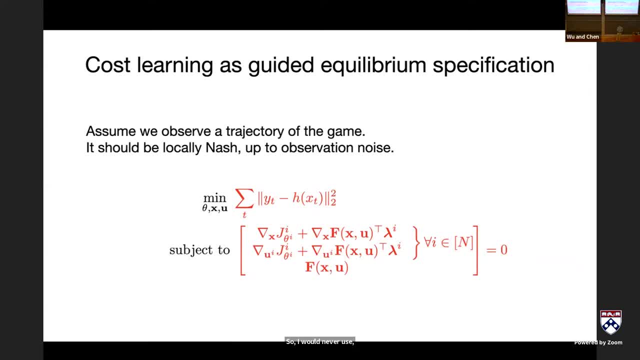 never use, like, even if we could solve zero-sum problems perfectly, which I just described, have issues? Well, even if we could do that, we're only finding a local solution. So I would never, you know, just go and tell you, hey, this solution is not going to solve zero-sum. 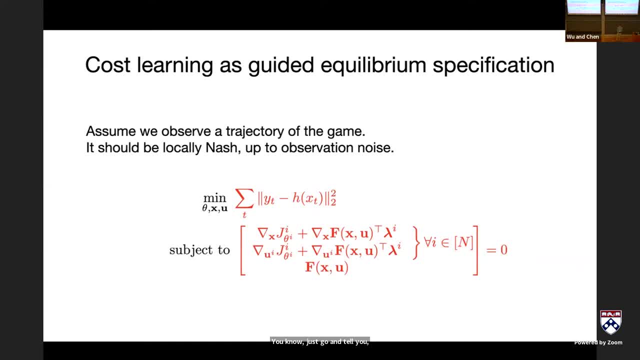 problems perfectly And you know the solution is robust to arbitrary perturbations of the problem because, like I, would never go and use this for a safety-critical situation. So you have a live art form: Yeah, Where it's much more complex systems, Yeah, Yeah. 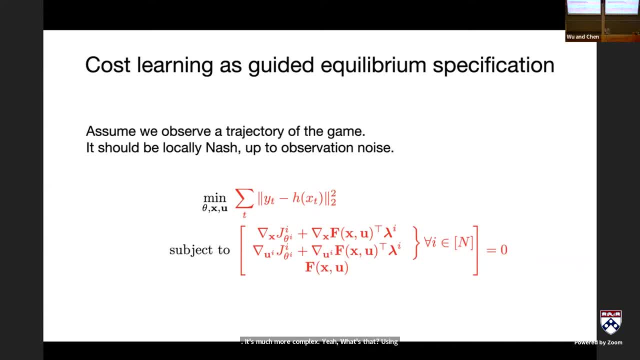 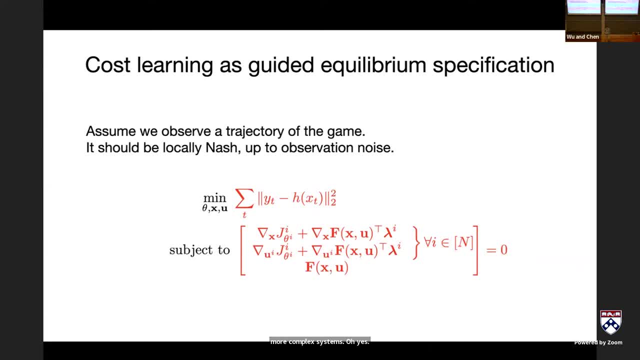 oh yes, situations using the same methodology? yes, so, for example, i mean uh, like one of my students just now is working on uh algorithms which are not so susceptible to the numerical problems i mentioned in zero sum cases. um, just as an example. all right, thank you very much for all of you. 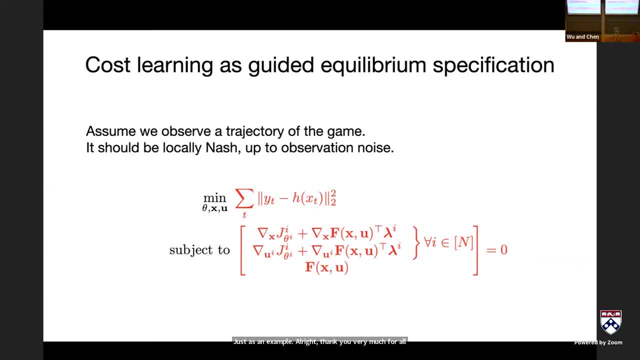 coming. yeah, thank you.